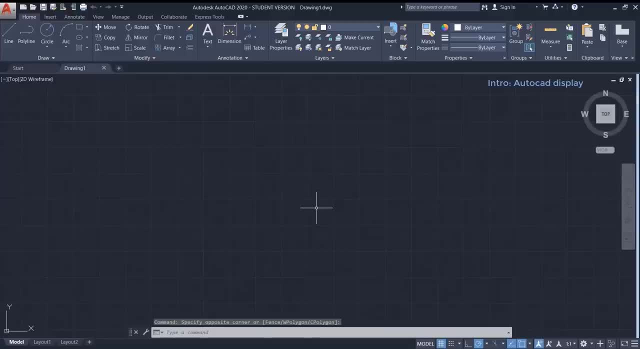 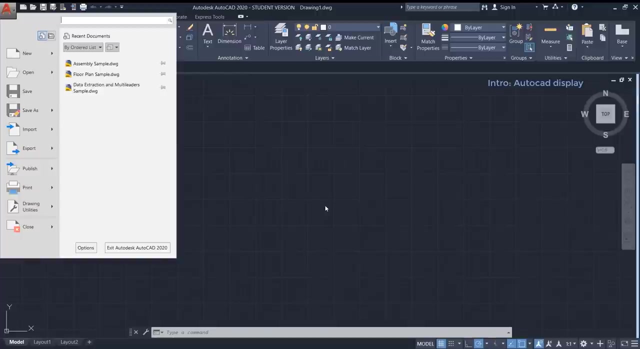 Okay, this is the AutoCAD default display, which consists in different areas. Above at the left, you find the application icon. This is the menu where I can open a new document, open a file or do operations regarding saving or exporting a file. Then 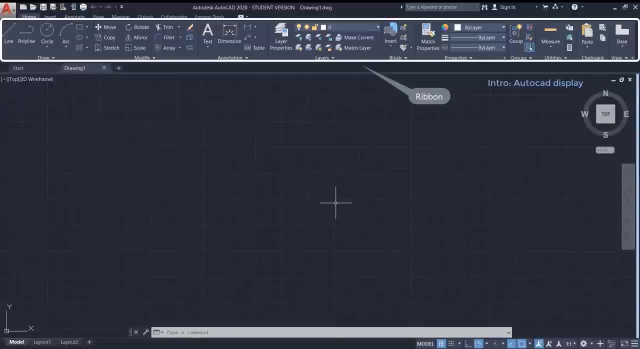 the main part at the top is called the ribbon. There you find the majority of tools you will need during the program. Right above you can find these tabs which group the buttons in different categories. For example, the current one is the home tab which has the most used icons. 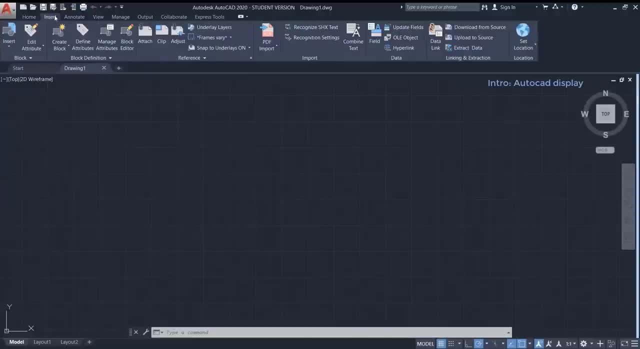 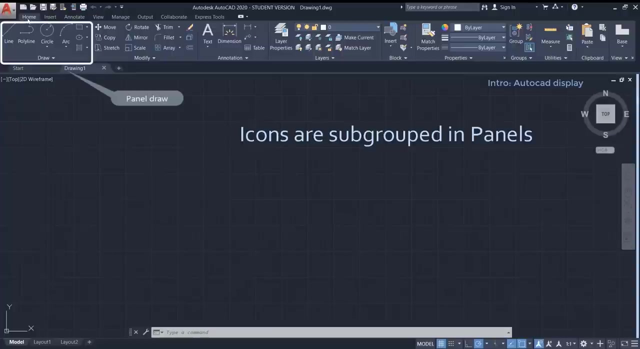 If you switch to the insert tab, I find in this case icons related to this category. Then, inside the specific tab, the icons are subgrouped in panels. For example, in the home tab, the first panel have the icons which can perform drawing actions. In the second panel they are related to modifying objects. 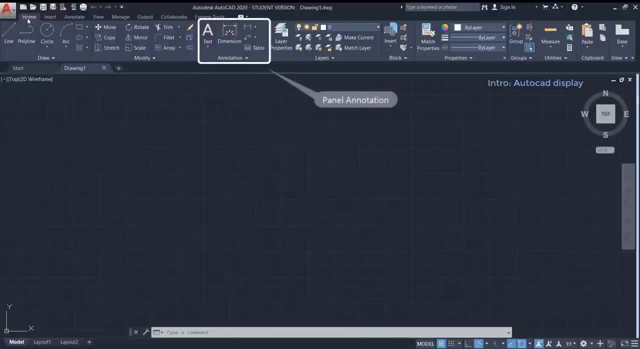 And on the third panel are the annotation icons. Additionally, when you click in a panel that has an icon, you will see the icon that has the most used icons. So if you click in a panel that has an arrow facing down, it shows extra icons which are used less often. 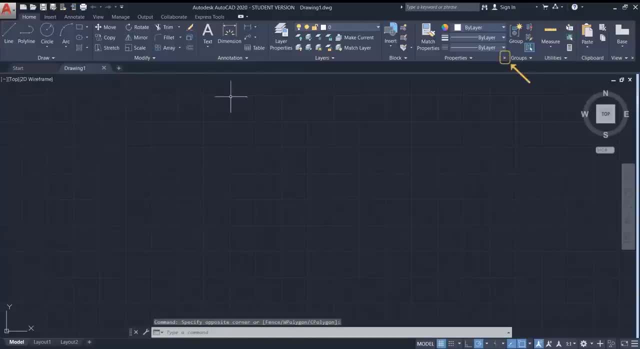 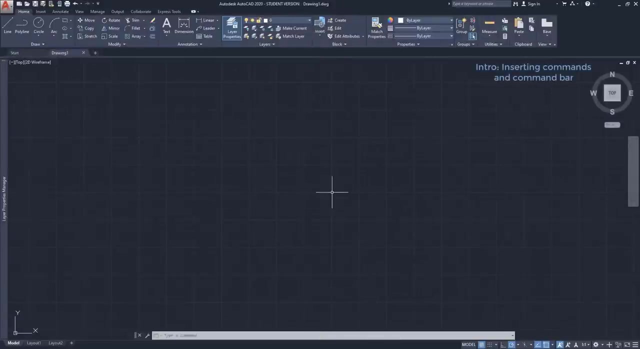 When a panel has a diagonal arrow at the right, I can access to the settings window of this category. Now let's show you how to use tools in AutoCAD, For example. imagine I want to draw a line. As you may guess, the tools are very simple to use. 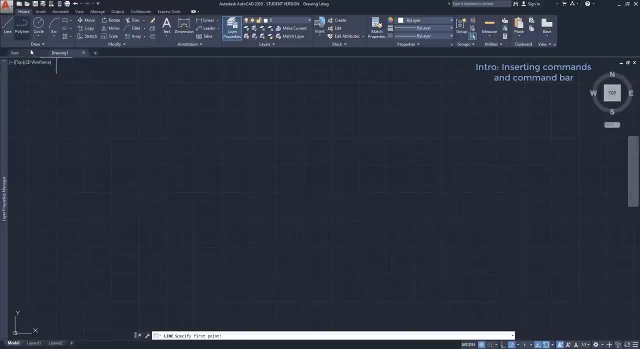 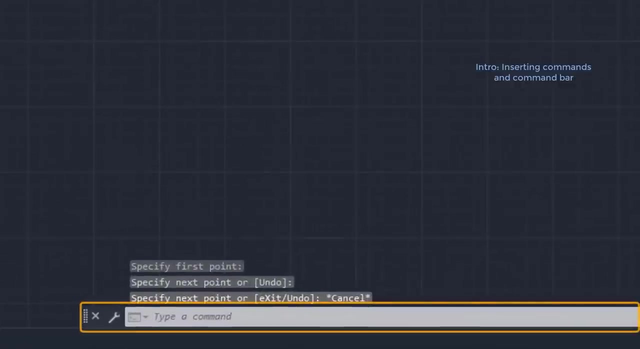 may guess. I can click in the icon here. I go to the workspace, I click for the first point and then, where I want the second point, I click again, simple. then I'm going to repeat the process, but this time I want you to pay attention to this- the command bar. this shows the operations that are taking. 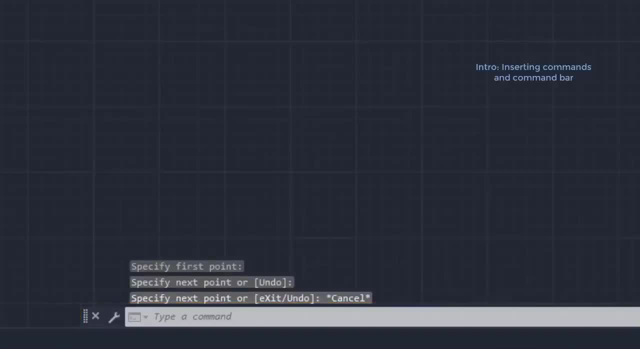 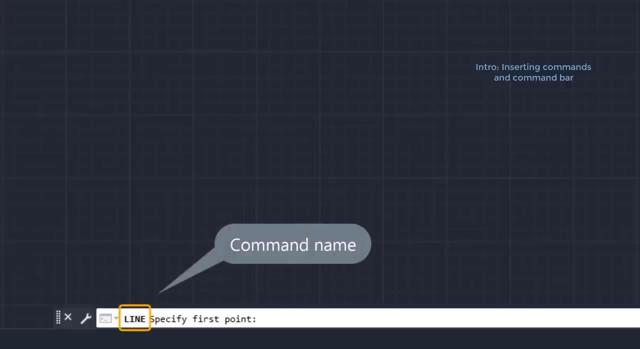 place during the project. I will show you. I click again in the line icon and you can notice here: line specify: first point: the first word which appears in capitals is the command name, in this case line. then that's the prompt sentence which tells me what I should do next. 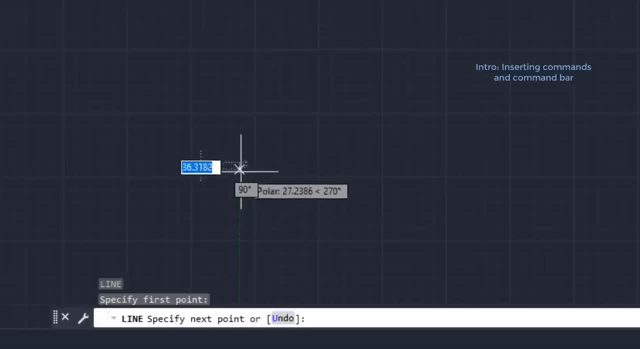 though. I click here to start specify the first point. then it asks to specify next point. click again. as you see, I just draw a line but it keeps asking for specifying another point. it would draw a new line. as I don't want, I can press escape to exit the line command. in conclusion, to perform any 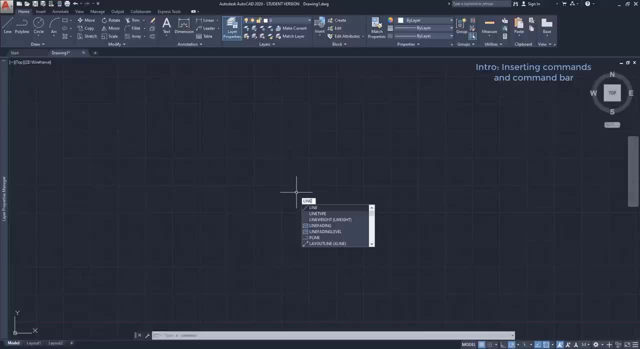 I can type its command name. for example, I type line and press enter and I can draw a line, then press the button escape to leave the command. now I want to draw a circle. I can click in its icon or type the command name, which is circle. additionally, each command has a shortcut called. 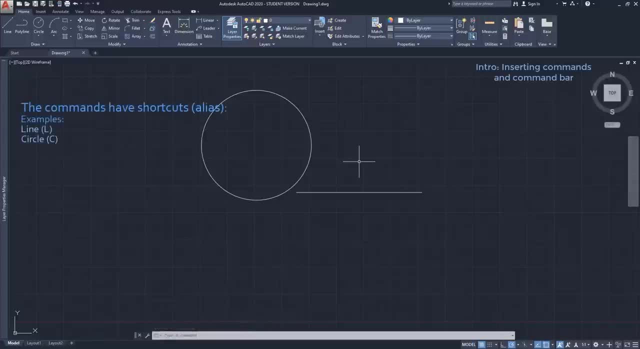 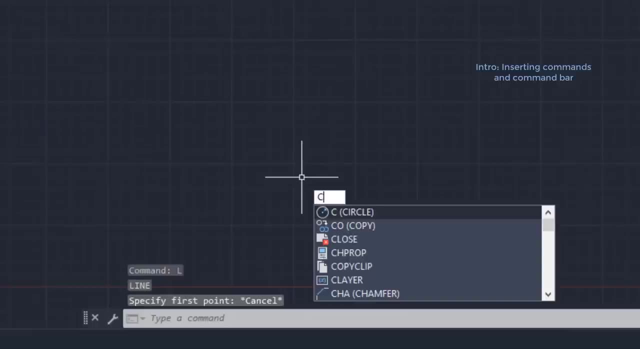 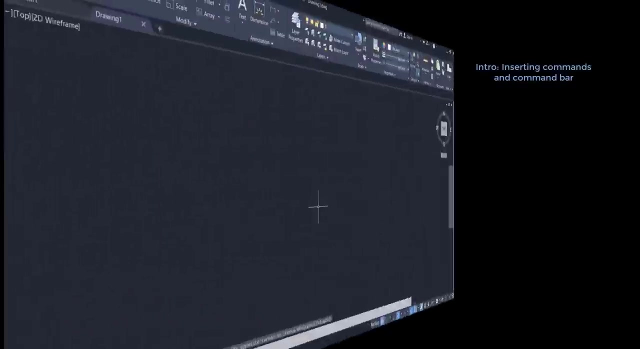 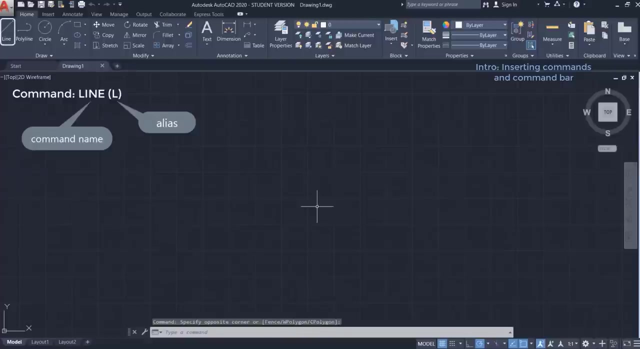 alias, so I don't need to type its full name. for example, l is the shortcut for the command line and c is a shortcut for circle. during this tutorial, each time I introduce a new command, I make an annotation at the left part of the screen showing the command name, the alias and its location on the ribbon. this way of inserting commands show. I hope you liked the video. subscribe to my channel and see other tutorials found on this tutorial. I will put all the links written in the description as achterbox and all my works in the description. I put all the links in the description. you have to dial the box for every ah as well and look at comments. 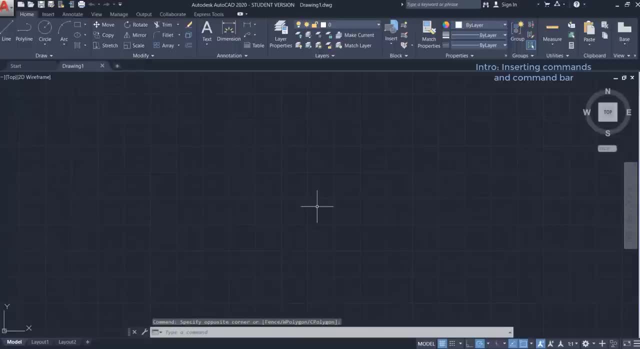 for school. just click here to find the name and againigning you can use this Alt. This way of inserting commands makes AutoCAD easy to switch from different versions. If, for any reason, I'm going to a computer that has AutoCAD 2007,, which had a different. 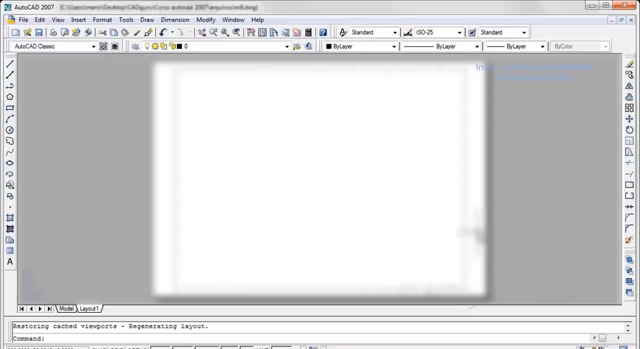 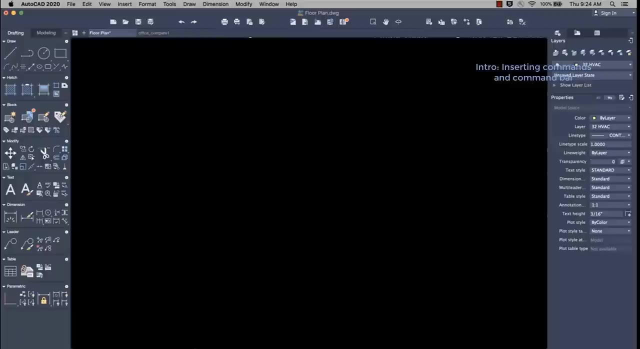 display than this one, I can still work with no problems because the command names and their shortcuts are the same. Of course, some functions were not available in that time, but almost all the basics didn't change. The same applies to the version in Mac. 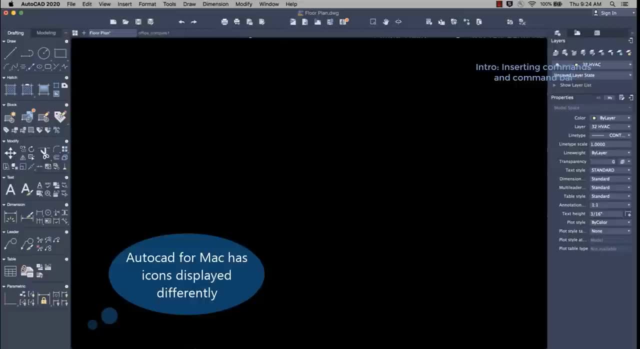 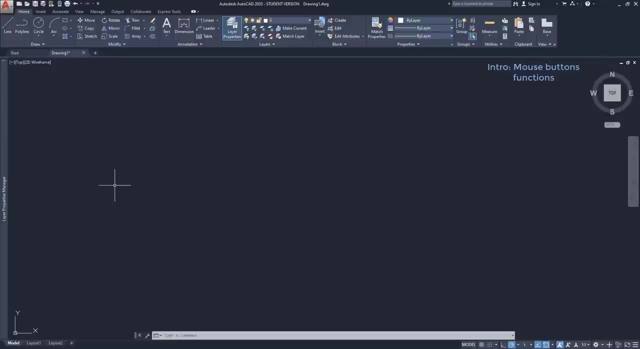 Even AutoCAD 2020 there has a different display. the icons are in different places. you can just type the command names and don't need to worry to find them out on the screen. How to use the mouse in the workspace. Having a mouse is very important for work. 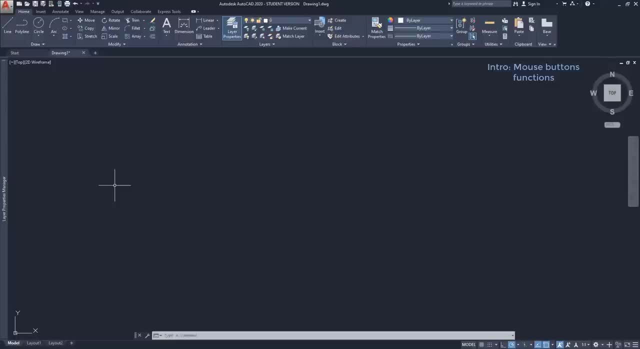 It's much more comfortable than using just a touchpad, especially for zooming or moving the workspace area. Let's see the functions of the mouse buttons Here. I attach this image to help you: Mouse wheel. With the mouse wheel I can zoom the workspace. 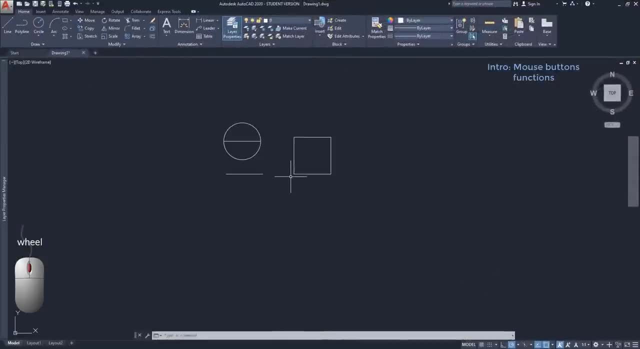 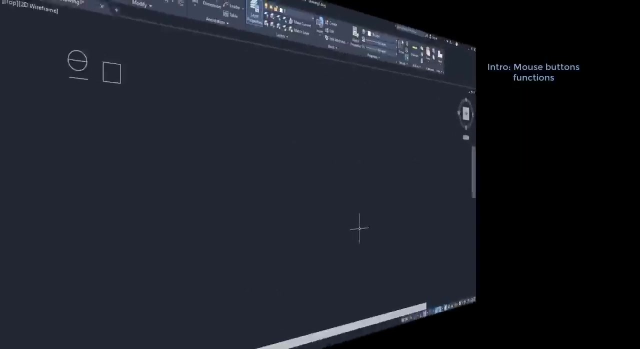 It's very simple: If I scroll up, I zoom in. If I scroll down, I zoom out. The zooming always applies to the exact location of the pointer. For example, in this situation, if you want to zoom these objects, I need to move the. 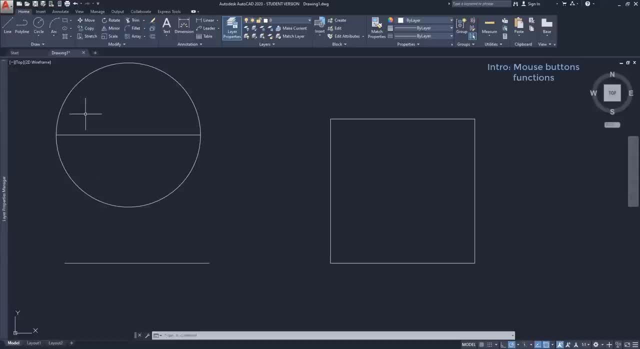 pointer over them. scroll up and you notice they are filling all the screen. Simple To move the workspace area: press and hold the wheel. When you see this hand, You can move around. Left button Clicking with the left button I can select objects like this circle: 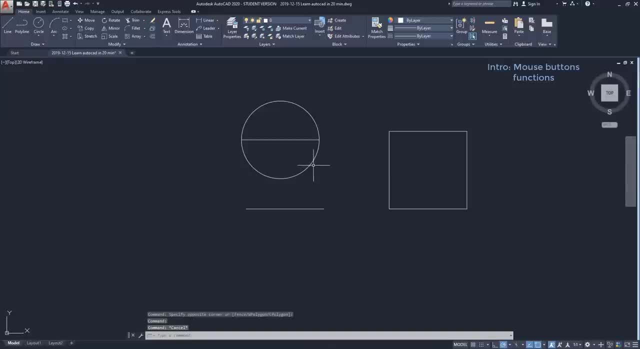 If I want to select the circle and the line, I can click first in one, then in the second without pressing the control key, unlike other programs. But now imagine you have a bunch of objects to select. Let's hide the control key. 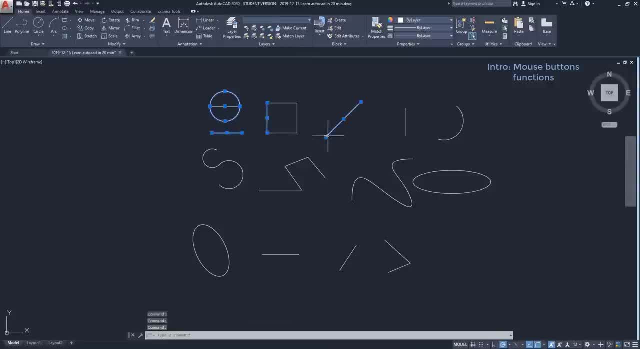 Just look could take a long time to select them all. for that reason, if I click in an empty space, a selection area opens. this allows me to select more than one object, however. this is important. there are two kinds of selection. if I open the area to, 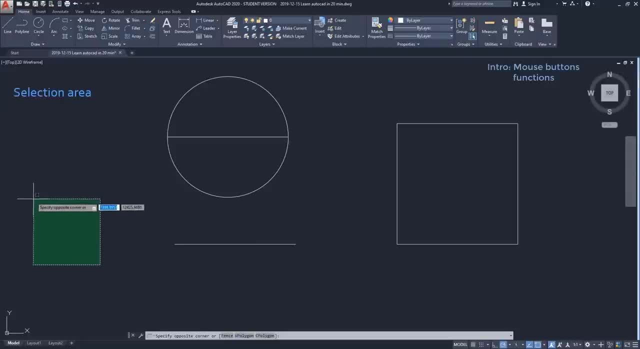 the right, the color is blue. if I open to the left, the area appears in green color. what's the difference? when I open to the right blue color, I have to cover the entire object to select it. if I would open to the left green color, it's enough. 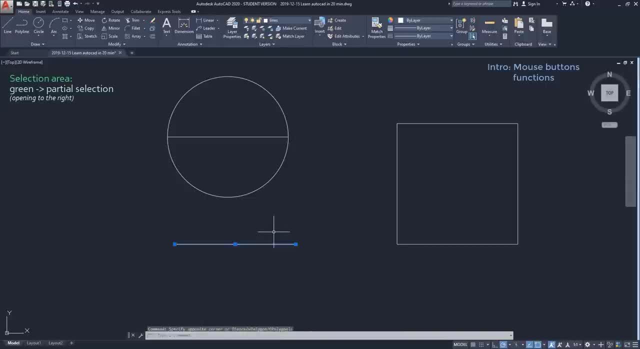 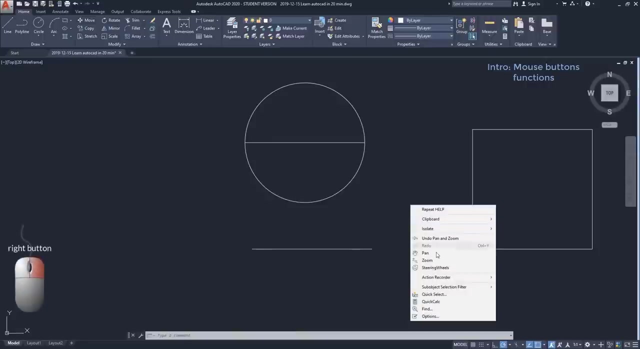 if I only cover one part. also, you can understand if the object is going to be selected. when you see it turning bold, you can select it with the right mouse button, now the right button. the right button opens this panel with several options you can choose. but when you select an object and right click, you can access. 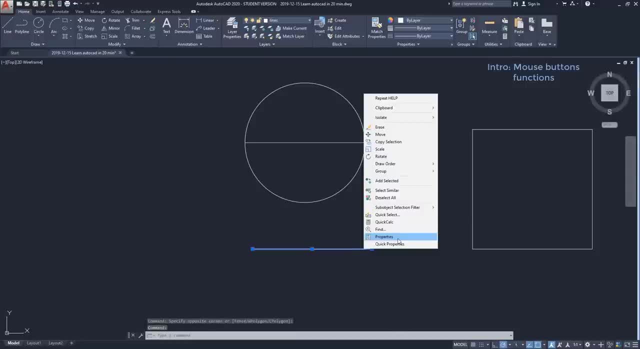 for example, to its properties, I click. it's a long list over here, I'm going to close it. however, there is a compact version of properties- quick properties- which contains the most important features for this line. you can see the object type, line, color, layer, line, type and length. by the way, in the quick 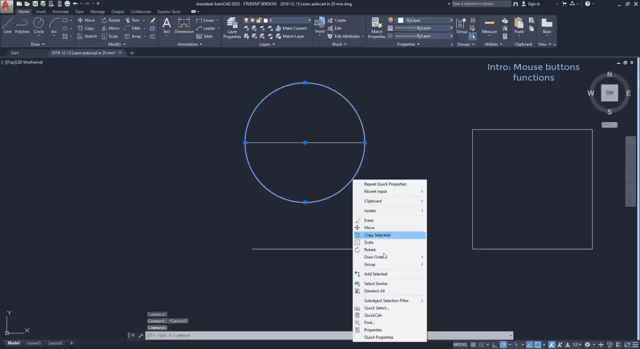 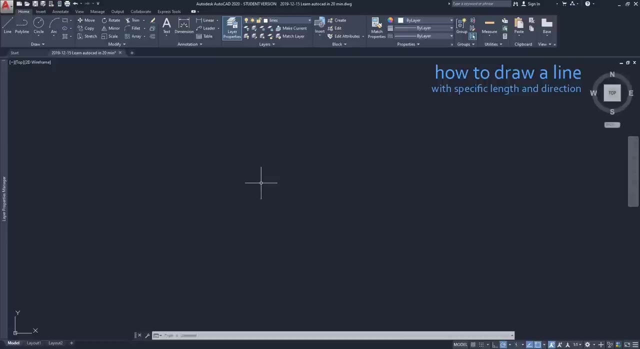 properties of this circle. some of the topics didn't pop up for the line, as they are more relevant for circles like the diameter, radius or area. in this chapter, I'm going to teach you to draw lines properly. the line is probably the most basic tool and the one you will use most of the time. before I 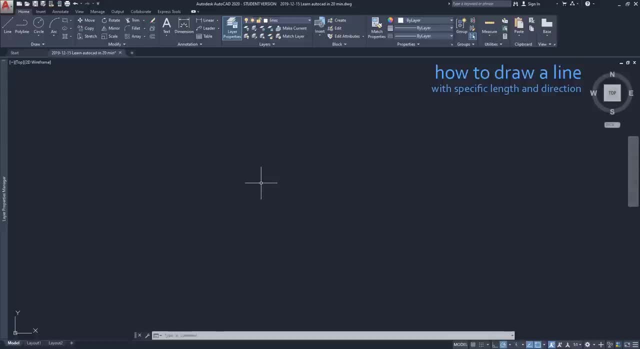 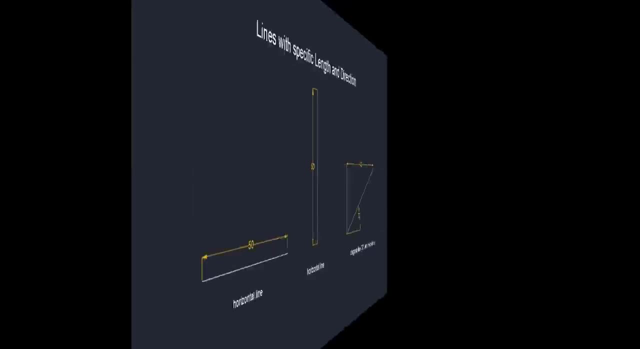 showed how to draw a line, but without any specified lengths or direction, I mean if it's horizontal, vertical or if it makes an angle with the x-axis, for example. that's exactly what you will learn the next few days, until we can draw a line with this tool. 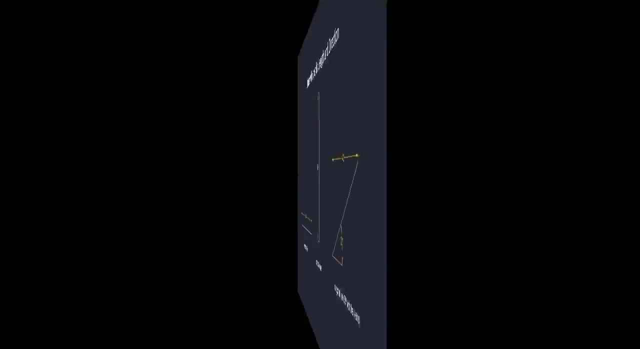 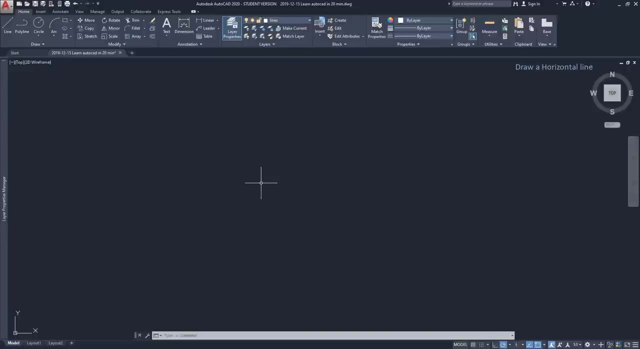 few minutes. Draw a horizontal line. To draw a horizontal line I need to activate first the command line. I can click on the icon there or type the command name as you remember from the first captor, or I can simply type l- it's the alias for line- and press enter. 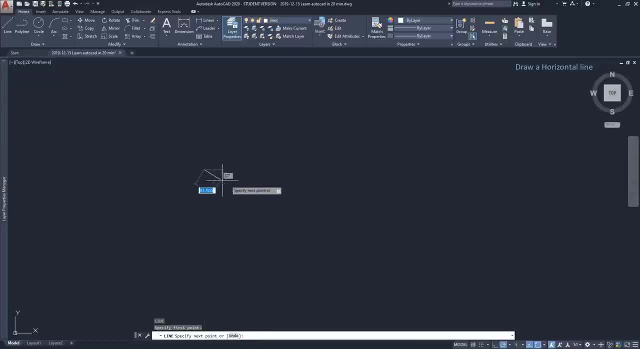 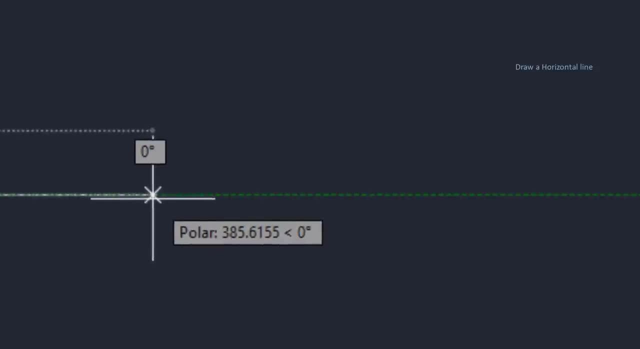 I click anywhere on the workspace for the start point, then I drag the cursor to the right and you can notice this dashed green line with this label saying polar and zero degrees. if I click right now, the line becomes completely horizontal. this happens because I have the polar tracking turned on. 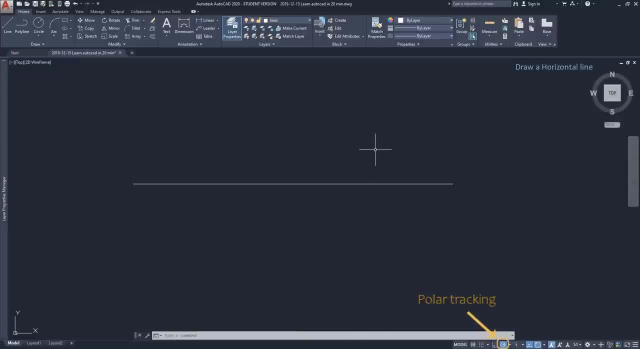 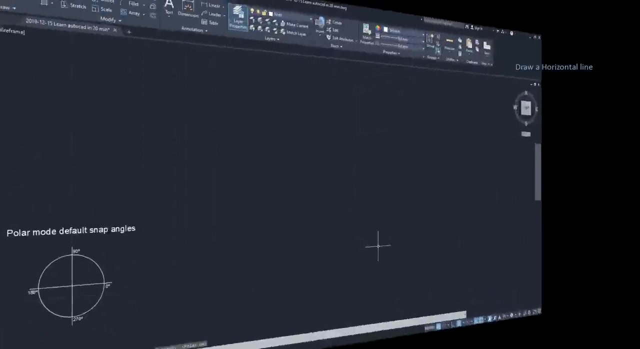 this icon located in the status bar. the polar tracking allows the cursor snapping to certain angles. by default, these angles are set for zero degrees, ninety degrees, one hundred eighty degrees and two hundred seventy degrees, making the lines vertical and horizontal. now look what would happen if the polar tracking is off. 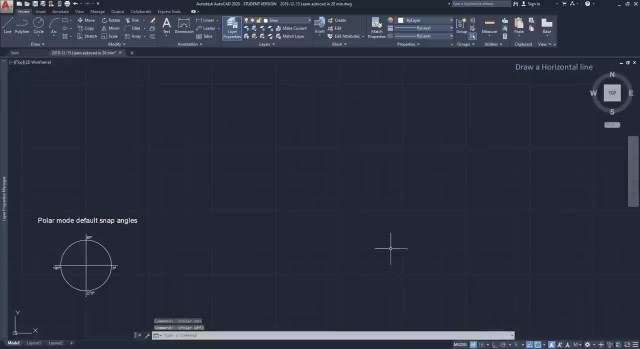 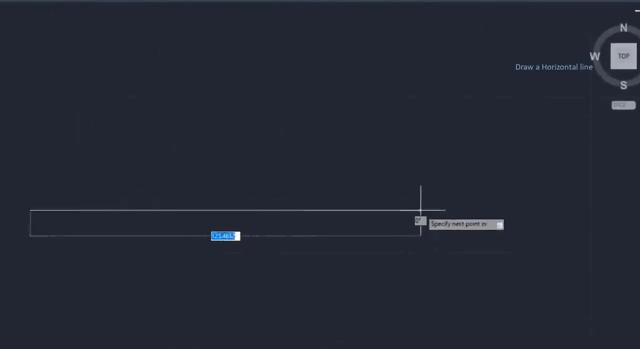 click on the icon, it's disabled now. then I'm going to draw a line again. type l, press enter, click for placing the start point. then, as I'm trying to draw a horizontal line, I realize that the dashed green line is not there. that means when I click. 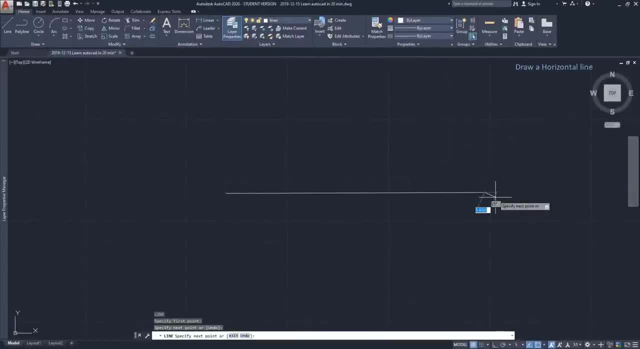 even the line looks horizontal, there will always be a slight deviation. so I strongly suggest you to use the polar tracking whenever you want to draw a line. whenever you are making precise drawings, draw a line with specific length. this time I'm going to draw again the horizontal line. 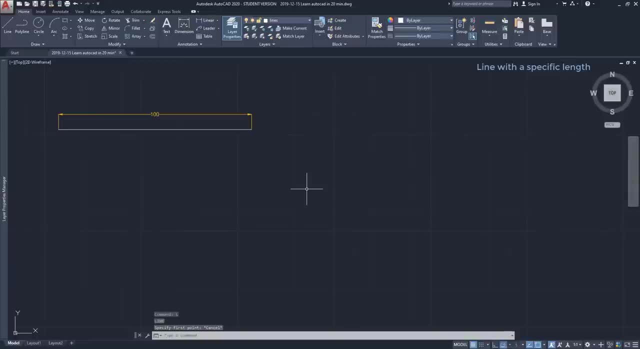 but with a precise length of one hundred. it doesn't matter the units for now. as the last command used was line, I can press enter to revert to the previous one. look, it turned on again the command. I click. I move horizontally to the right, now that the line is on the direction I desire. 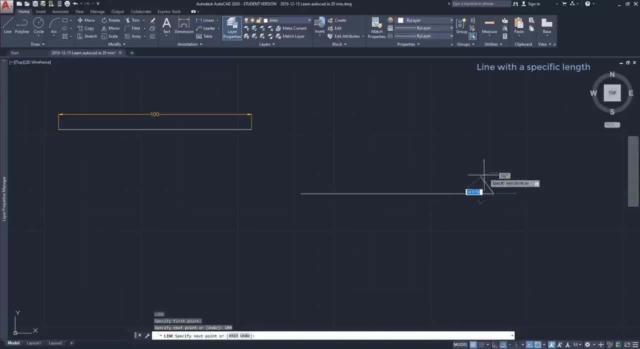 I can type one hundred and press enter, easy. you just drew a horizontal line with a length of one hundred. but be aware, when I type the length, I cannot change the direction anymore. see, I move the mouse and nothing happens. so, I move the mouse and nothing happens. 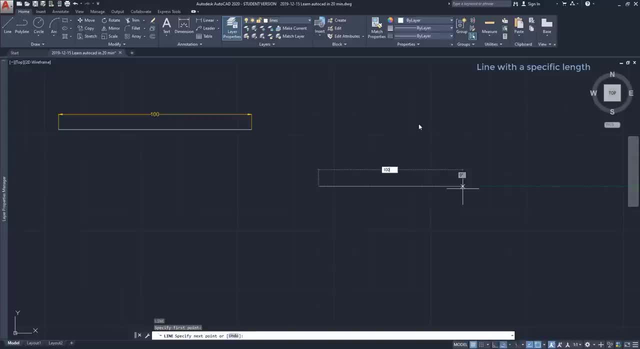 so I move the mouse and nothing happens. so if it's not on the direction you want, you can press escape. now I can make it vertical, for example, insert the length again and press enter to confirm this. I click on the line right-click. go to quick properties. 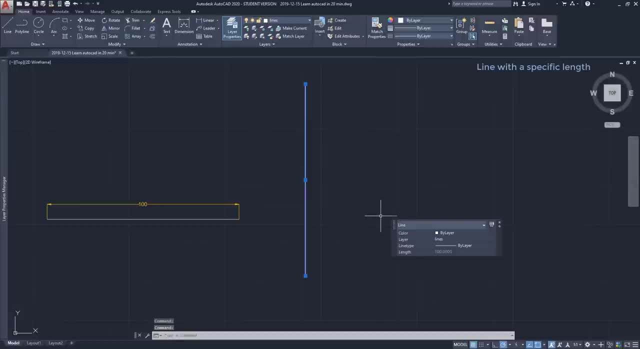 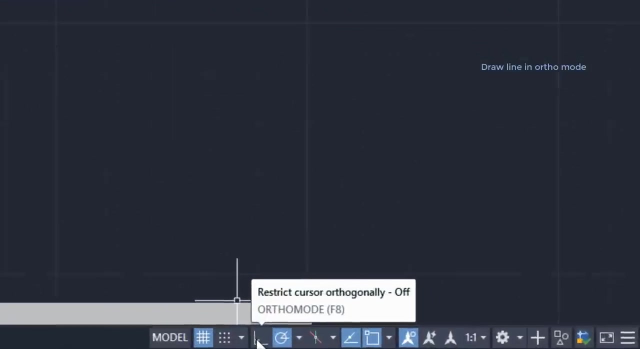 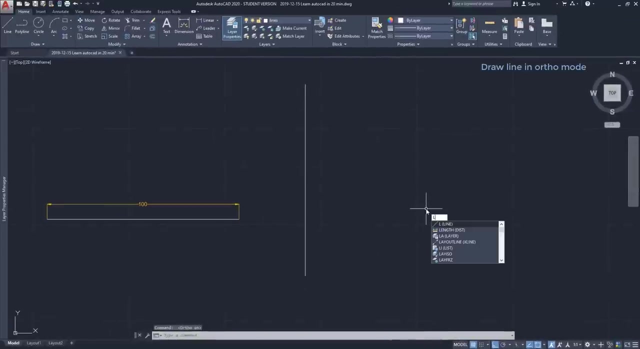 and here you have it: length, 100 or some mode. if I want to add a new one, want to draw only orthogonal lines, I can click on the icon ortho mode, restrict cursor orthogonally. then when I'm drawing a line I can only make it. 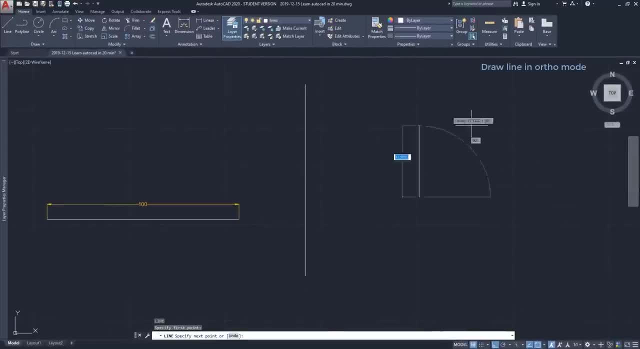 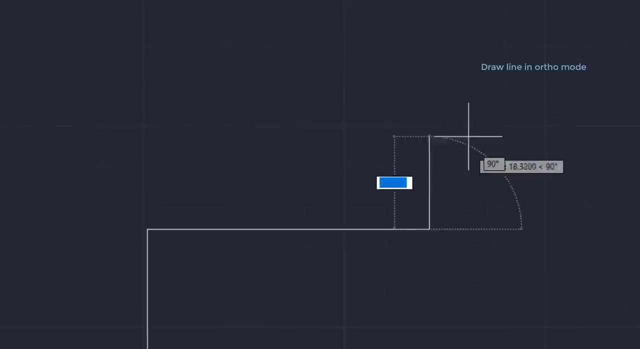 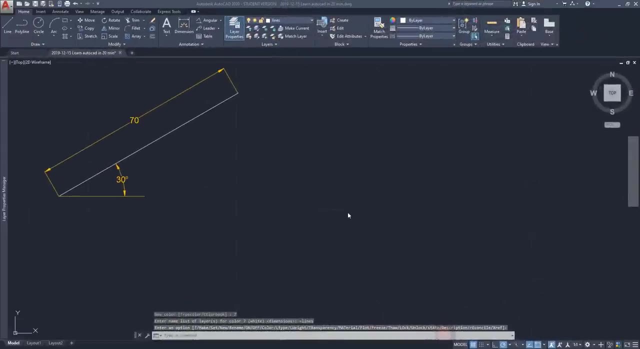 horizontal or vertical. this can be useful if I'm at a part of a project where I just need those type of lines, like in the example here. now let's draw this line here with 70 of length, but with the 30 degrees angle from the x-axis, which you can check looking at the UCS coordinates. they are by default. 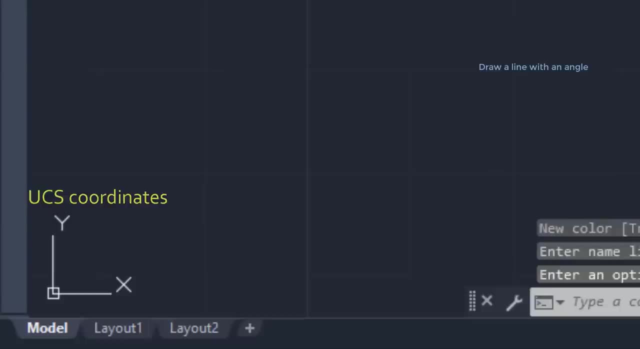 located at the left corner of the screen here. so I draw again a line from the X axis to the right of the screen, from the X axis to the left of the screen. so I draw again a line from the X axis to the left of the screen, from the X axis to the left of the screen. 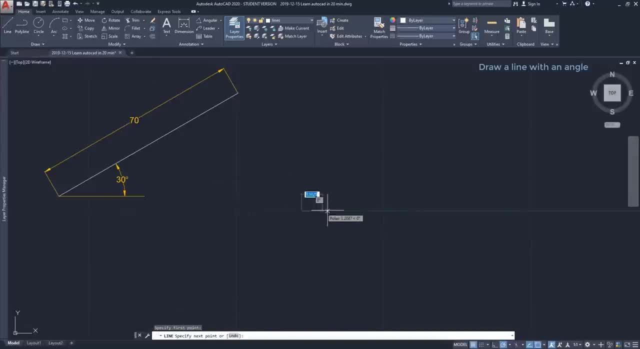 start point. I type 70, but this time, instead of pushing enter, I press the button tab, the one above the caps lock. with this way I locked the length, but I can choose the direction. I place the pointer more or less here, type 30 and press enter. as you see, it's quite simple. then look at: 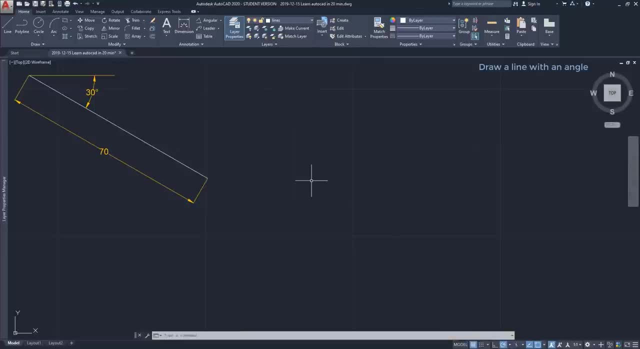 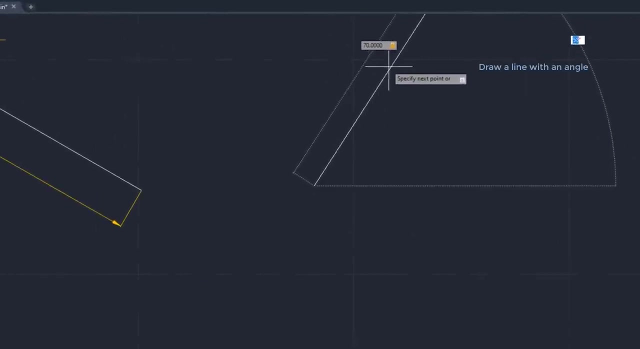 this different situation. the line makes the same angle, but in the opposite direction. I do the same as before. type the length, then look at this label showing the current angle. while I'm moving the cursor around it's increasing until I reach half circle- 180 degrees. then it decreases. 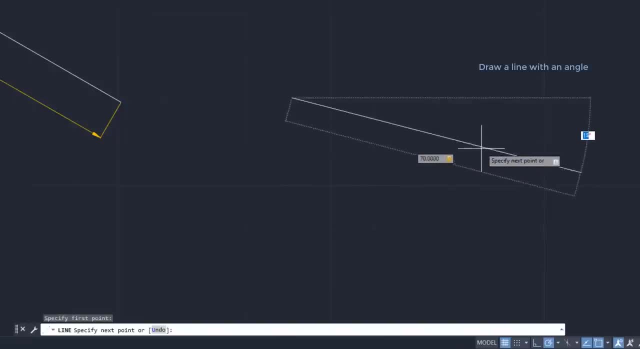 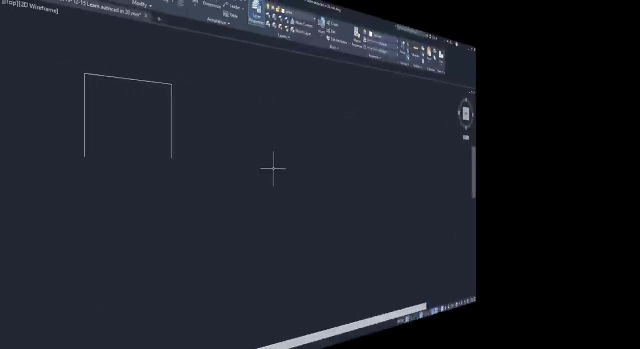 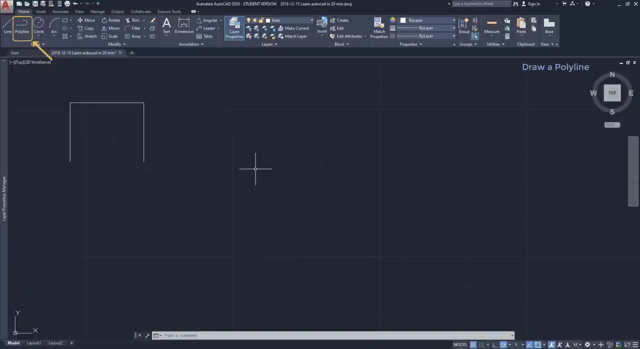 as now it's showing the other side angle. basically, if I'm below the x-axis and type 30, the angle starts again in the same place, but in a clockwise direction. next to the line icon is the polarizing line. a polyline is a connect sequence of lines created as a single object. for example, let's draw: 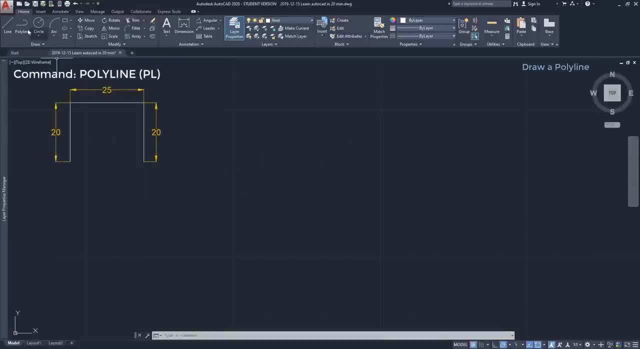 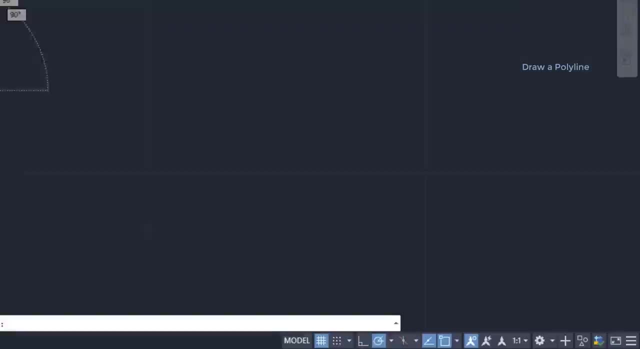 this exercise. here I click in polyline, choose a start point to draw the first line. go up and make sure you have the polar mode switched on. type 20, press enter. then to the right, I type 25, press enter again and finally vertically down. this is important: always click when the polar tracking is. 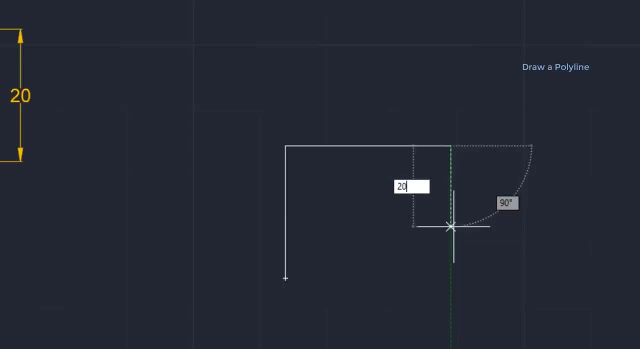 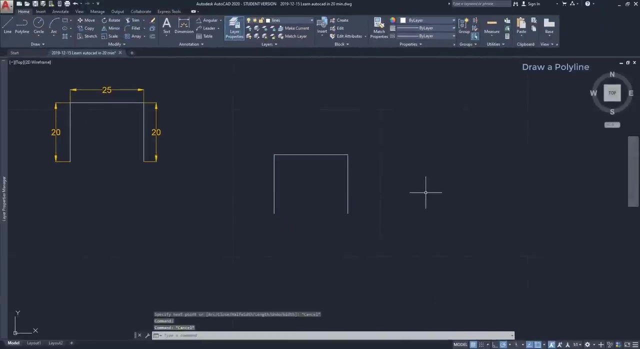 on the screen, type 20, again press enter and escape. so if I click in the polyline, it selects the full sequence. as you see, although I could use the command line to draw the same example, all the lines would be considered as a complete sequence, although I could use the command line to draw the 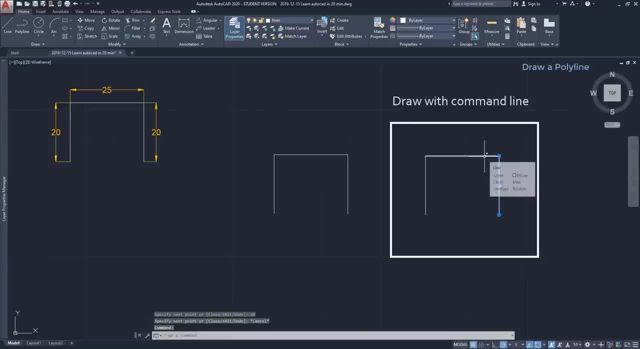 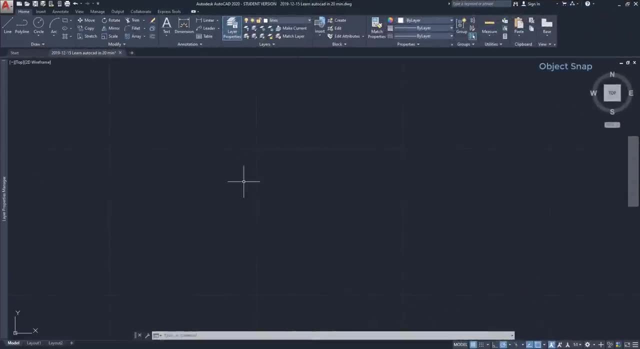 same example. all the lines would be considered as a complete sequence, although I could use the separate objects. now that you know the basics to draw lines, I want to introduce to you a very important function in AutoCAD: the object snap. this will allow us to make our drawings with the maximum precision. take a look at the next. 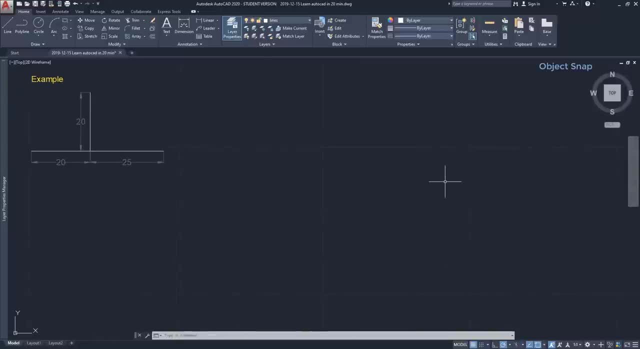 example. let's draw it. I can use either line or polyline command. I choose polyline. I'm going to type its shortcut: PL, draw the first line, then the vertical one. as there is no line to continue here, I press escape. now, the third line has to be connected to the next line, and the third line has to be connected to the next line. 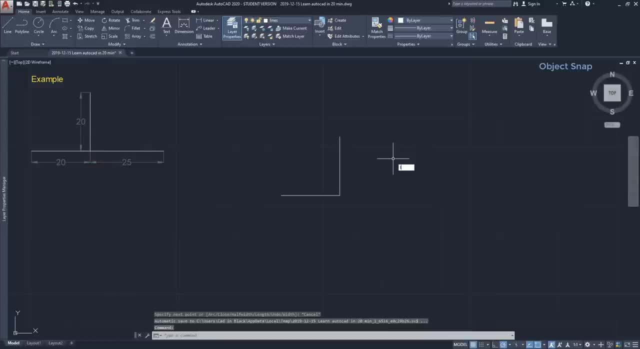 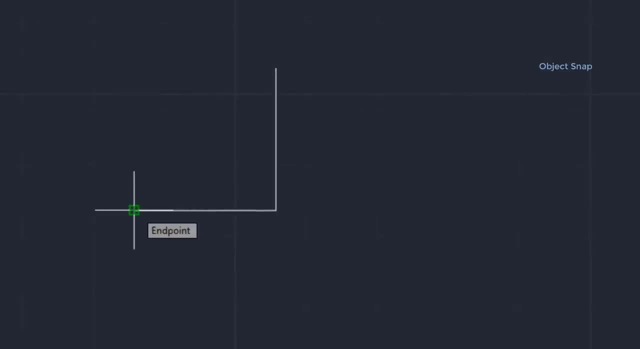 this intersection, I turn on the command line, I move the cursor near the left end of this line and look at this green square appearing here saying endpoint. the same happens when I go to the other side. you can see it again if I click right now. the next line starts automatically from that point and it 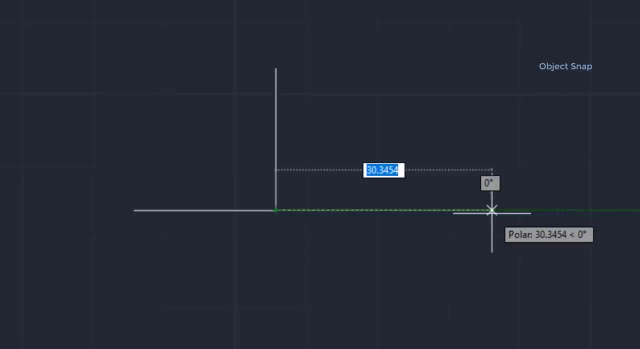 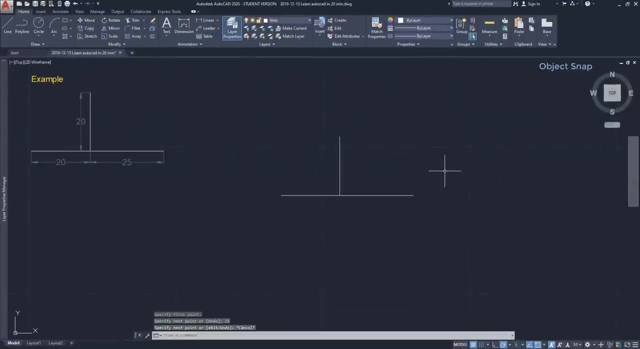 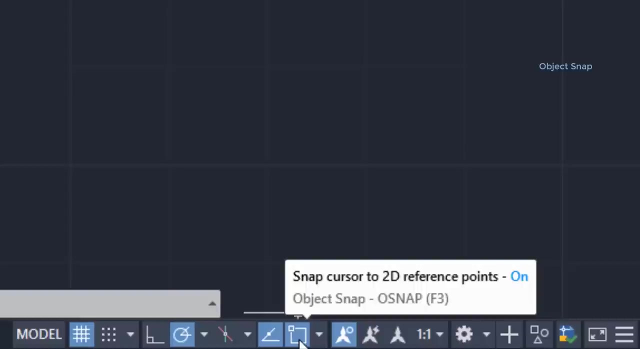 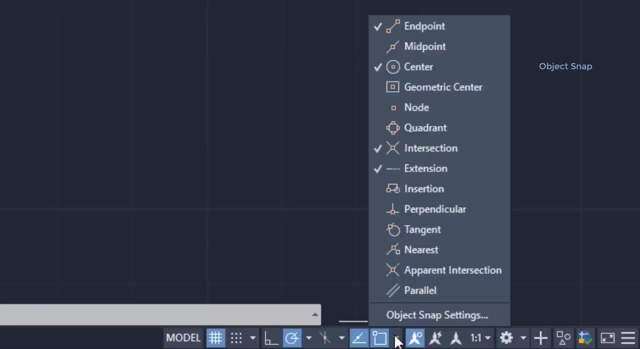 means the three lines are now connected to each other. type 25 and press Enter. those green squares only appear because the object snap is active. it's this icon at the status bar. at the arrow just next I can see the modes that are currently active. see here the endpoint, which is an extremity of a line segment. 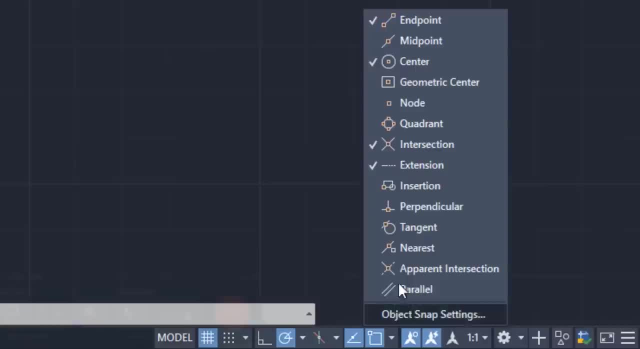 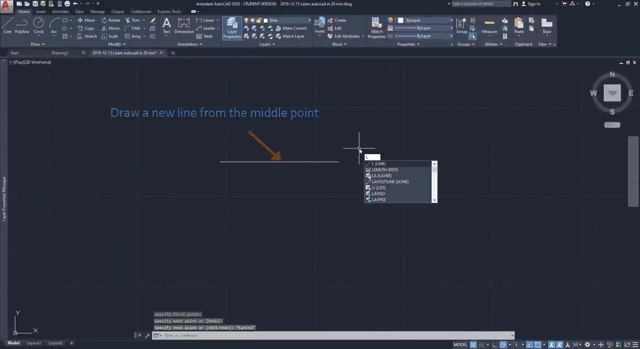 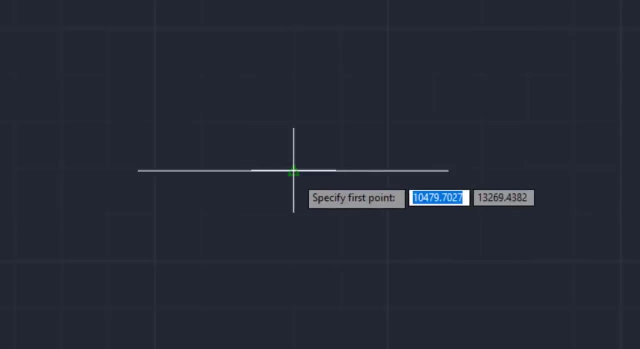 now I'm going to introduce you also the midpoint. first I'm going to click in it because it's not active. then I want to draw a line from the middle point of this one. I activate the command line. as you can see, this triangle indicates the midpoint. I click now and the next line starts exactly from there. 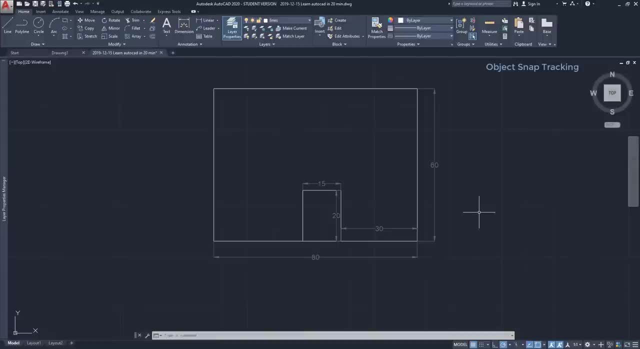 then I move the cursor to the starting point from the middle point. I'll leave it for a while so that I can't miss it. this is a very useful function and I will explain it with an example because I think it's easier to understand. we have this example here and we want to draw. 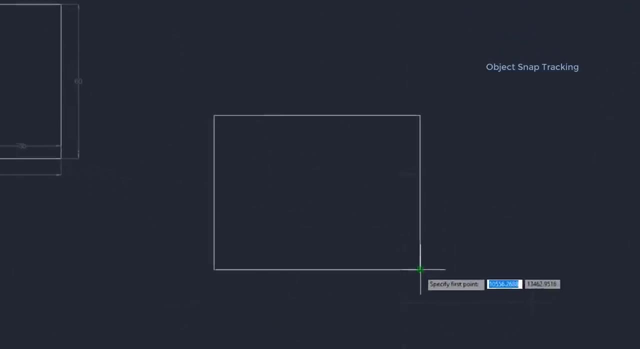 this line, which is located at a distance of 30 from the right. I turn on the command line left slowly so that I see this label that says extension. in this moment, if I type 30, the new line starts with that distance from the end point. it's simple. 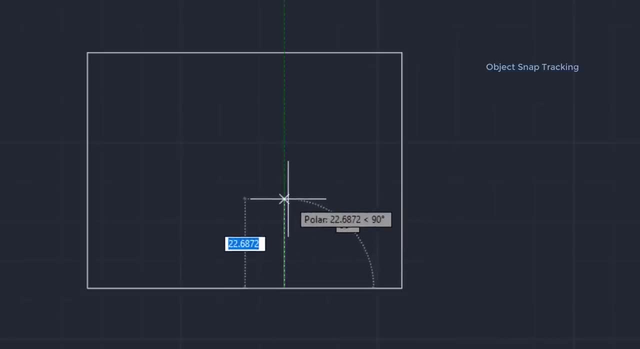 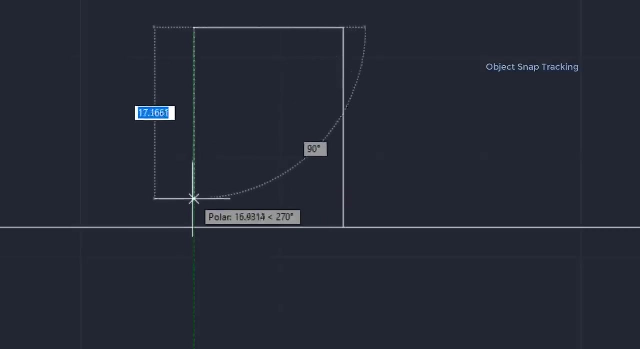 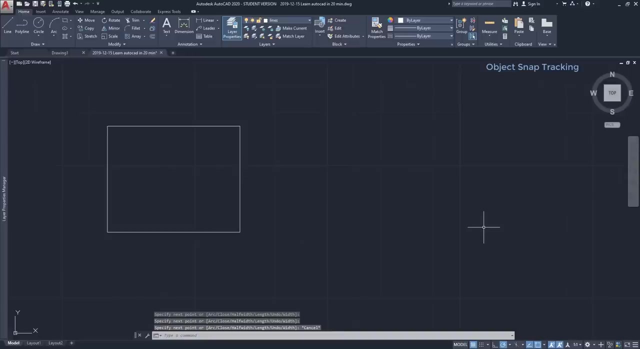 and with this we can avoid drawing extra lines. then you just need to draw the remaining objects to connect this line with the rectangle below. drag it down until I see this cross here. now click and press escape. another way to use object snap tracking can be when I am drawing this rectangle. 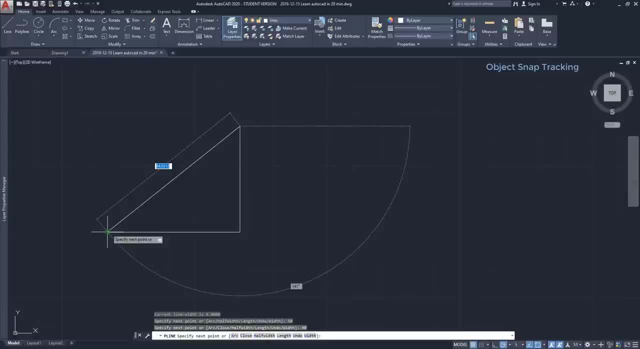 I can draw an extension line up from this point until I intersect the polar tracking of the line I'm making like this. so this kind of things are very interesting to play around. now you need to make a bit of practice to strengthen the knowledge you got in this. 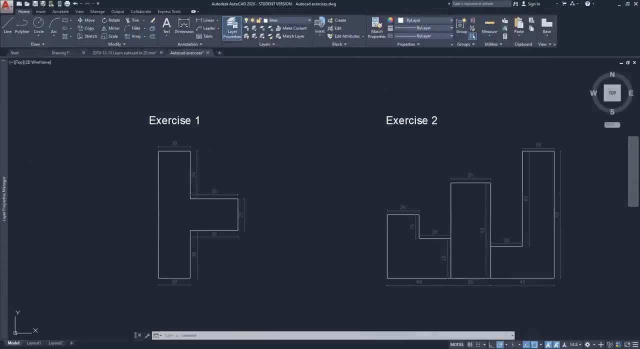 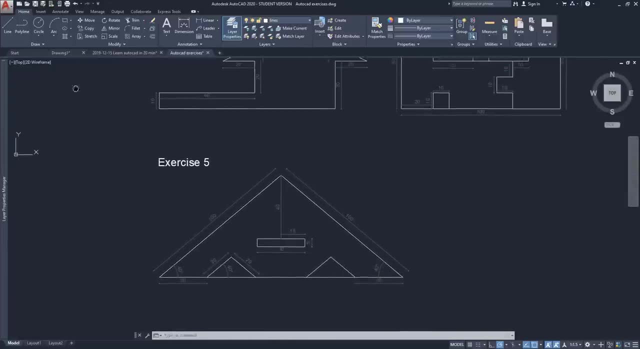 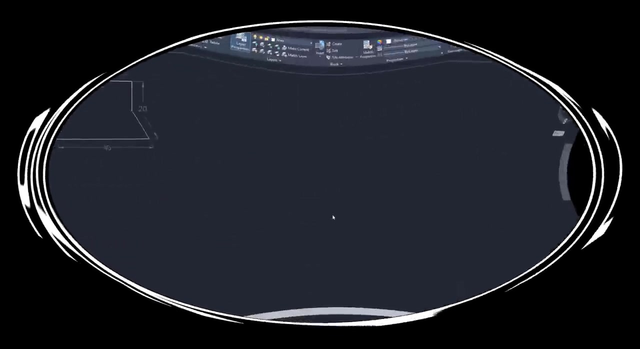 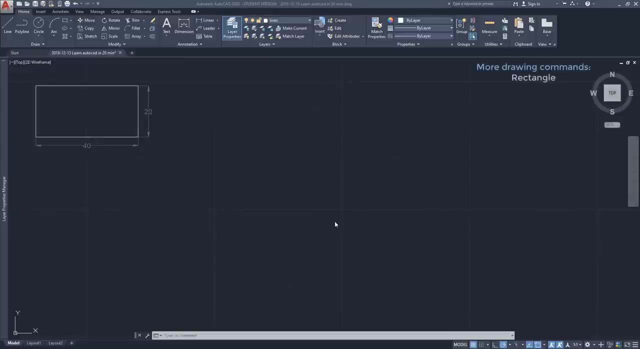 video. for that reason I prepared these exercises for you. you can get them in PDF by clicking on the link available in the description. part two: I am going to explain to you briefly more drawing commands- rectangle. a rectangle is in reality a polyline. it's just a faster way to draw this kind of 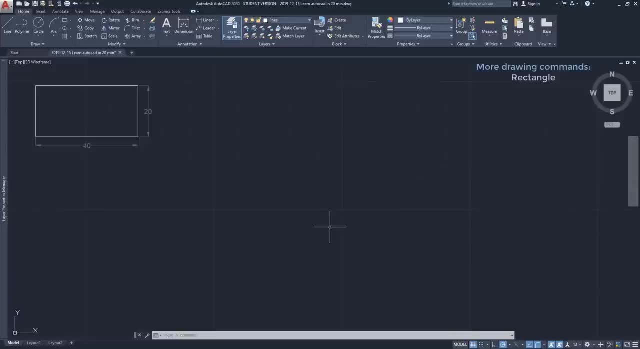 objects. as I just need to specify two points, I'm going to show you the command is this one: specify the first point And then I only need the opposite corner. I can simply click to place it or insert the coordinates regarding the first point. That's what I'm going to do. 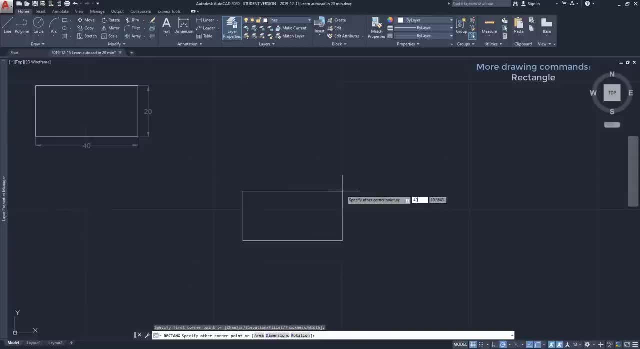 The first blank is for the x-axis Type 40. Then I press Tab to switch to the second coordinate- This one is for the y-axis Type 20- and press Enter again. In fact, what I have done was inserting the length and the width. 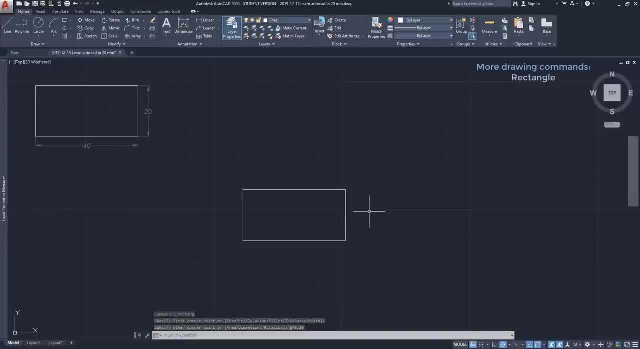 Simple. However, as I still have to take into consideration the UCS coordinates, sometimes the values might be negative. Let's suppose I draw another rectangle, but with the start point The x-coordinates would be minus 40.. Click for the start point. 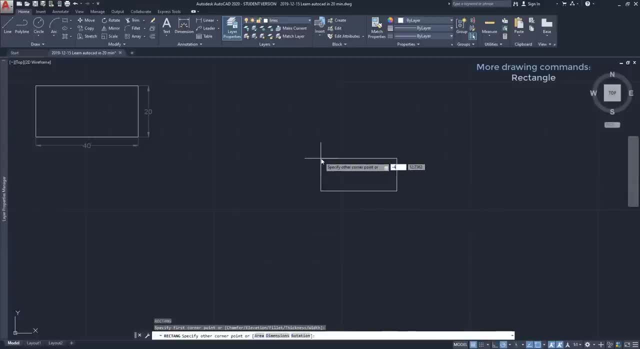 Then type Minus 40.. Press Tab And as the y-coordinates are positive, I type 20.. Here you have the result Circle. To insert a circle in AutoCAD, I can click in this icon, as I believe you guessed. 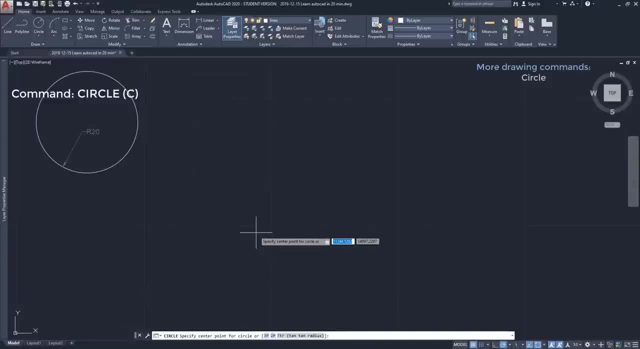 Then just follow the prompts. to draw the example here: Specific- Specify center point of the circle. OK, I click anywhere. Then Specify radius of circle: It is 20.. I type that value and press Enter. Let's do the next. 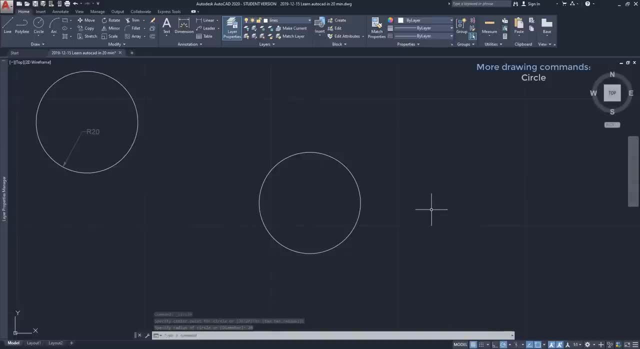 Now check out this tip, As I want to use again the command Circle. press Enter. the system automatically reactivates the previous action. This is very important to know. It saves time. I am going to draw the same circle again Now. look to the prompt at the command bar. 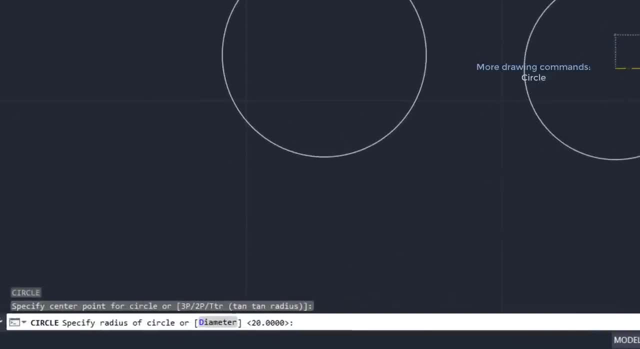 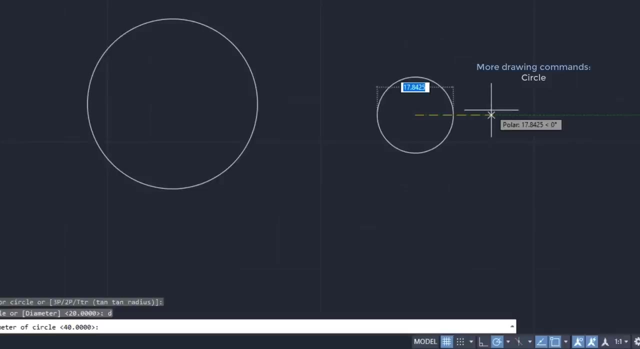 Specify radius of circle or diameter. So instead of typing a radius, I can switch to typing a diameter. I do it by clicking on it, or simply type the first letter, D, Then press Enter. As I am drawing a circle, I am drawing the same circle. 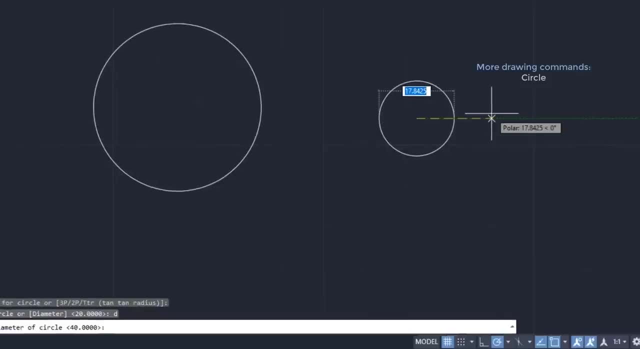 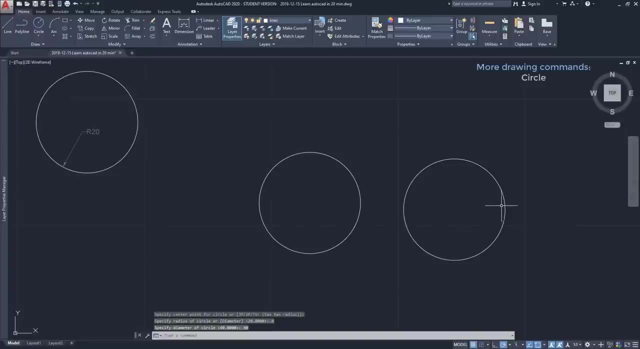 The value is two times the radius 40.. Press Enter again, As I am drawing the same circle. the value is two times the radius 40. Press Enter again. OK, This is just one of the several ways to insert a circle. 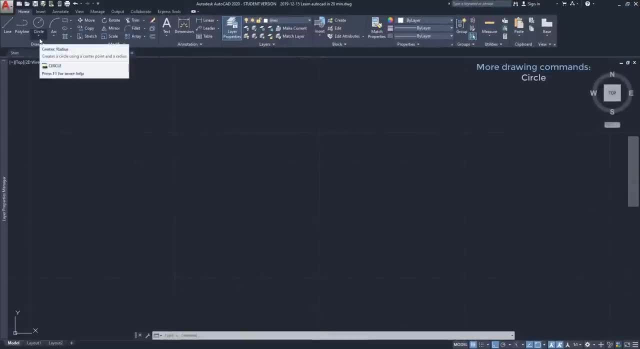 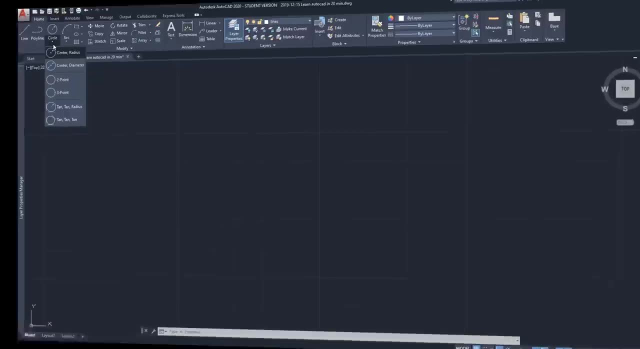 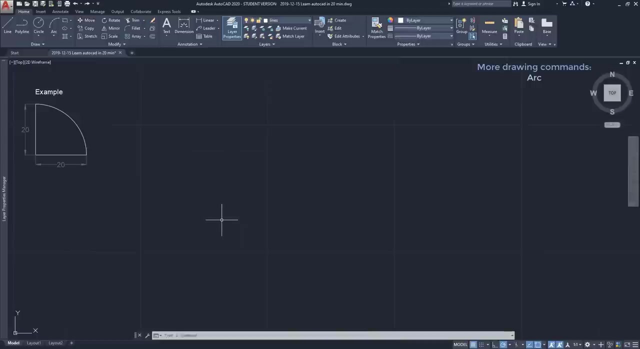 If I click on the arrow below the icon, you can see all these options available. That depends the situation that you are drawing Arc. An arc is a segmented circle, is a section of a circle and, like the previous command, there is an arrow below. 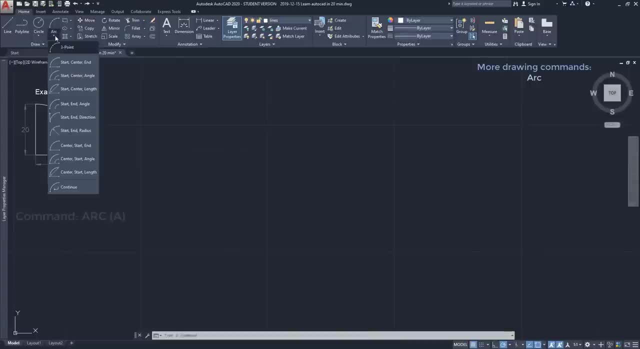 the icon with different ways of specifying points. I'm going to draw the arc of this example above, and the best option here is inserting the start point, then the center and finally the end point. by default, AutoCAD draws the arc in the clockwise direction. let's click on the arrow, then find start, center and 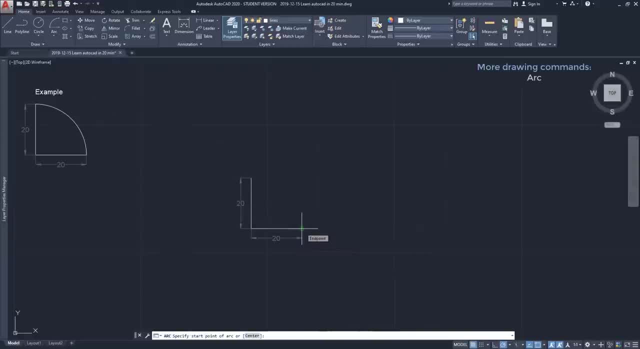 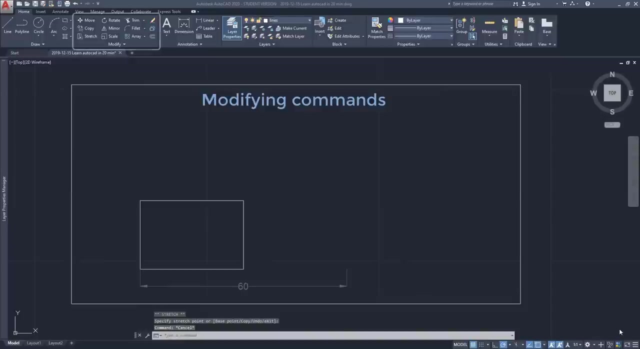 click on the end point of this line. for the start point, the center is the intersection between both lines and finally, the end point is this one: see how the arc is being drawn, clockwise, modifying objects. until this moment, I taught you the most used comments to draw in AutoCAD. in this section, I will introduce to you comments that will help. 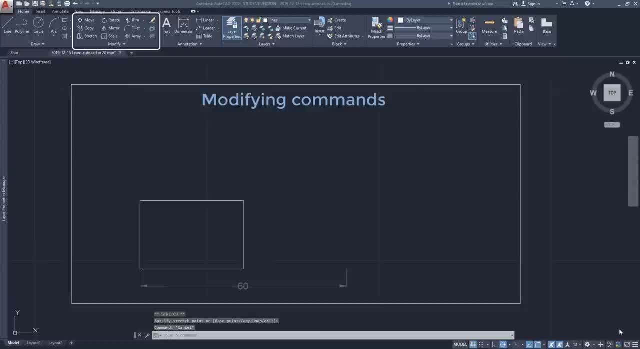 you in modifying objects and to be more effective while drawing. I'm going to start with the basic ones: move to move an object to a different place. for example, want to move the small object or the blue object rectangle to a distance of 60 to the right click on the icon, select the 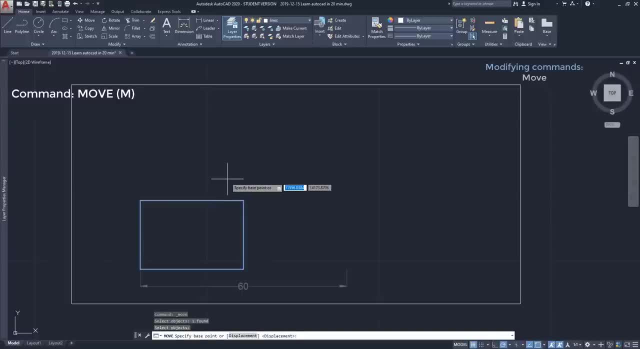 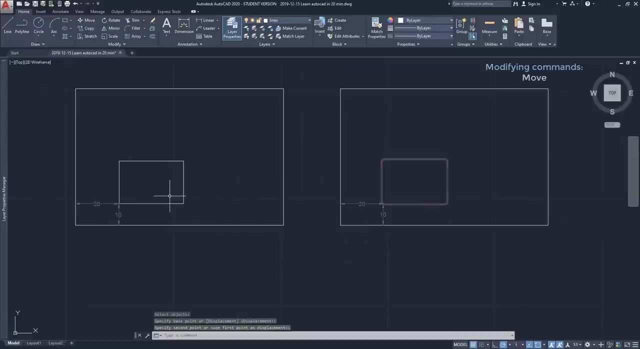 rectangle, press ENTER. specify a point from where I want to move the object. then I move to the right horizontally and type the distance of 60. press ENTER. in the following example: I want to move the rectangle to the other box which is located at the same distance from the corner as here. I activate, move again I. 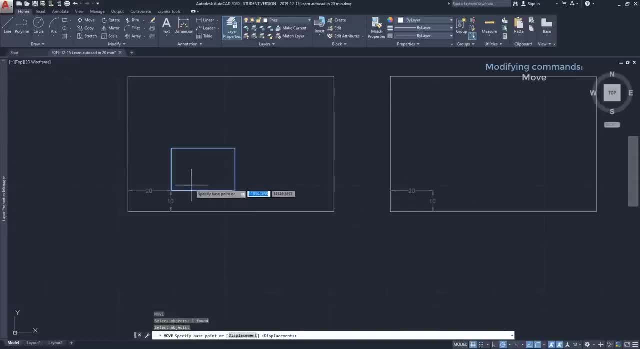 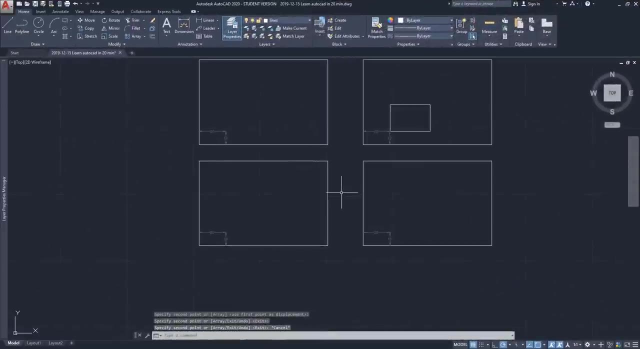 select the object, press ENTER. but this time the base point it's going to be the corner. then I click in the next corner to move it there. copy. this command works in the same way as the command move. I'm going to copy the object to the first rectangle. 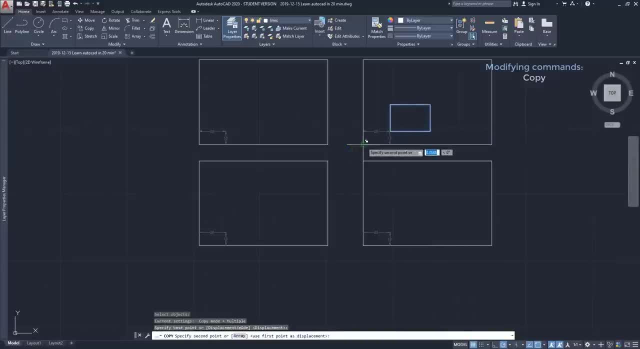 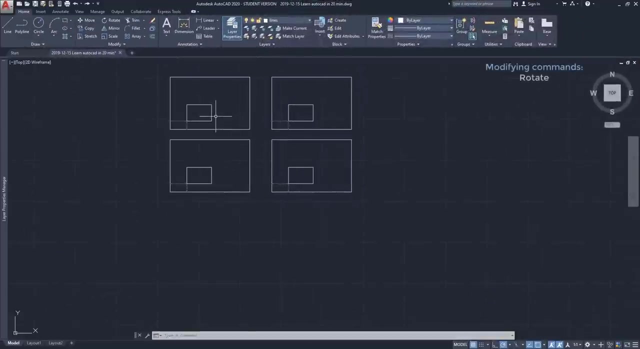 I use this base point, then I can copy it in this intersection. then I realize I can keep copying the object the number of times I want. do you see? it's very nice this. and when I'm done I press ESCAPE- rotate- to rotate objects. I can use this command. let's see how it works. I click. 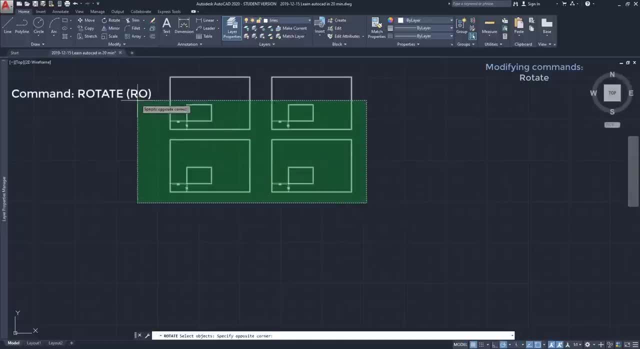 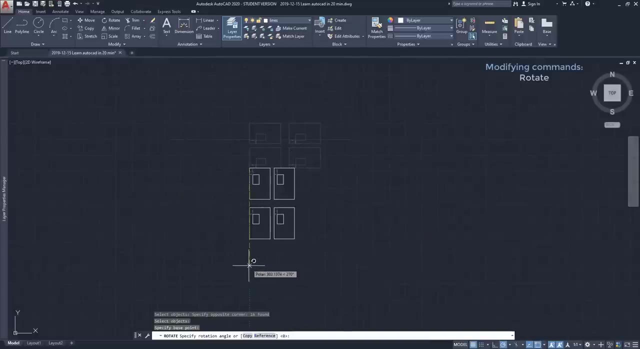 on the icon select the objects, press ENTER. then I choose a base point where the objects can rotate around it. as the polar tracking is on, I'm going to rotate them now 90 degrees to this side. another situation: the same objects are in this position if I try to rotate them back. 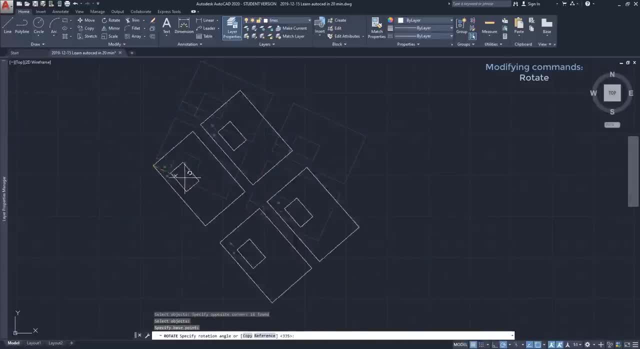 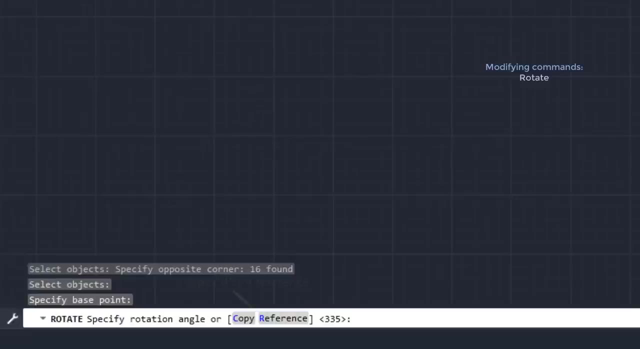 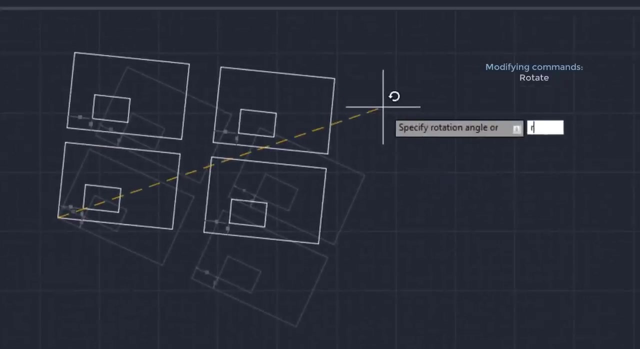 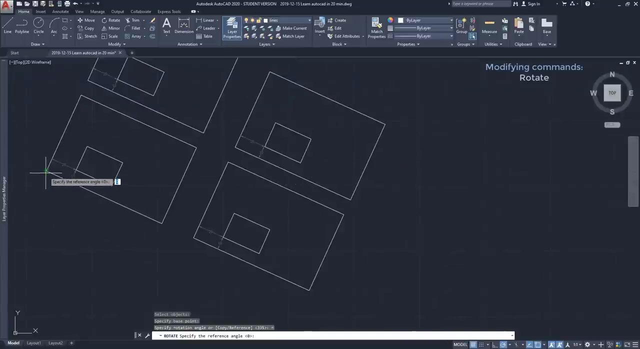 to the position they were before. the polar tracking doesn't work this time. however, I can use a different way. if you look to the prompt, there is an option that says reference. to use it, I can either click on it with the mouse or type R. usually the first letter is enough. after I can specify a reference angle or draw a reference line. let's do a reference line. 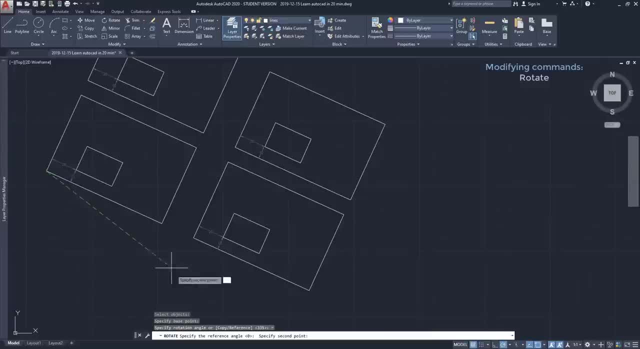 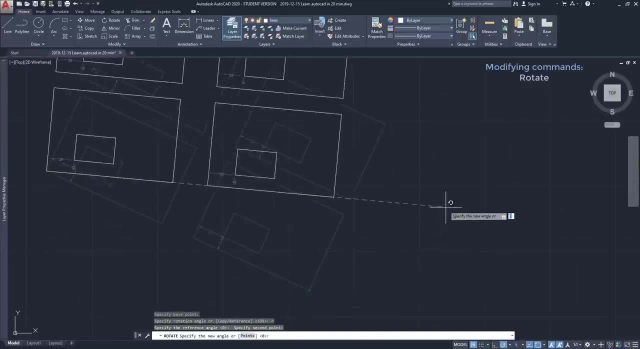 that prefer this. click here for the first point, then for the second point. I chose this end point. finally, I can rotate until the polar tracking and this is done. then I can select a reference point right here and I can also switch between the reference and reference lines. 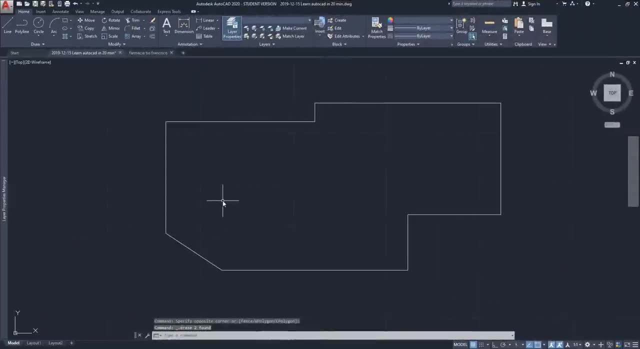 appears. now. look at this polyline. with the command offset. I can inscribe that polyline inside with a specific distance. that distance is called offset distance and it has a length of 10. in this example- let's do it- the icon offset is this one. clicking it then for specify offset distance, I type 10, select the. 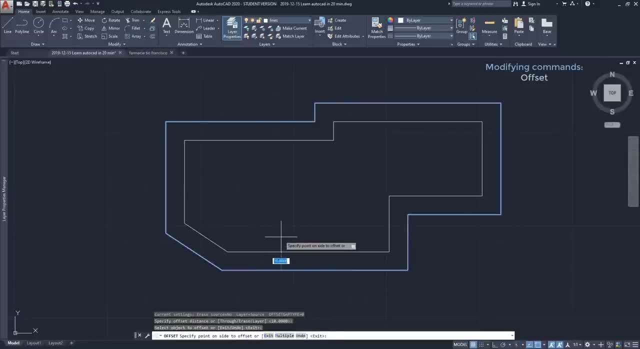 polyline. I move the pointer inside and click there to draw the new polyline. by the way, if I click outside the area, the new polyline offsets outside the original one. the command offset can also be applied to lines. if I have this line and apply offset to it, a new line shows up parallel to the 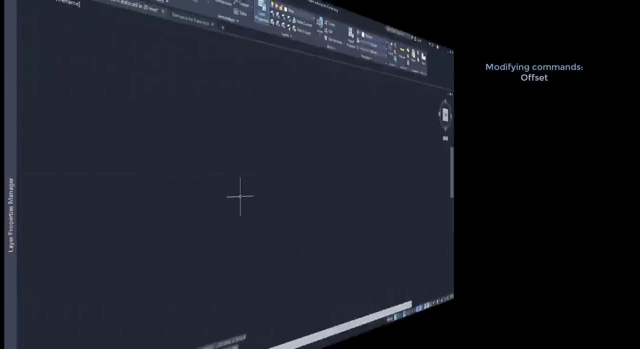 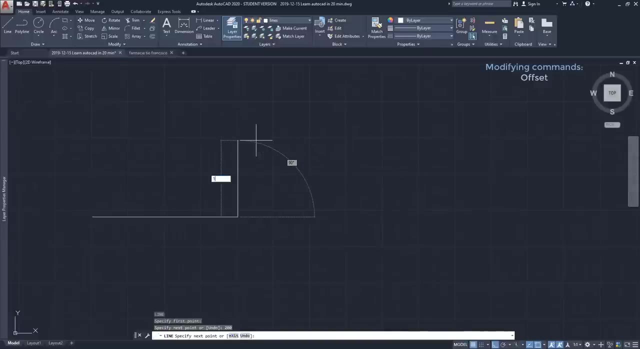 first one. now I want to show you a situation that happens to a lot of people. I'm going to draw a rectangle with the command line, then I want to offset the lines, like before I type O to activate the command, specify the distance of 10, and when I click to offset, I realize I can only click on one line at a time and 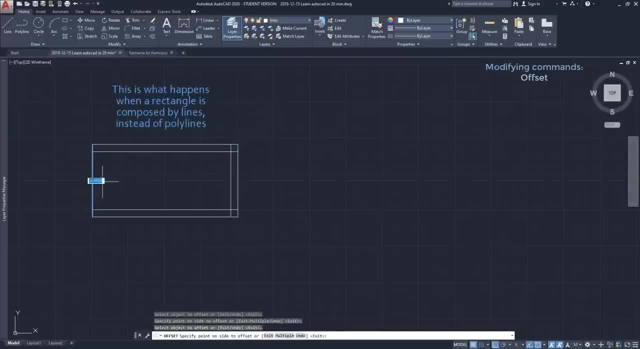 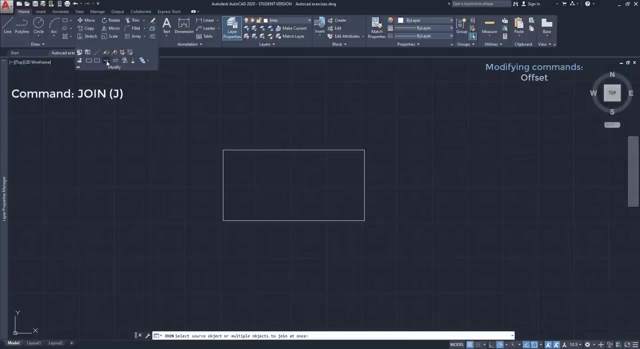 the result is different than when I applied to polylines. however, I can easily merge lines in a polyline. there is a command for it, join. I type join, or I can still find the icon on the modify panel here. it's very simple: select the lines to merge and press enter. 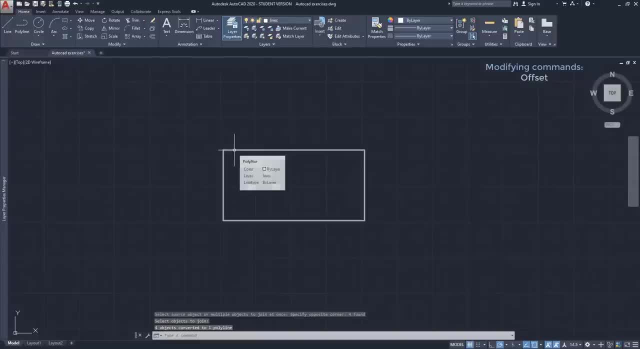 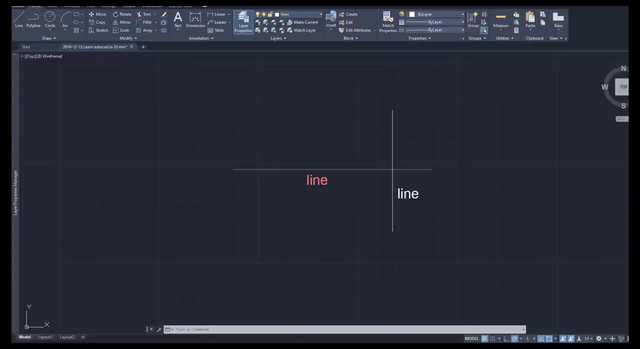 as you see, now I have a polyline. finally, if I do offset again, the result will be identical as my first example: command trim. in AutoCAD we often need to cut parts of objects we have drawn before. for that we can use the command trim. let's check out. 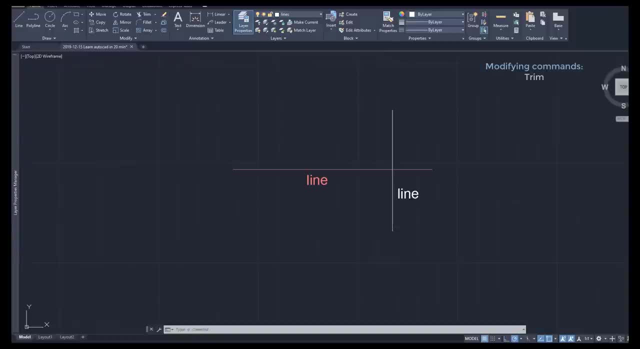 how it works. I'm going to start with a very simple example. we have these lines and I want to erase this segment. I click on the command- trim is located there. select both lines, press ENTER. then if I drag the pointer over here, the screen shows that this part will be. 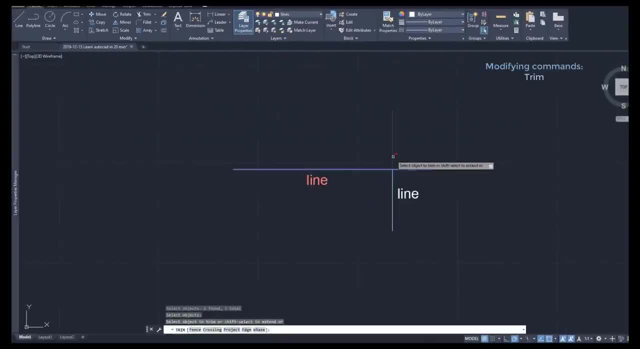 erased. the same happens when I move the pointer to the other segments. I click on this one and you see it disappearing. it's done to leave the command, press ENTER or ESC. look to the next example. this time we have three lines. I turn on trim again, select all the objects and then I can erase any segment between any. 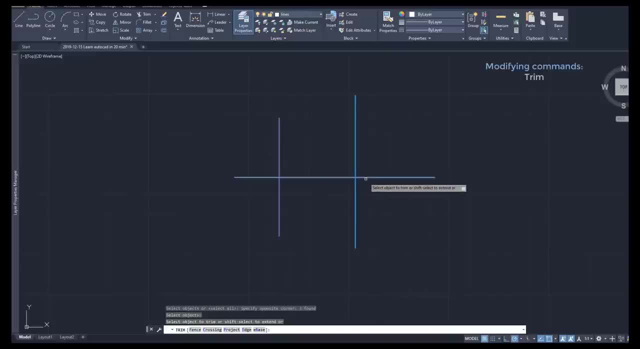 intersection, as you see now. suppose I want to erase all this part of the horizontal line. turn on, trim the vertical line on the right. I don't need to select just the other two, press ENTER and when I'm going to click on this line it erases. 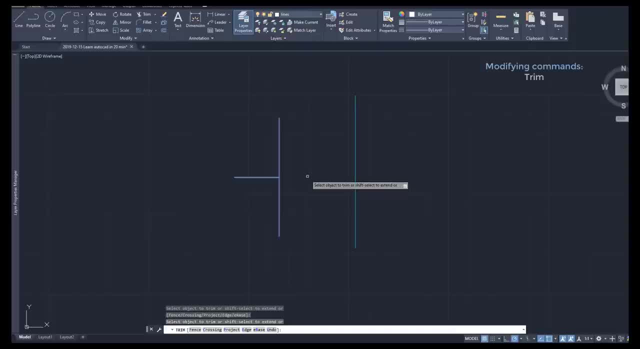 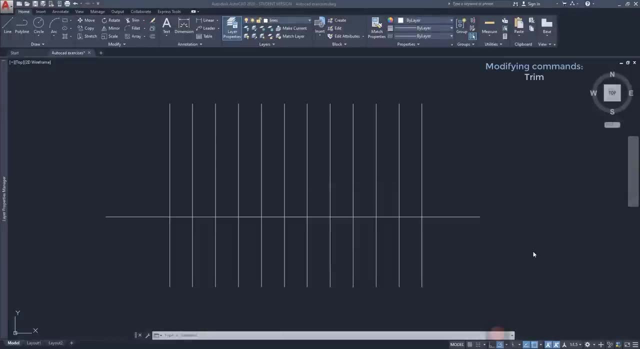 everything from the intersection of the lines I have selected to the right. maybe for this situation this didn't make a big difference, but look at this case here. I want to delete all this part of the line so I can erase all the lines that I have selected. 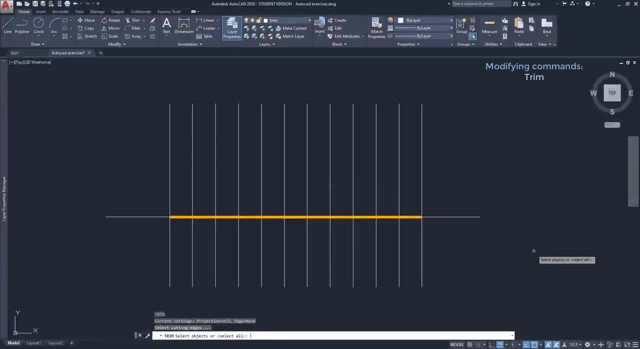 maybe for this situation this didn't make a big difference. but look at this case. here I want to delete all this part of the line line. if I select everything, then I need to erase one by one. it takes a long time, so it's better to only select the lines I'm going to use, like this: 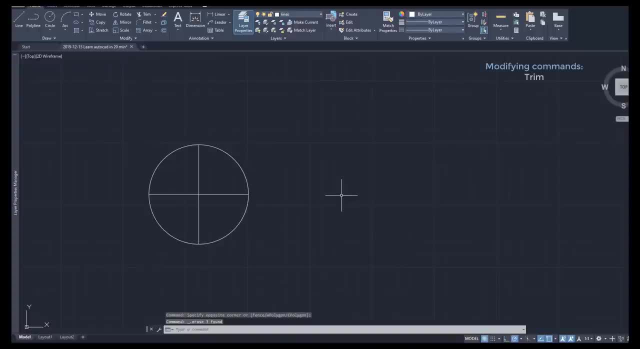 of course I can use trim not only for lines. it works for other kinds of objects, for example. I want to change this drawing to that. of course I can use trim not only for lines. it works for other kinds of objects, for example. I want to change this drawing to that. 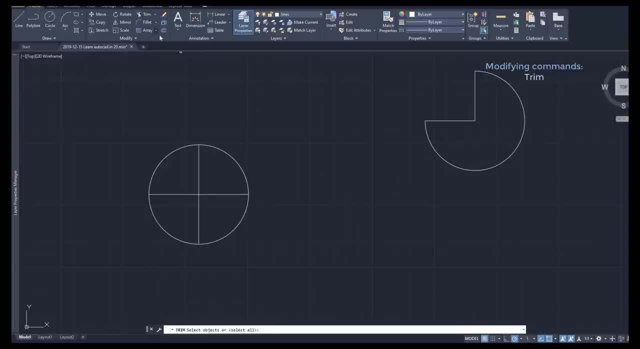 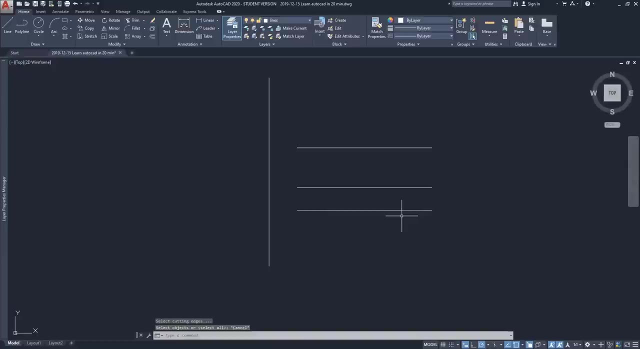 one. I activate stream, select everything, press ENTER and finally click on the parts to erase. extend. this command is used to extend lines. in the example here, I want to extend this line to intersect the vertical line on the left. I am going to click on the arrow located next to the command tree, then I select. 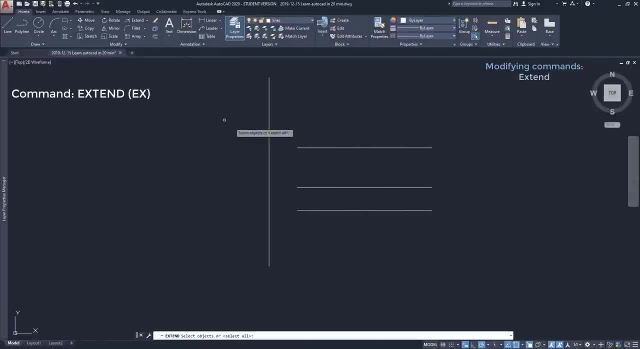 extend. first I have to select not the line that I want to extend, but the one where the extended lines will connect. so it's this one. press ENTER, then I select the line to extend. to extend the line to the left, I have to click on the the left half in order to work. Look, if I drag the pointer over the right half. 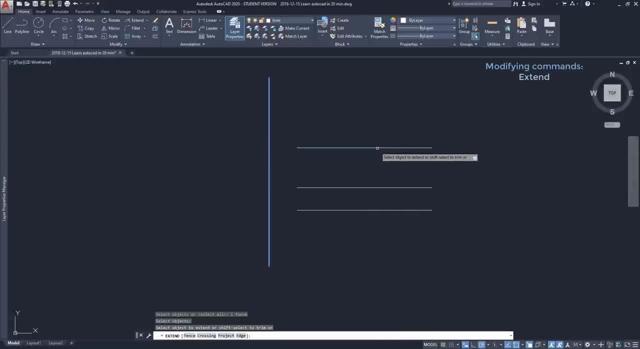 nothing happens. I go slowly to the left and after passing the middle the extension appears again. I click and press ENTER. In this example, I want to extend all the vertical lines on both sides. I type EX, press ENTER. Select both horizontal lines. press ENTER again To extend the. 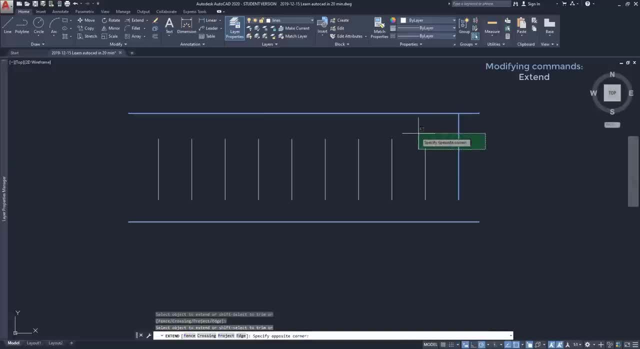 lines up. I can open a selection area to cover the upper part of all vertical lines. I click, then I do the same for the part below to extend the lines down. When I finish, I press ENTER to exit the command. Of course, in this situation there is a faster procediment by opening an area that. 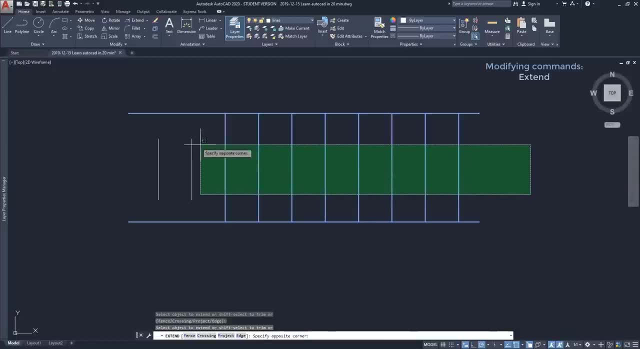 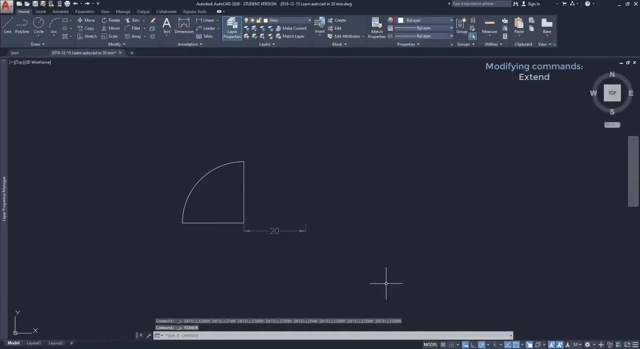 covers both line sides. That extends both parts in just one step Mirror. With this command, we can copy objects symmetrically. This is how it looks. Also, when we need to make a symmetrical drawing, we can just draw half of it. 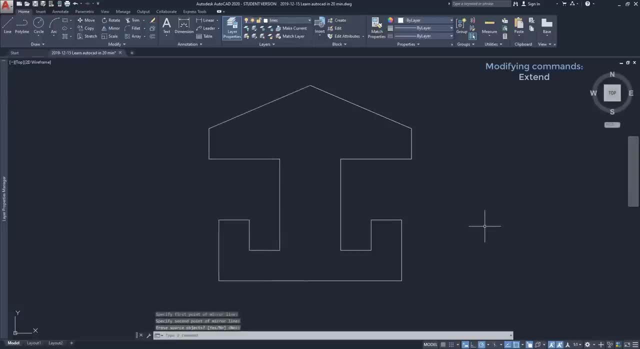 and then use Mirror in order to complete the process without spending time in drawing. Let's see how the command Mirror works for these objects. Click on the icon select everything and press ENTER. Then the prompt asks me to draw a mirror line. I'm going to insert the first point at a distance of 20 from the objects. 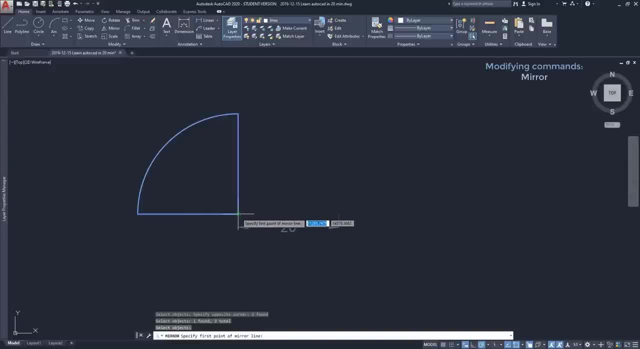 I put the mouse over X2.. this endpoint: move right, type 20, and press enter. I'm going to draw the line vertically and you can see everything reflected as a mirror. I click for the second point Now. the prompt sentence says: erase source objects. I choose no to. 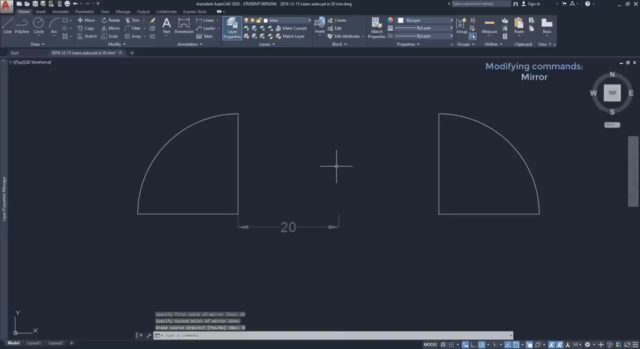 keep the original ones. Notice that all lengths are kept, including the distance between the objects and the mirror line. Now check out these considerations about command mirror. It doesn't matter the length of the mirror line, just the direction. As you can see, if I draw a long vertical line, the result is the. 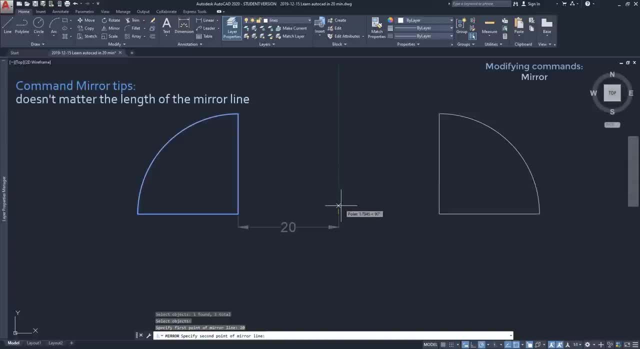 same. Only if I rotate it, the objects are placed differently. To make a symmetrical drawing, I just need to draw half of it, Because If I draw a vertical mirror line in this end point, the new mirrored objects connect to the original ones. 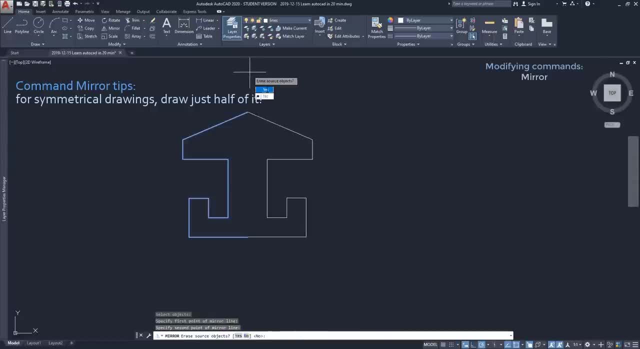 It's simple. Sometimes I don't want the original objects. In the option Erase Source Objects, I choose Yes. That's the result. Editing Objects Using Grips. The blue icons that show up when I select an object are called grips And they allow me to edit it. 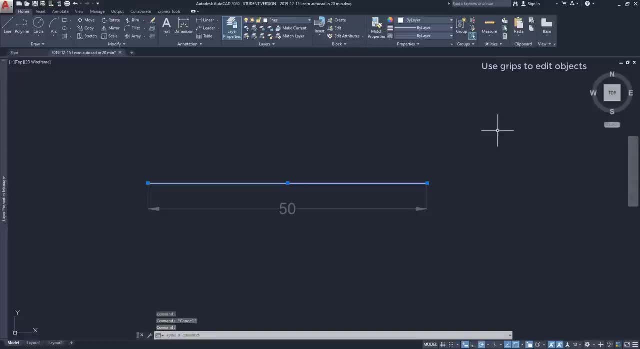 When I select a line, there are three grips. If I click in one at the extremity, I can change the position of that point, keeping the other end in the same place. If I click on the grip in the middle, I can move the line without changing the length and direction. 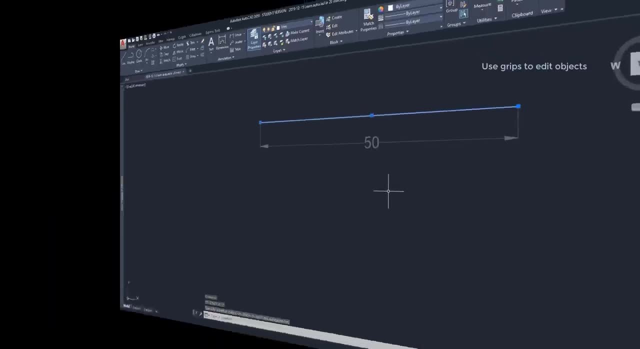 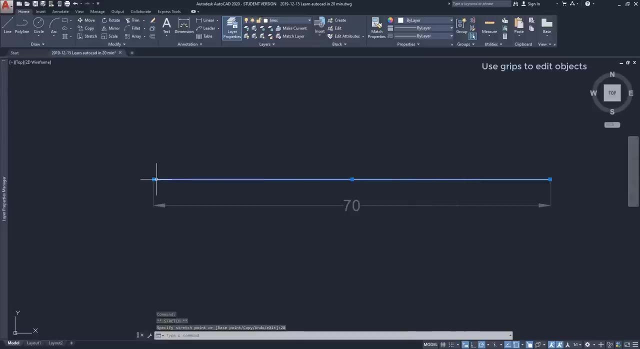 Now let's see some editing tips. Change the line length by moving one of the ends. I'm going to click on this icon. I drag left, I'm going to type 10. And the line length increases to 80.. Of course, this also works if I want to make the line shorter. 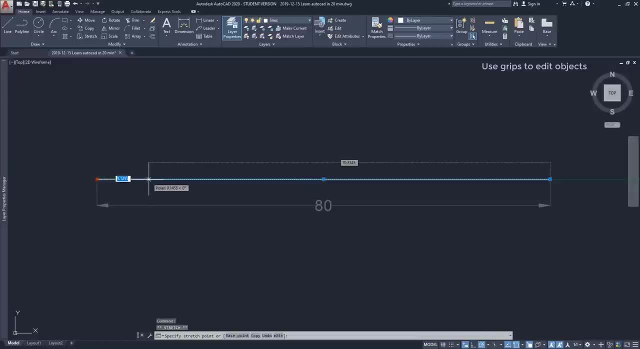 Click again. This time I drag right, type 10, and the line returns to its previous size. Editing Objects Using Grips. If I want to type a new length to the line, I click on the grip, drag left, and this time I press the button TAB and the input switches to the full length. 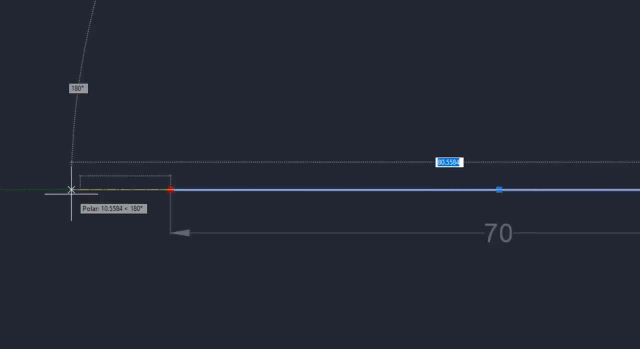 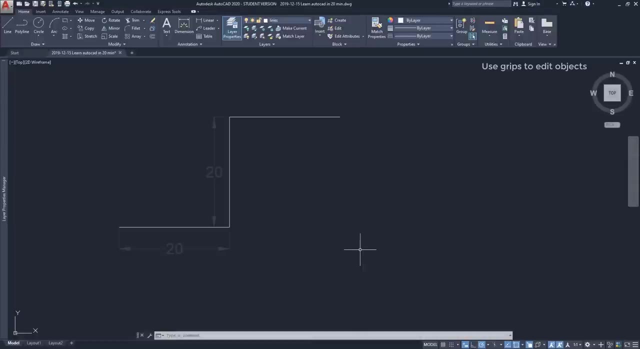 Editing Objects Using Grips. I am going to insert 120. Editing Objects Using Grips. Then let's check out how grips work on polylines. Editing Objects Using Grips. The end grips of each line works in identical way. Editing Objects Using Grips. 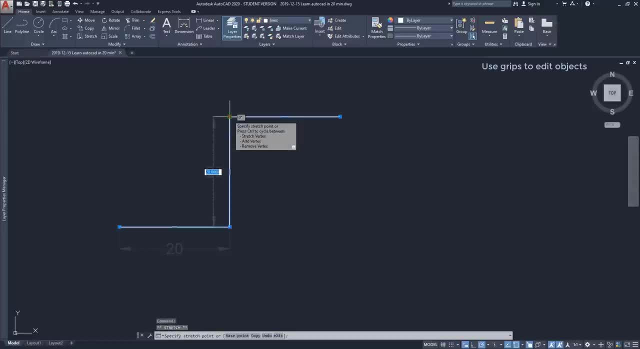 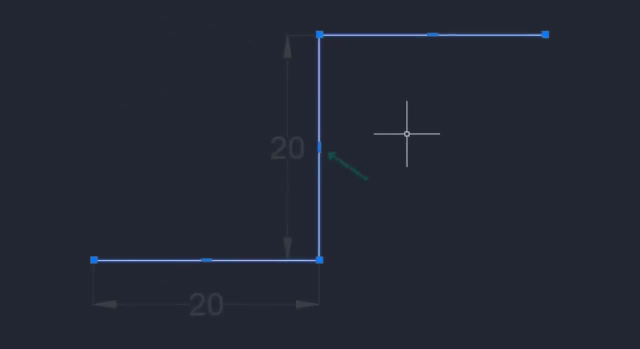 I click on this one to change its position and you can see all the other vertexes don't move. Of course, this may cause me to deform the polyline Editing Objects Using Grips. Now, unlike the lines, the grip on the middle has a rectangular shape. 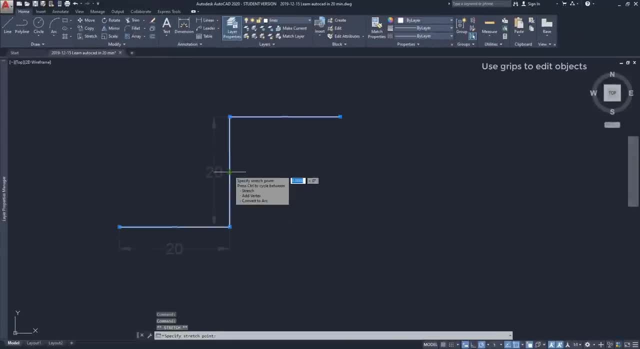 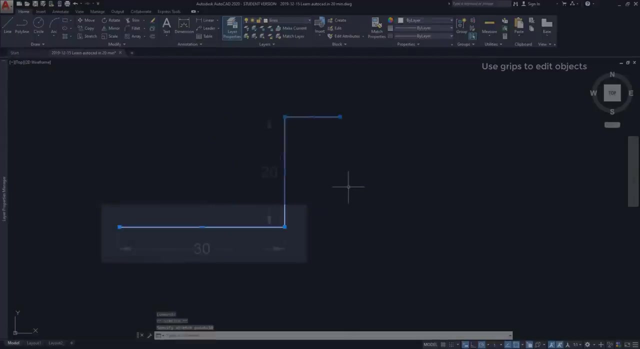 I'm going to click on one and I can move that full line. Then the rest of the polyline has to adapt to its new position. Editing Objects, Using Grips, For example, I move right, type 10, and you can notice this line increases 10 of its total length. 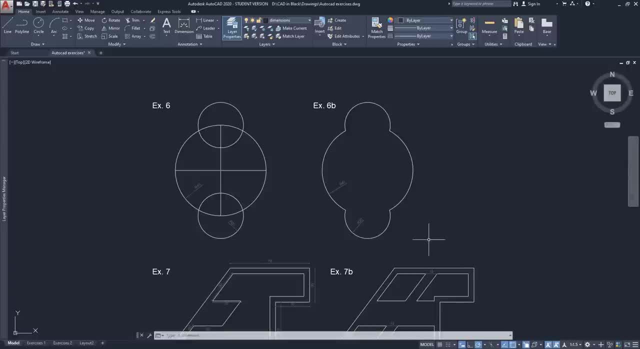 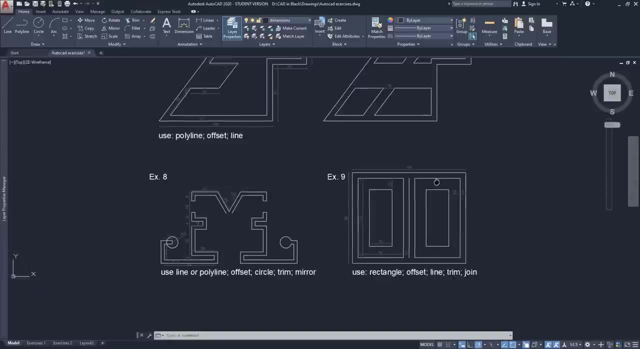 Editing Objects Using Grips. So we reached the end of the second part of this tutorial. Now I prepared more exercises for you in order to practice what you have learned here. The link is in the description of the video: Editing Objects Using Grips. 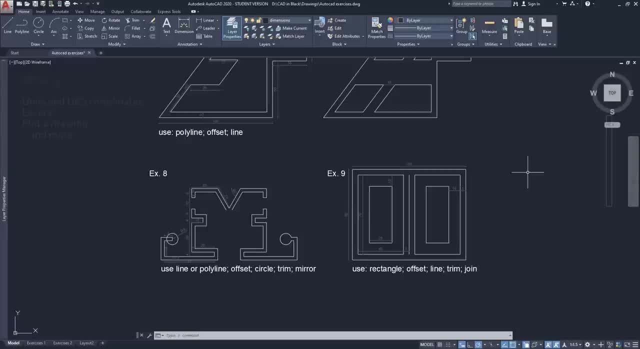 After: don't miss the third part of this course, As I will keep teaching very important features for beginners. I'll set up units, work with layers, plot a drawing and more. Editing Objects Using Grips. Part 3: Editing Objects Using Grips. 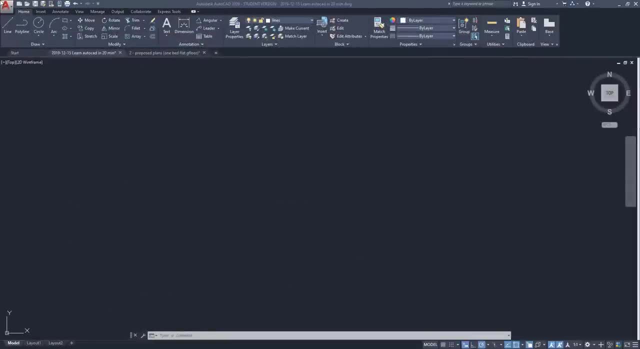 Until here I taught you commands to draw objects and modify them, But I haven't mentioned any units for the dimensions. When I was drawing lines, I said: Draw a line with dimension of 50, or 100. I didn't say if it was meters, millimeters, inches or feet. 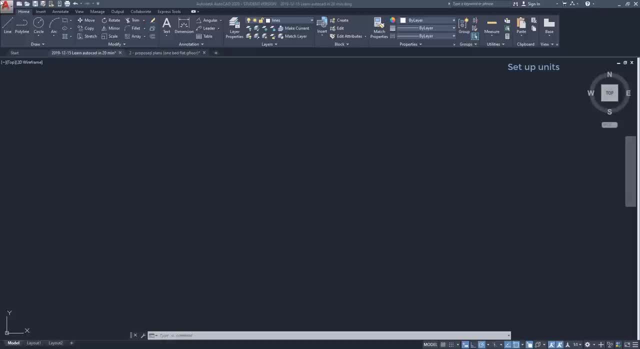 But I'm going to talk about this now. First of all, AutoCAD uses a-dimensional units. This means that it's up to me to decide what is the unit of a line that has length of 20,, 50, or 100. 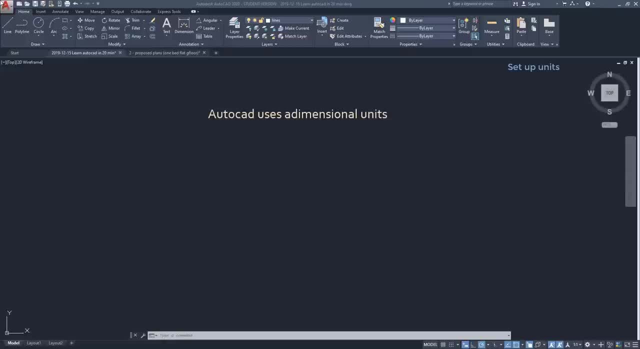 It's very simple. Let's suppose I want to make a project in millimeters. That's the unit I usually want. I want to insert a line with 5 millimeters of length. I draw the line as usual, and when I want to set up the length, I type 5.. 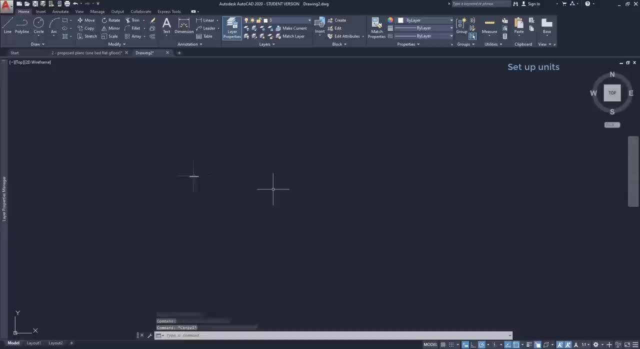 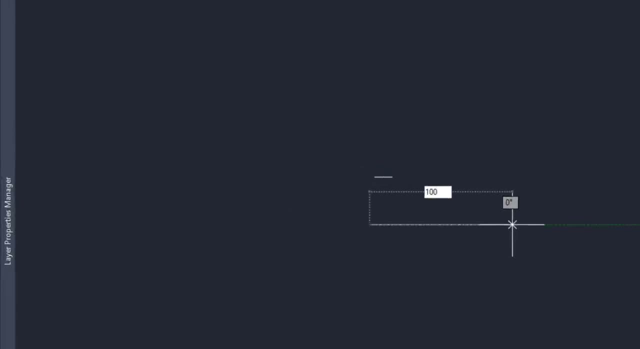 Then I'm going to insert a line that measures 1 meter. I do the same, but this time for the length I type 1000. Because, as you may know, 1 meter is 1000 millimeters. 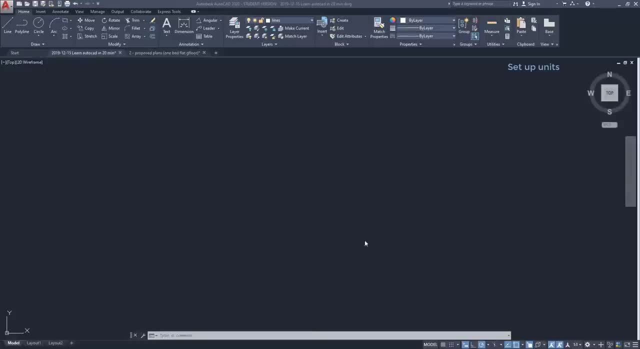 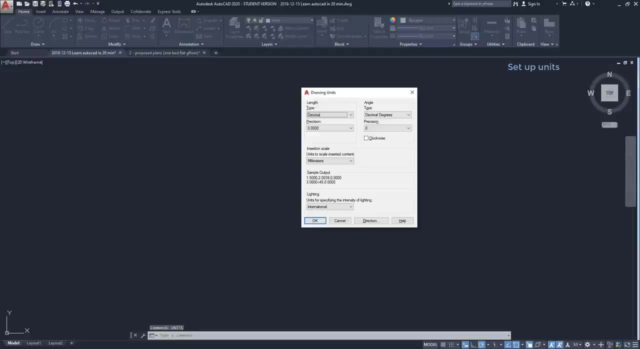 Now let's go to the unit properties window. I type units and press enter. Here on the length section at the left, you can choose the format for units of measure. If you work in millimeters or meters, you should use decimal units. 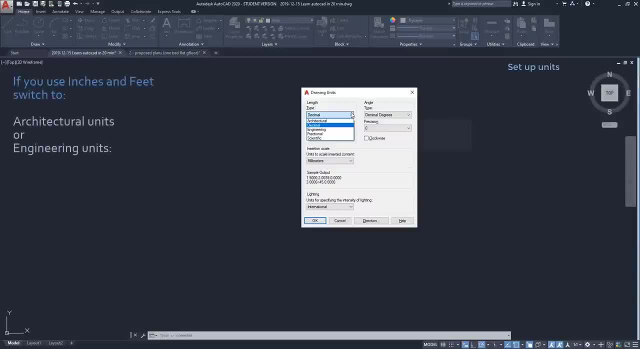 Instead, in some countries it's more common to use inches and feet. In this case, engineering or architectural units are more suitable. Below you can set the precision In this drawing. I consider the units millimeters and I don't need decimals. 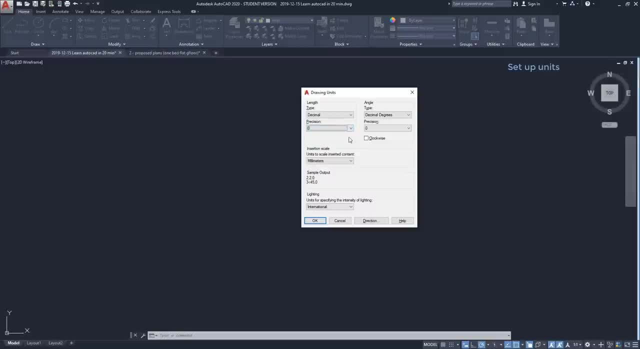 So I choose the first option. At the angle side I can choose the units for angles. Most of the time I use decimal degrees, But there are others here that could eventually be more suitable for you. The units in insertion scale are used only when I insert objects or drawings from a different file. 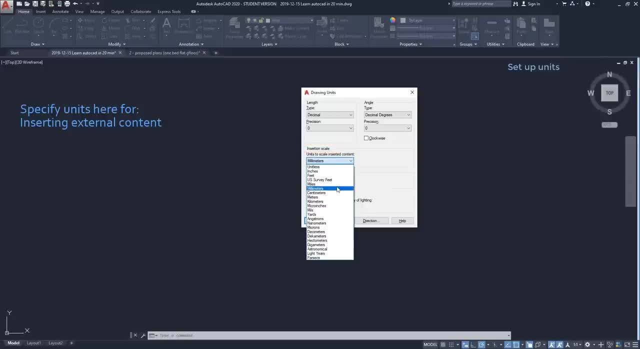 Usually, when we start learning AutoCAD, I don't need to insert anything external, But in my opinion it's better to specify the unit. I click on millimeters. When I finish, I click on the unit. I click on OK to exit. 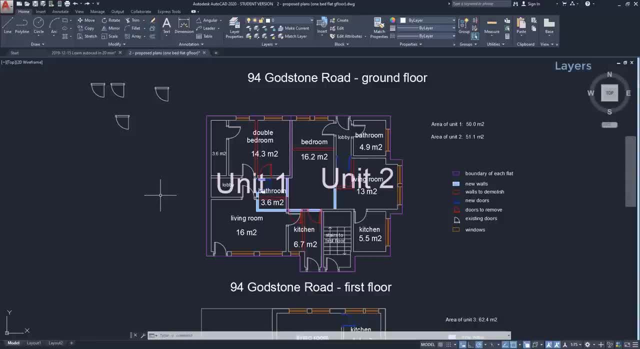 Layers. Layers is how AutoCAD organizes objects, For example. have a look to this file. Here I have two floor plans. It's a proposal for converting offices in flats, So instead of having the objects all together, I decided to organize them in different layers. 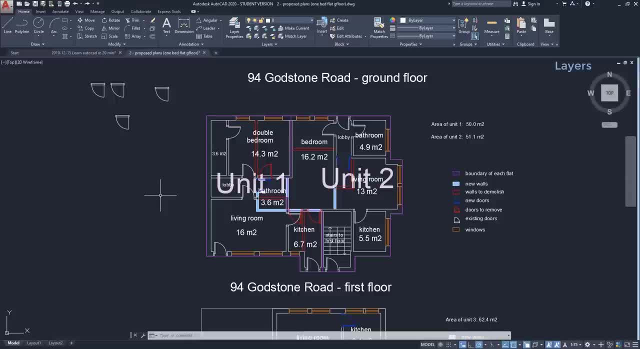 So, instead of having the objects all together, I decided to organize them in different layers. So, instead of having the objects all together, I decided to organize them in different layers. I am going to click on this icon to open the Layer Properties Manager. 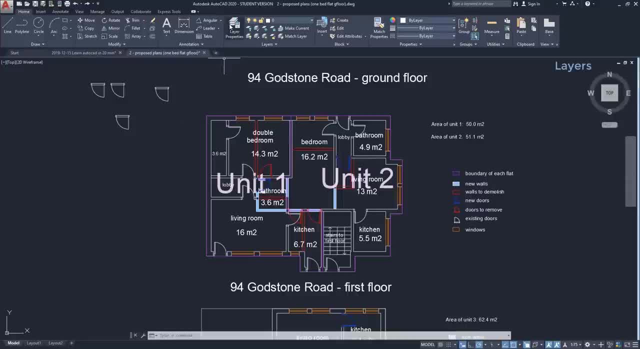 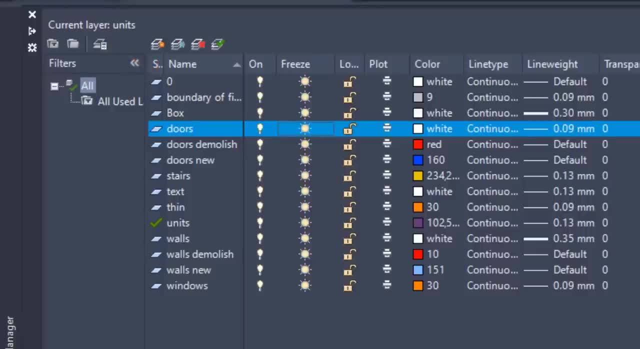 For example, I placed the windows in one layer, the walls in another, and I did the same for the doors, text labels and so on. In any project, I recommend to you to keep this layer without objects that are cool. You cannot rename it or delete it. 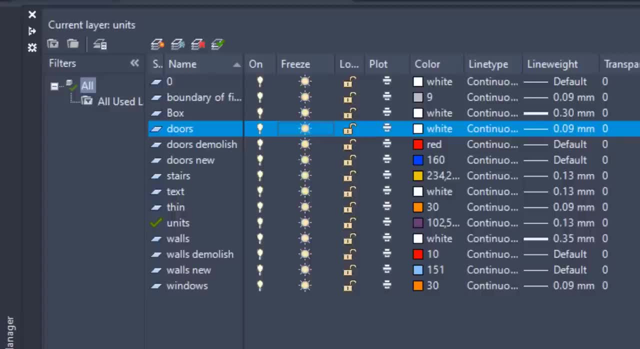 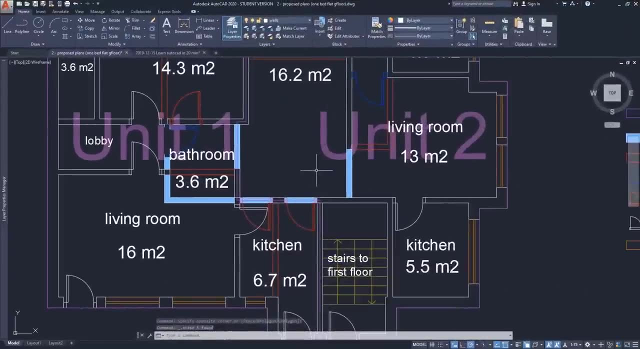 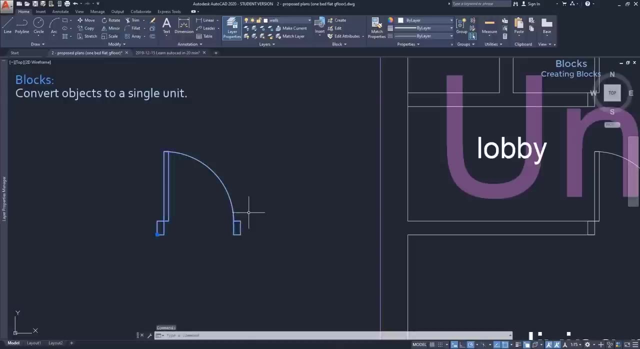 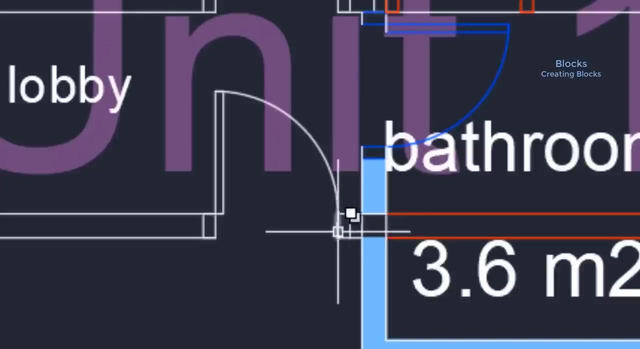 However, this layer can be useful for creating blocks, which is what I'm going to explain in the next section of this video. Sometimes we draw something that's easier if it would be a single unit, For example, a door. If we want to copy it, I have to select all the objects that compound the door. 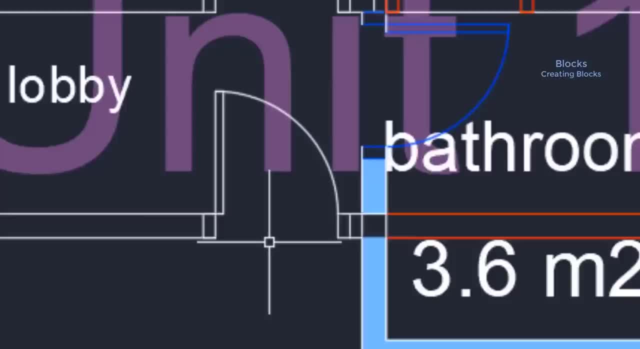 If we convert all these objects to a block, they act like a single object. So I want to convert this door to a block, As it's on the floor plan, to be easier to select it. I'm going to isolate the layer where the objects are located in. 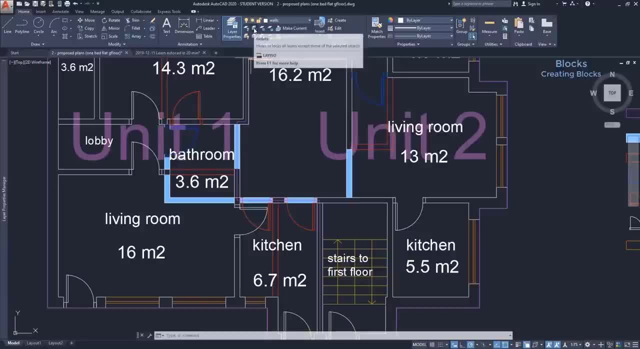 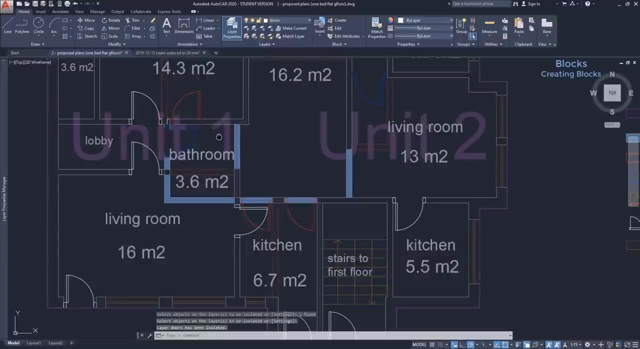 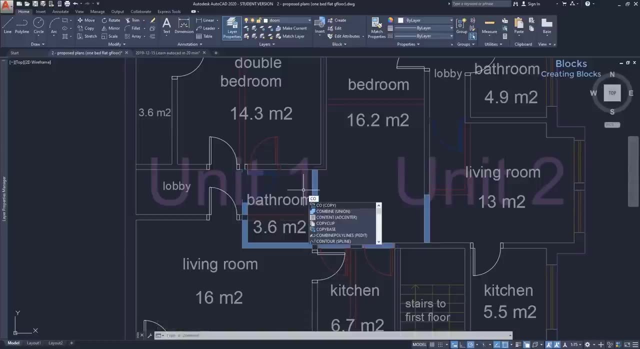 Click on the icon Isolate and click on any object of the door. Press Enter And the layer doors became isolated. Let's use the command Copy. Now it's very easy to select only the door with the selection area. That's because all the other layers are locked. 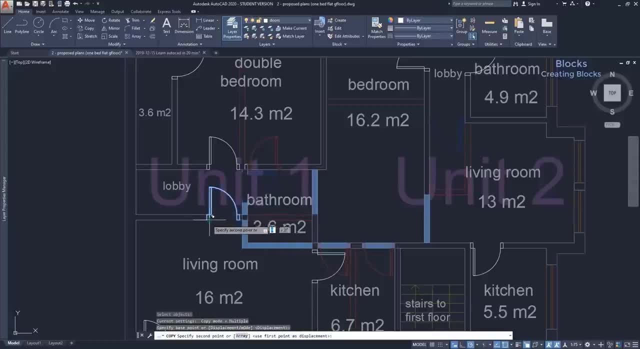 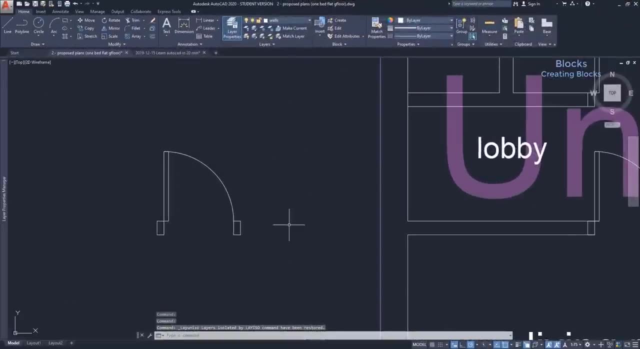 Press Enter and I can copy the door outside the plan Creating a block. Before creating a block, I'm going to move these objects to the layer 0. By doing that, I can later move the block to the layer I desire and it gets its properties. 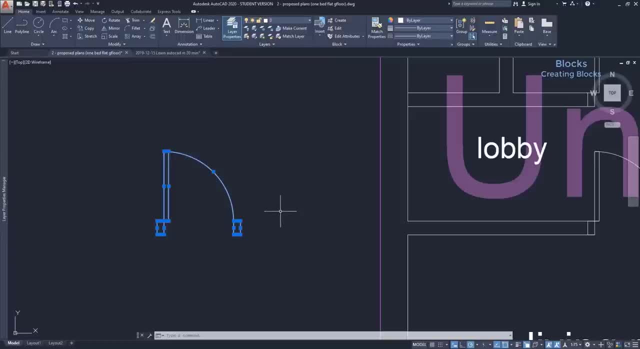 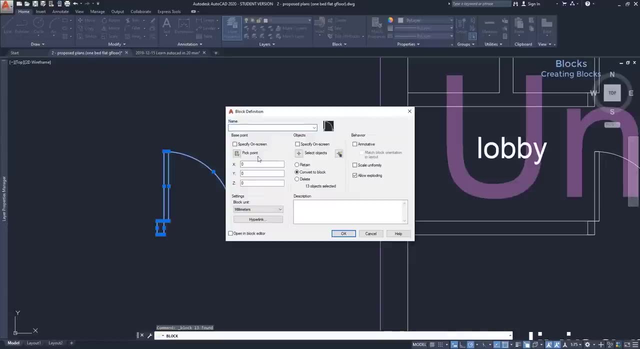 I select the objects and I'm going to click on the icon Create a block. The block definition window appears Here. I can set up a base point for the door. I choose this corner here. Back to the window. I have to write a name for the block. 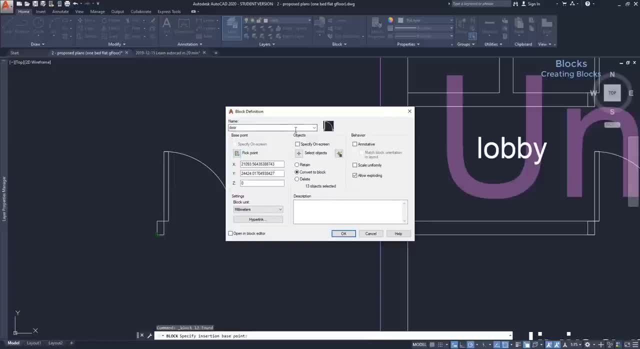 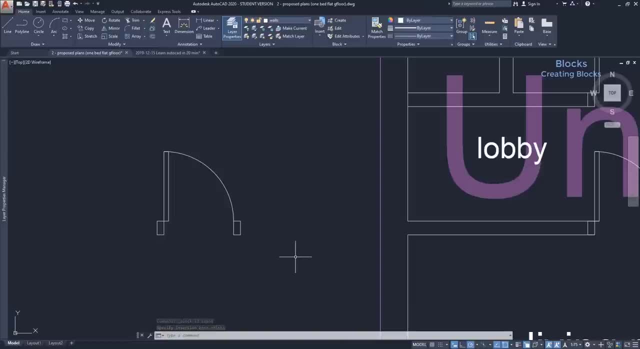 I name it as Door. When I finish, I click on OK. So the block is created. If I click on any part of the door, you can see that this is now a single object. Now I'm going to change the block to the layer that I want. 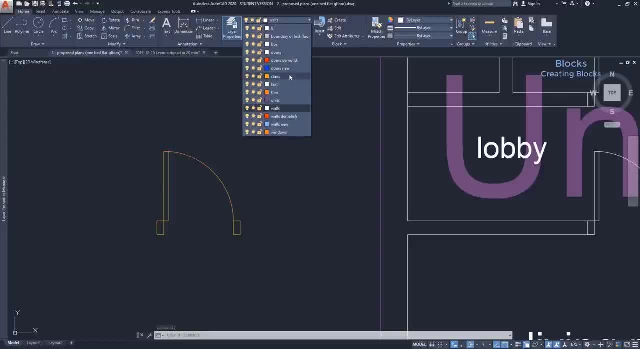 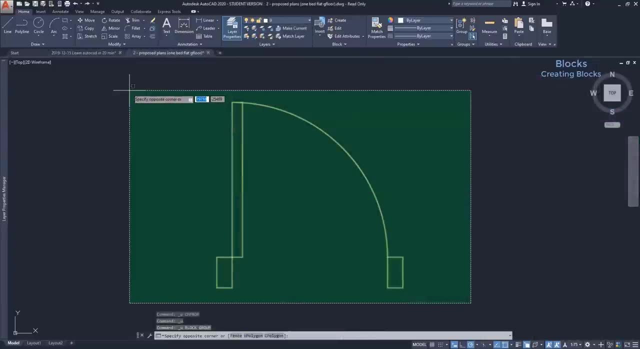 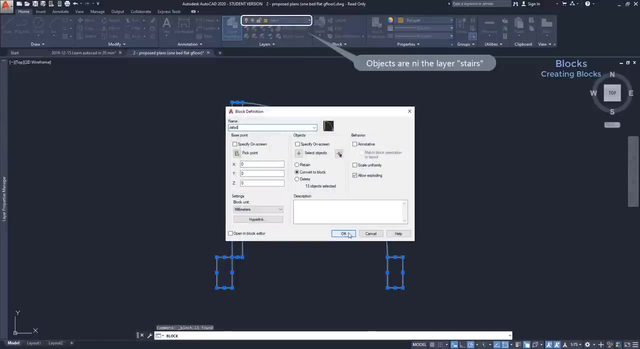 And you can see while I'm scrolling here- it changes the color to match the new layer. However, if I created the block with objects in another layer, for example stairs, I'm going to create the block. Then I'm going to change the layer of the block to another one. 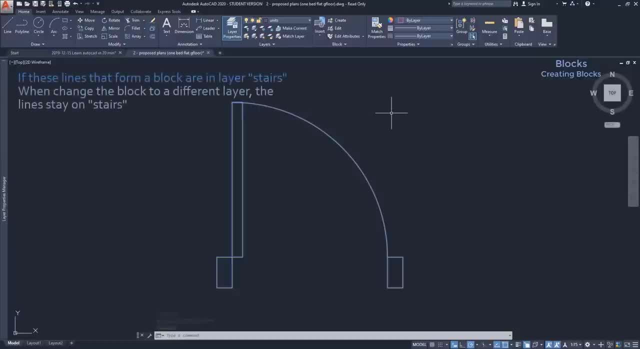 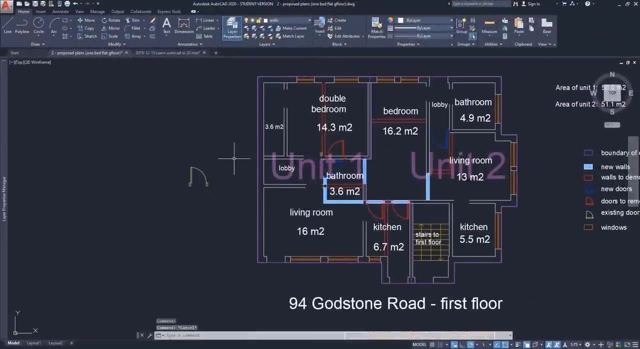 But it keeps the properties of the layer stairs. The layer 0,, on the other hand, means that the objects don't have any layer assigned. Check out this example: Add doors to the floor plan. As you know, I have my new block here. 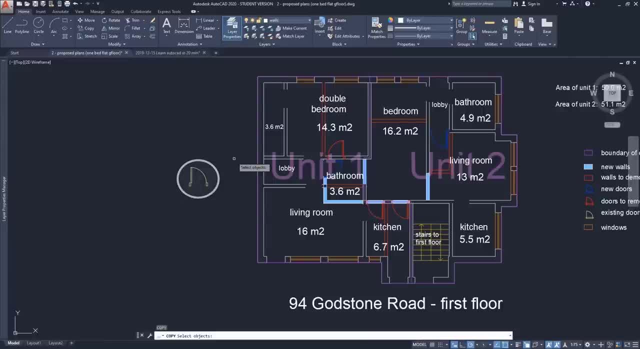 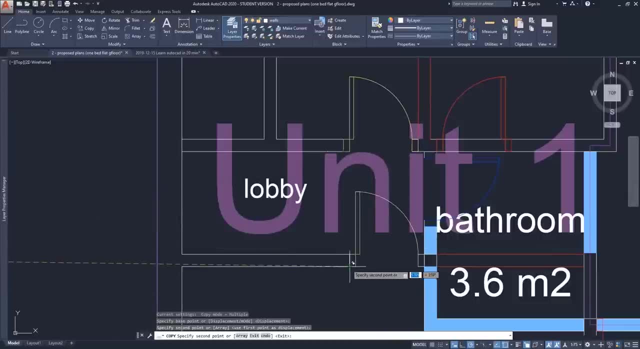 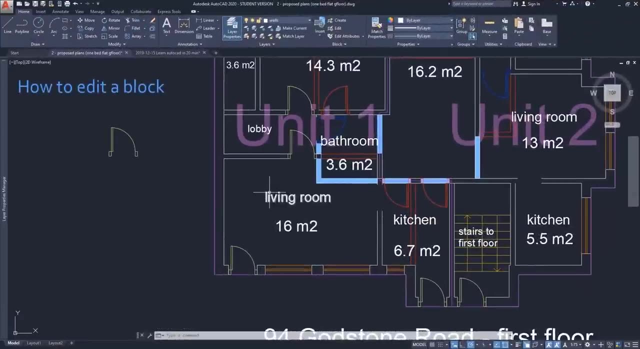 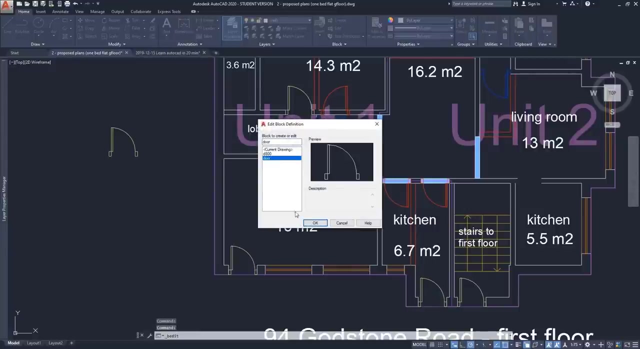 With the command copy, I can insert them easily in the floor plan. I just have to click on the endpoints of these lines. A great advantage of using blocks is the ease of modifying them. I go to this button that says edit block. Then I choose the block door. 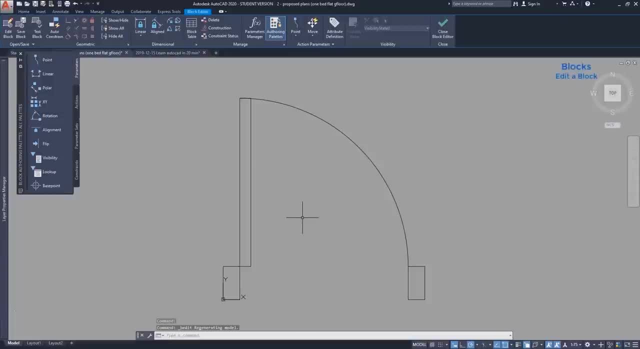 I click on OK. This is the block editor workspace, And also a new tab for editing blocks appeared on the ribbon. Here I can make all the changes that I want to this block. For example, I'm going to draw a circle here. 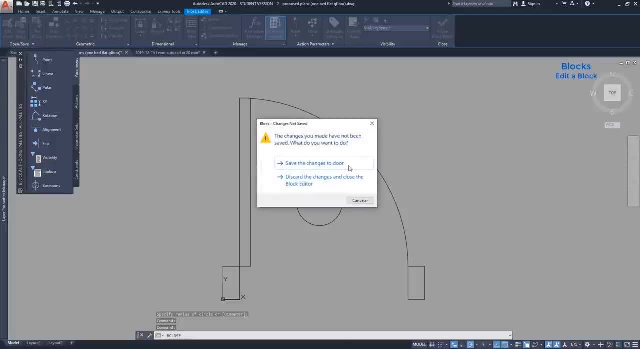 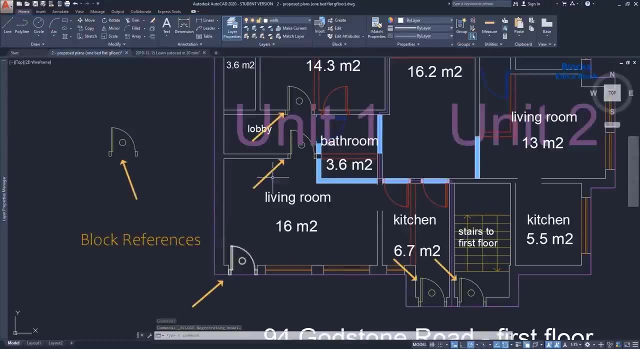 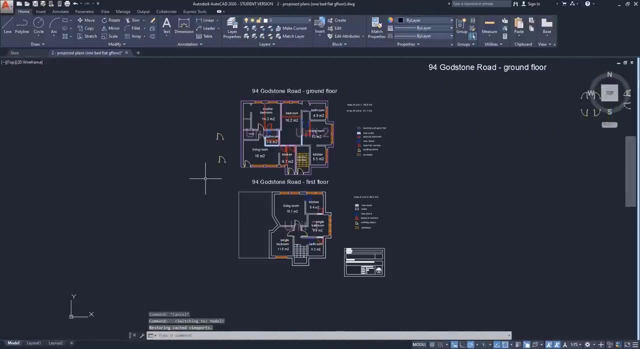 Then I close the block editor and save the changes. As you can see, all the block references of the block door have a circle inside, Which can save amounts of time. In this section I'm going to explain how you can print in AutoCAD. 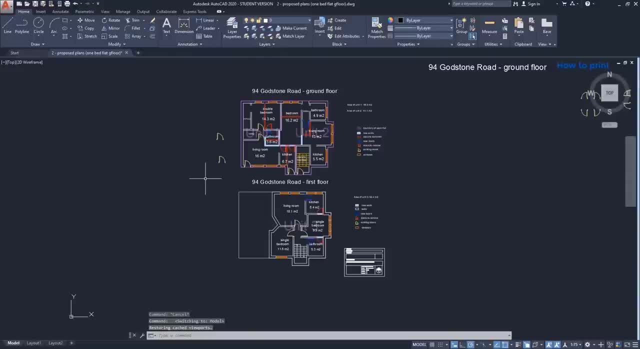 I know that a lot of people struggle with this topic as it's a bit complex, But I will explain the most important part To make it as simple as possible. First of all, look at the tabs located here. The first one that says model is where we can make all the project. 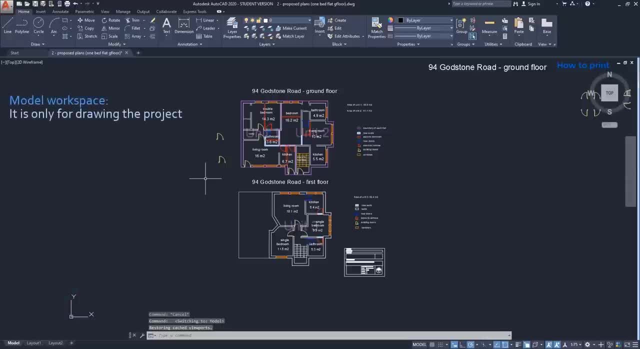 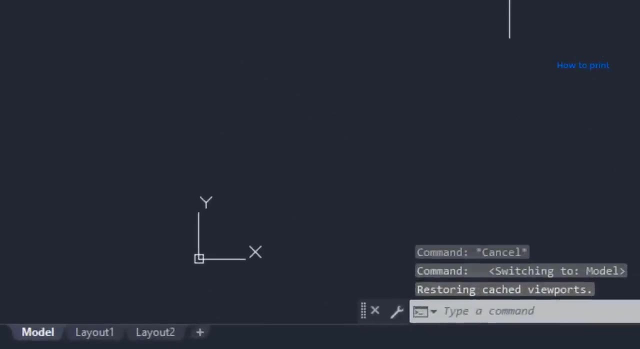 This workspace seems to have an infinite area, So we can make the drawings that we want, But of course, the larger the file, the slower the computer gets. The tabs that say layout are used for printing. I'm going to layout 1.. 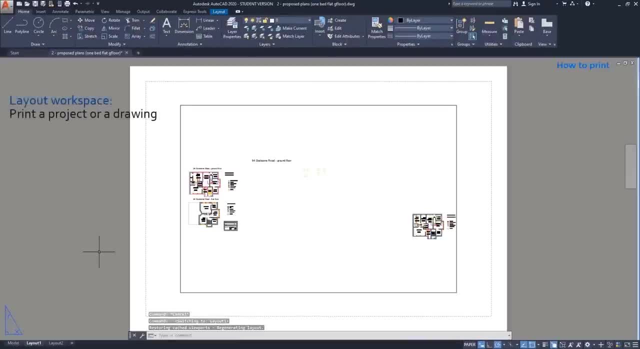 Here there is a paper with a specific size And these drawings is what it would be printed. To print properly, we should specify the paper size that we need. I'm going to click here with the right button And then click on Page Setup Manager. 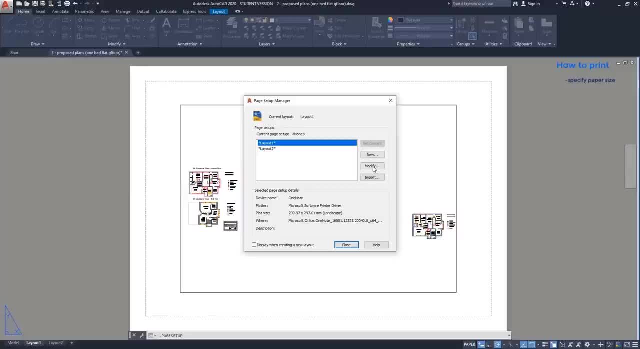 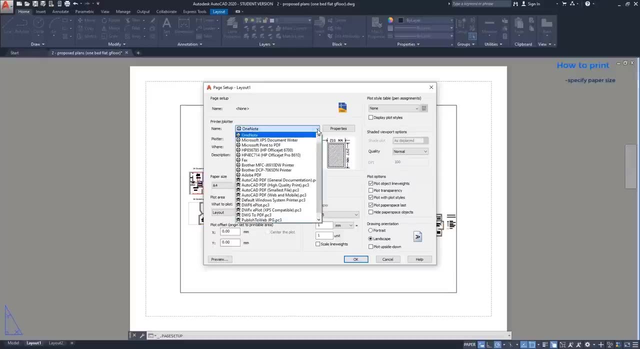 In this window, I choose Layout 1 and click on Modify. So here you have the page setup. First we should choose the printer by clicking on this tab If we want to save a page in PDF. there are several options here regarding the file size and print quality. 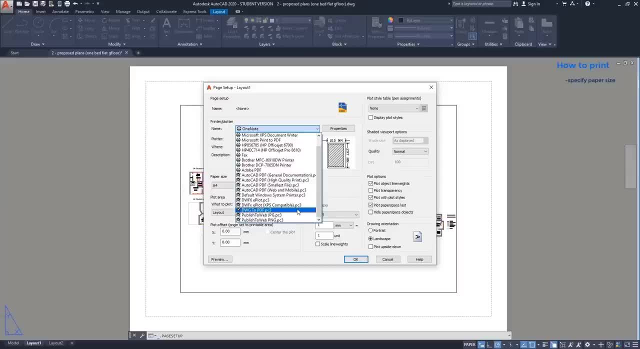 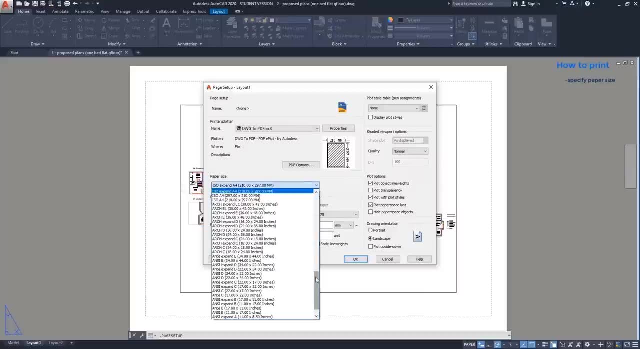 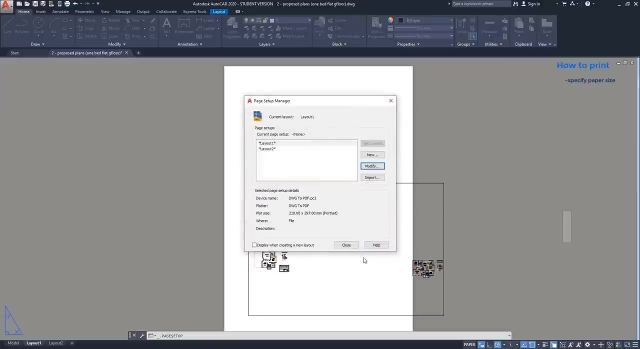 I usually use this one DWG to PDF To change the paper size. I have to click on this tab. For this case, I want A4.. This one On Drawing Orientation. I choose between Landscape and Portrait. Finally, click OK and close to save changes. 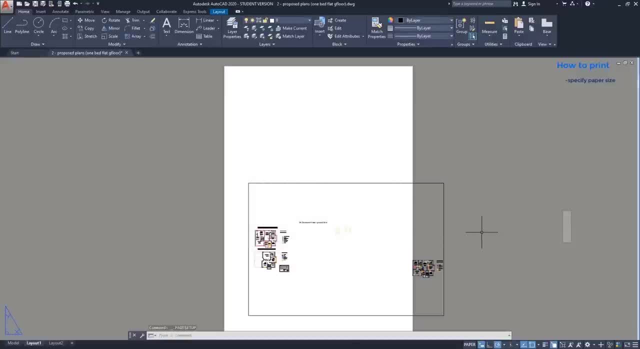 Now that we have the paper size, we have to decide what we want to print on there. On the Layout tabs there are two spaces: Paper and Model Space. We can switch between them here. Currently we are in the paper space. 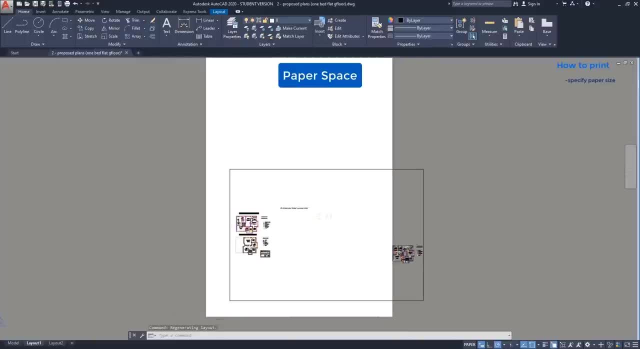 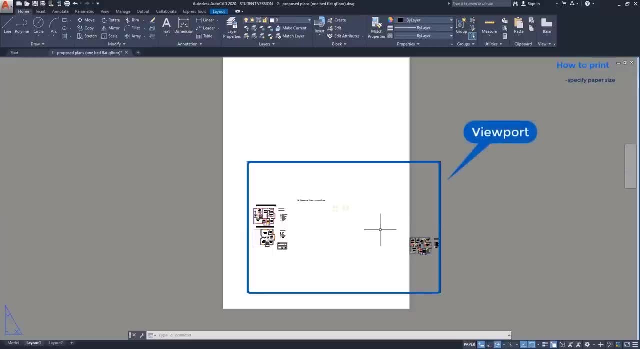 If I apply zoom or move, it works for the paper. Notice this rectangle here where I have the drawings. It's a viewport and it's like an access to the project. I am going to double click inside and it switches to the model space. 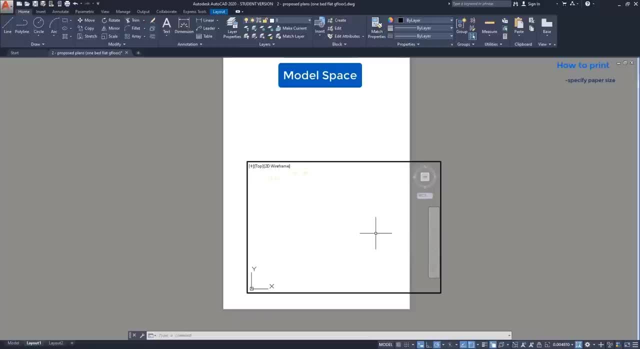 Now, if I zoom, the paper doesn't move, just the objects that I drew As well. if I draw a line here, it will appear exactly in the same place in the Model tab. Change the size of the viewport. I am going to click on Model. 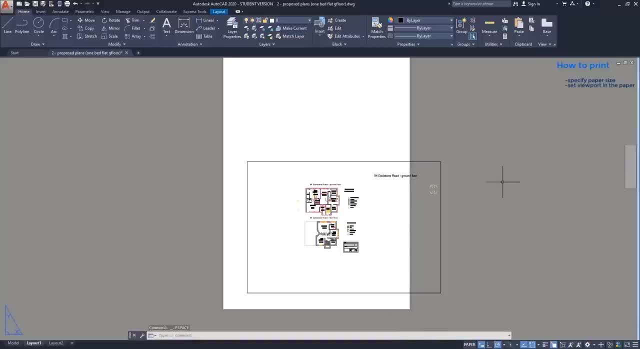 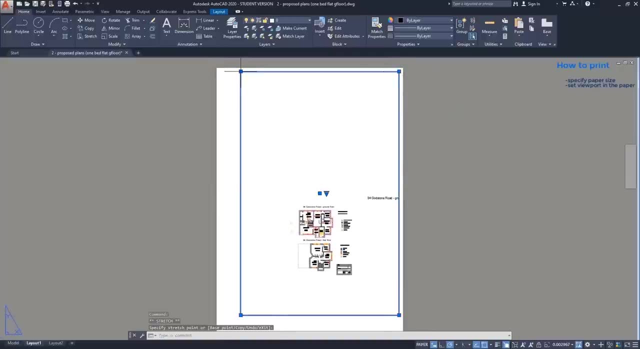 to switch to the paper space again. At this moment I can select the viewport. Then with the grips I can modify it to cover the entire paper. Double click to go to the model space. Now I can zoom in the drawing. 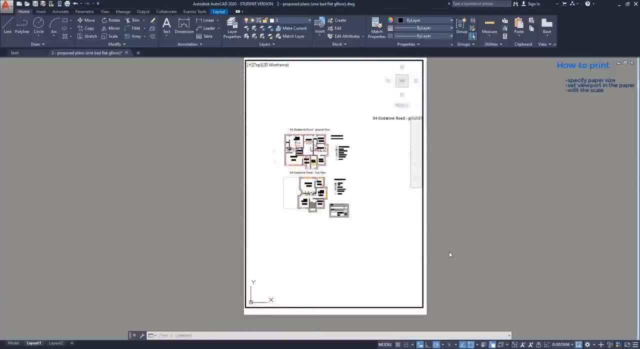 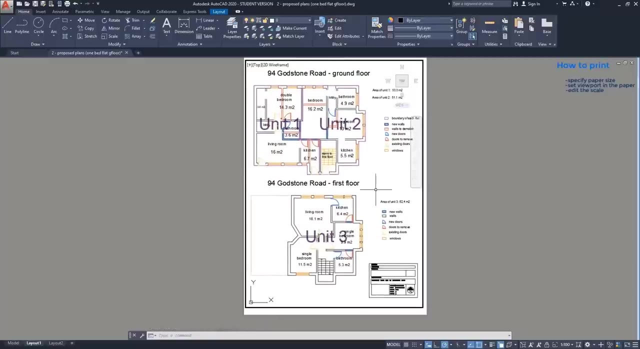 or put a specific scale for the paper It's. here I specify, for example, 1 per 100.. When I finish, I am able to print the drawing. I click here with the right button and this time I click on Plot. 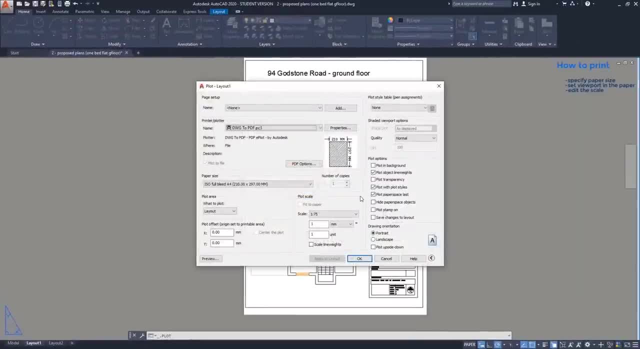 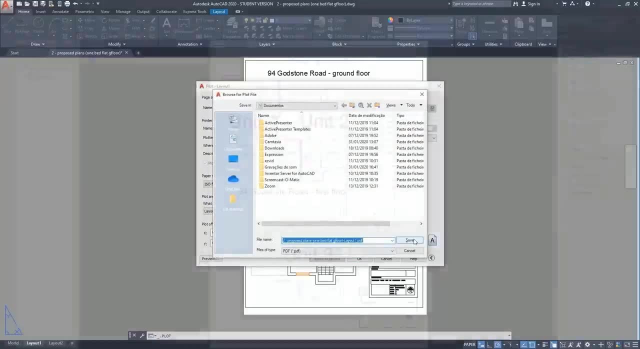 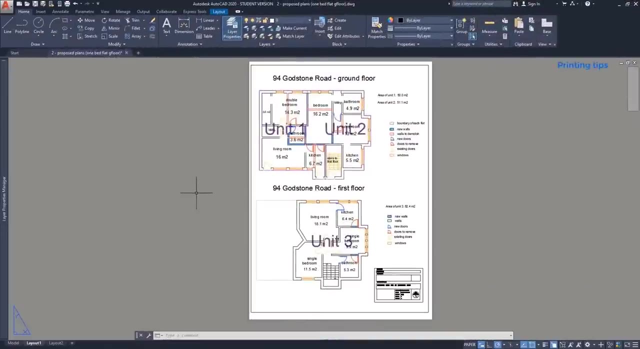 Continue to plot a single sheet. Here I can click on OK to print or, in this case, to export the file as a PDF. Some printing tips Hide the viewport. When I plot a file, the viewport appears by default on the paper. 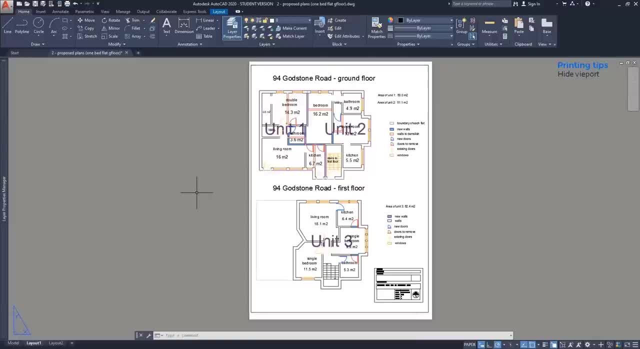 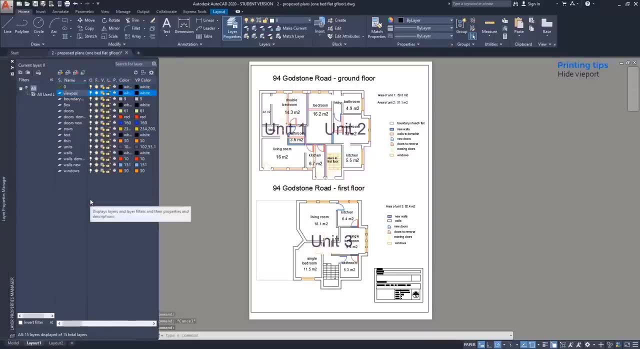 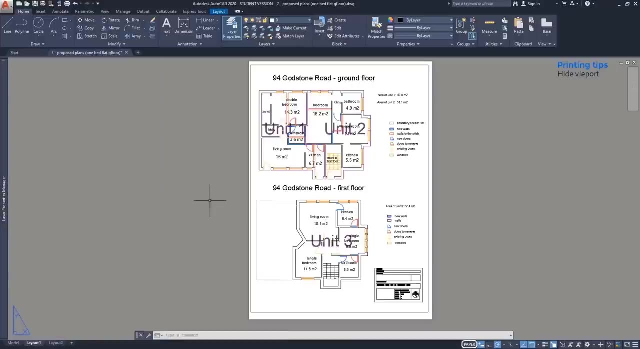 If you want to hide it, follow the next steps: Go to the Layer Properties Manager and create a new layer just for the viewport. Switch to the paper mode. Click on the viewport and move it to its own layer. Then go again to the Layer Properties. 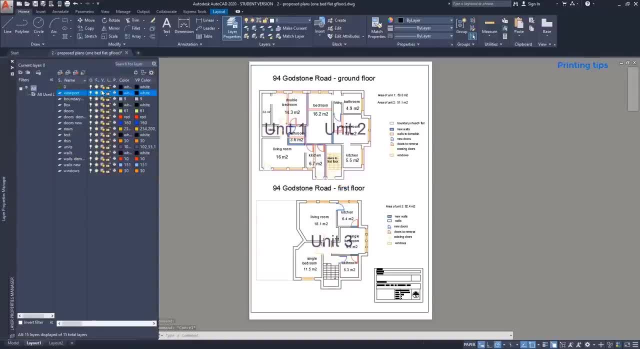 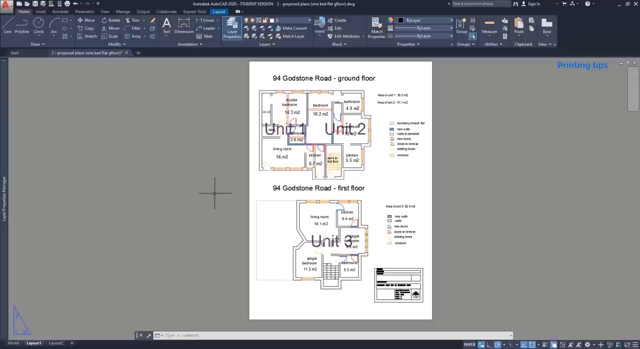 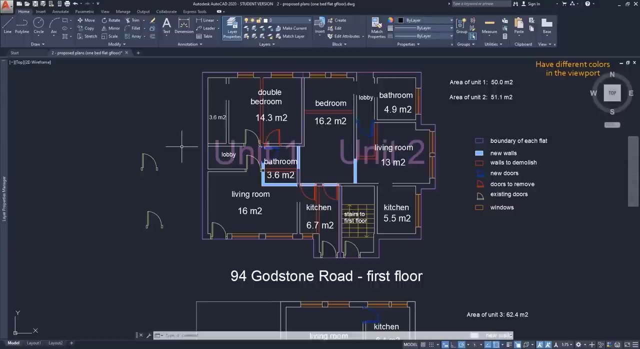 and freeze the layer, You can see that it's not appearing anymore. So if you save as a PDF or print a file, right now the viewport is not visible. Have different colors on the viewport. The default AutoCAD workspace uses a dark background. 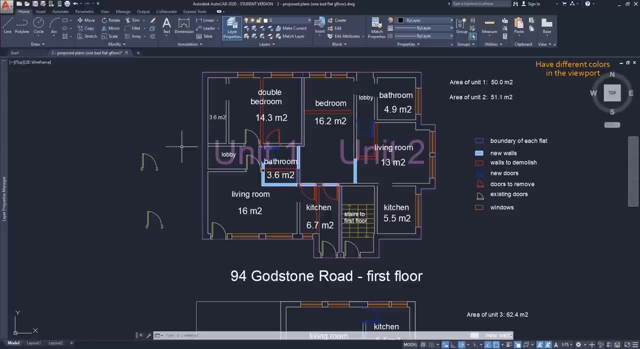 with the reason to be better for the eyes when working for several hours. Because of that, it's common to use light colors in our project. The problem is when we switch to the layout mode, the colors can be too light for a white paper. 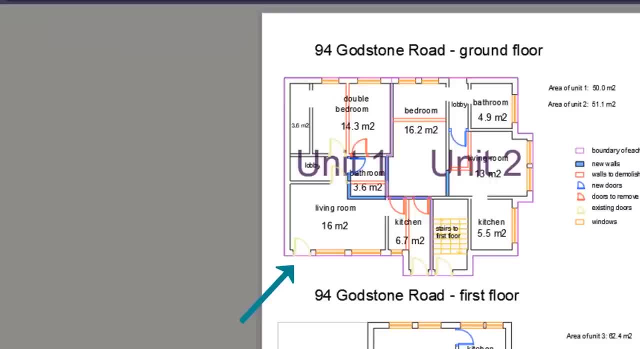 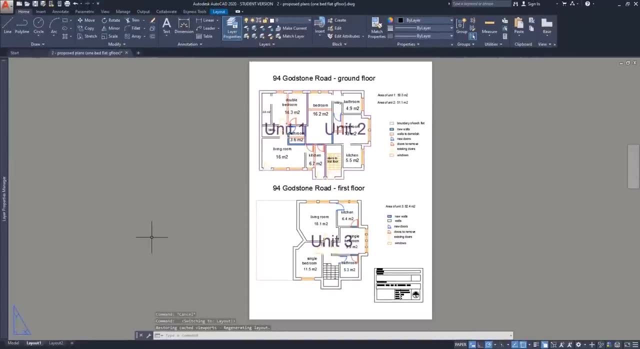 For example, the doors are a bit hard to see. Don't worry, It's possible to set up different colors for printing. First you have to double-click on the viewport to switch to the model space, Go to the Layer Properties and you can see this column. 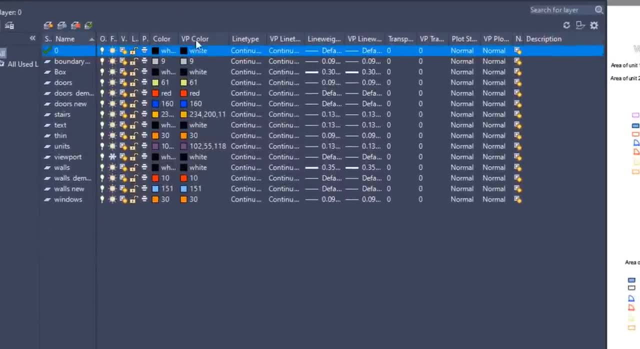 with the label VP Color. If in your version it's not located next to the Color tab, look at the right end of this table. Then I'm going to change the color for the layer doors. Click here and put this one. 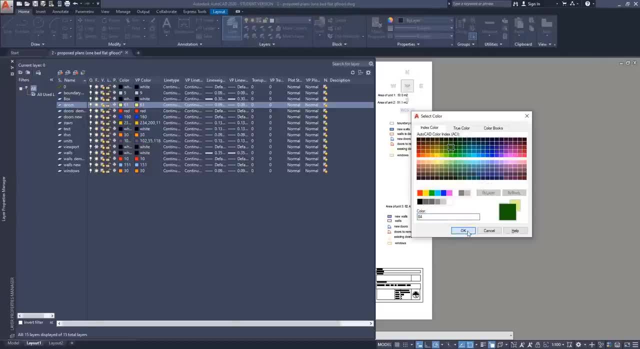 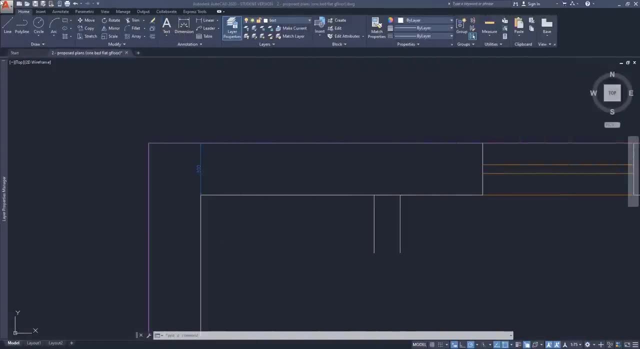 for example. Now it's much better Insert Text. I am going to explain to you quickly to insert text in AutoCAD. It's not hard and there are two types of text: single line and multi-line text. I will start with single line text. 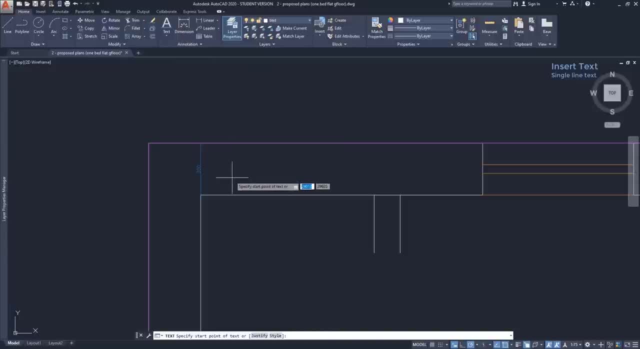 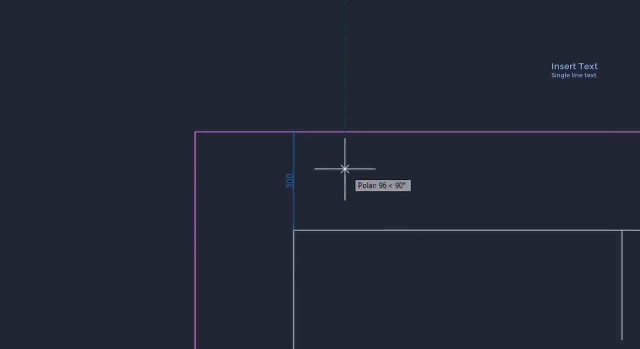 First we insert the start point, Then this line specifies our text height. I can either click or specify a distance. I'm going to type 100.. Press Enter and then I choose the direction If I want to type horizontal text. 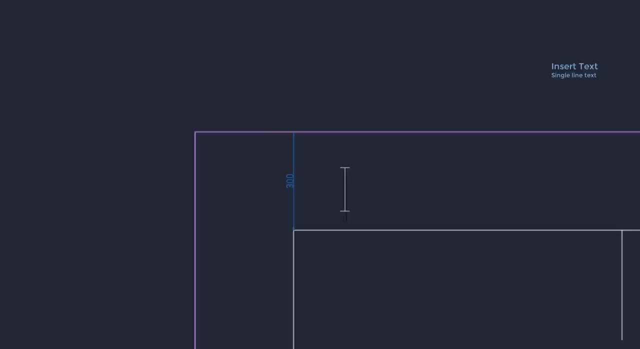 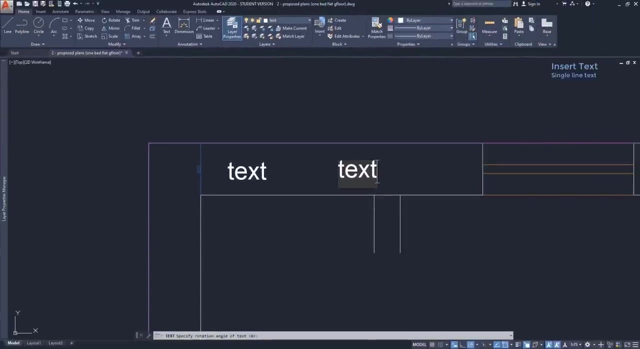 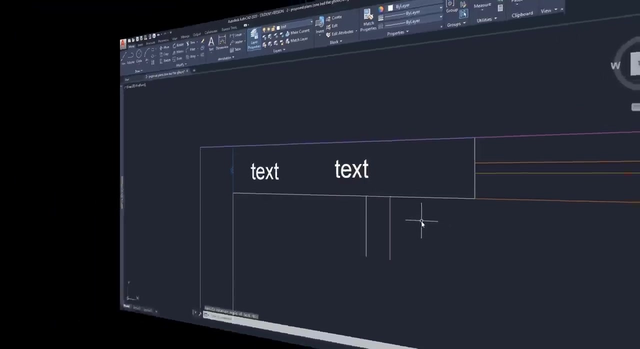 I need a horizontal line. Now I can write anything and when I finish I click in a different place to write another text. or if I don't want more, I can just press Enter or Escape. Now let's see the multi-line text. 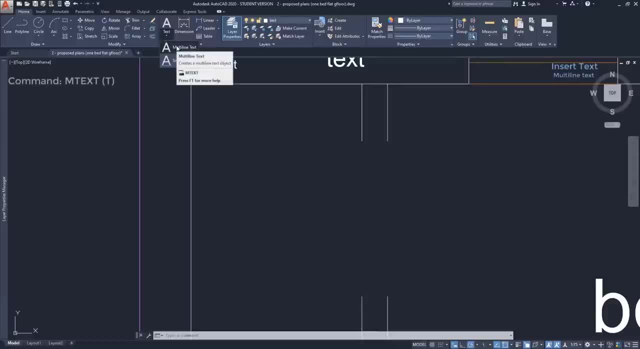 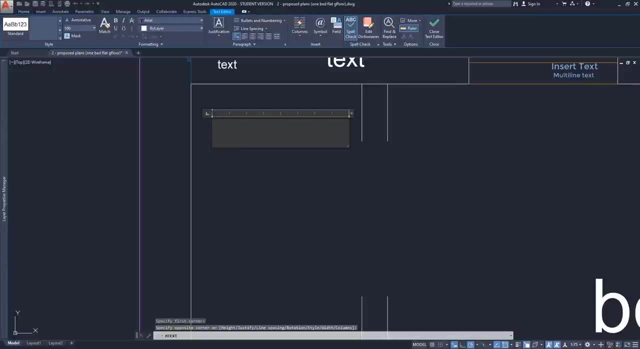 Activate the command, Choose first point and I specify a selection area to fit the text in, but just the horizontal length, The height of the rectangle doesn't matter. Then I can write the text. Unlike the single text, this time a temporary tab for editing text. 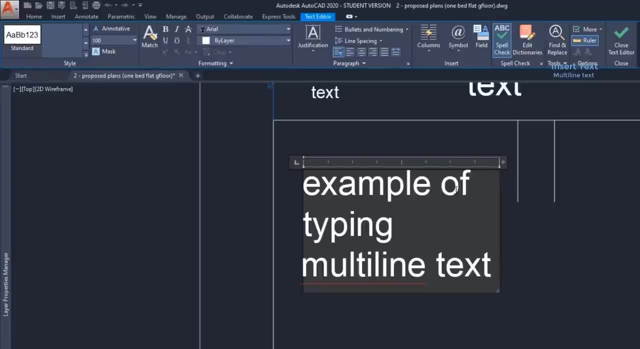 appears on the ribbon. Here I have options for editing a paragraph and much more. If I want to change the height, I need to select a text and change it here. As you know, this is very simple to write text in AutoCAD. 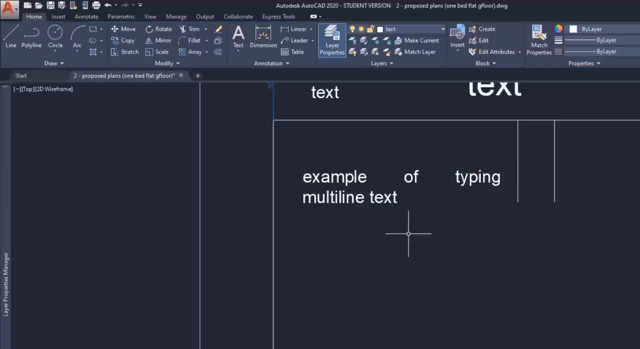 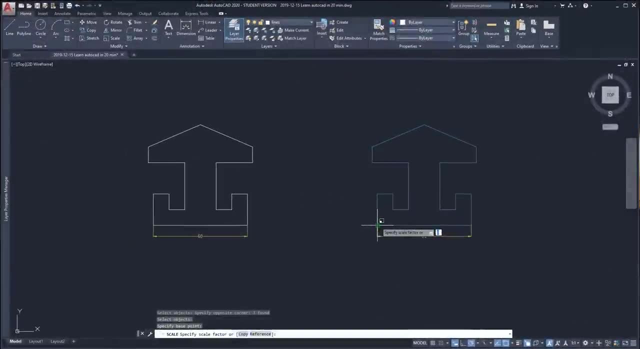 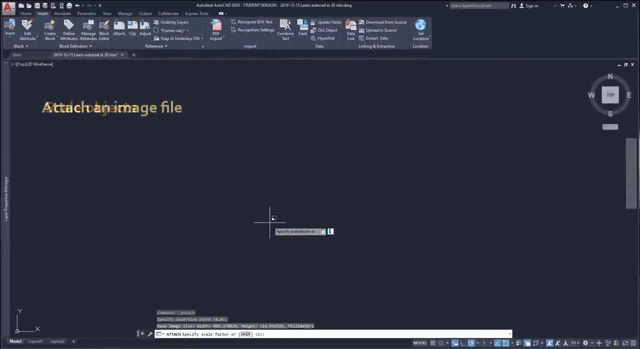 Part 4. In this part, I'm going to teach how to scale objects, how to attach an image to the image, how to add a text to the image, how to add a text to the drawing and apply scale in order to have the real dimensions. 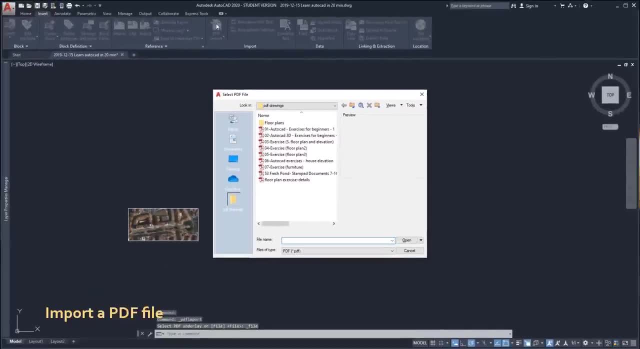 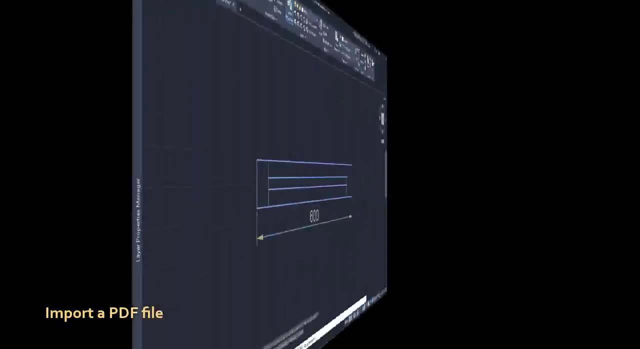 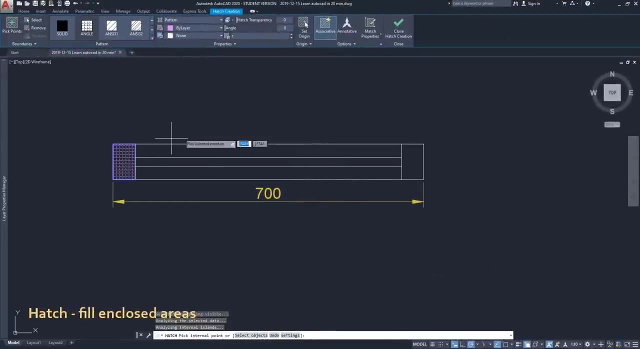 how to import a PDF file, and this is especially useful when the file was previously created within AutoCAD. how to stretch objects and how to fill enclosed areas with the command hatch. Of course, as always, I like to share some tips with you and the explanations. 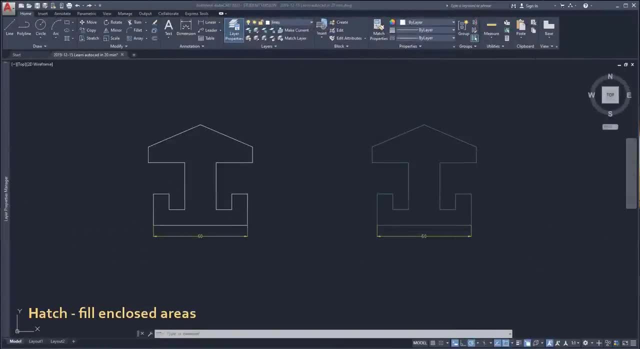 Let's start Scale objects. Let's learn how we can scale objects. This command is not hard, but you should understand it well if you want to use it properly. To turn on the command scale: click on the icon. It's this one. 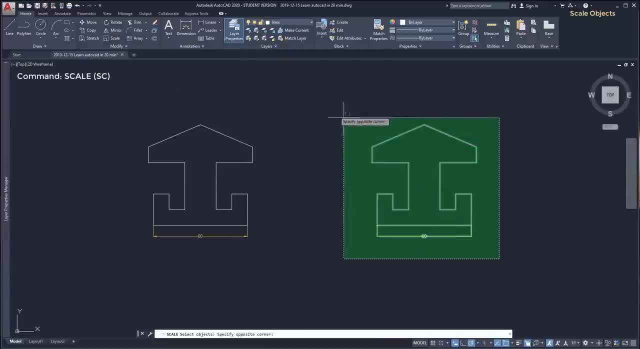 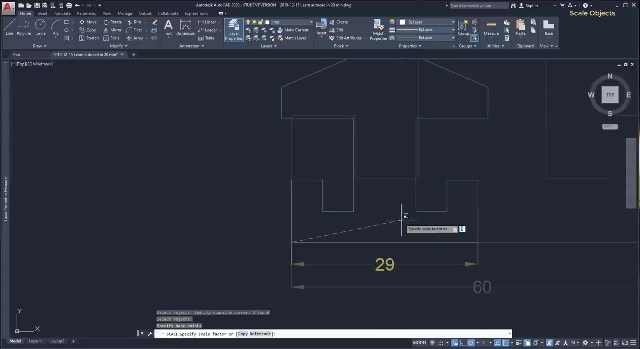 Select the objects I want to scale. In this case, I want to scale the figure on the right. Now there are several modes to scale objects. The one by default is to insert a scale factor. I am going to type 2 and the lengths. 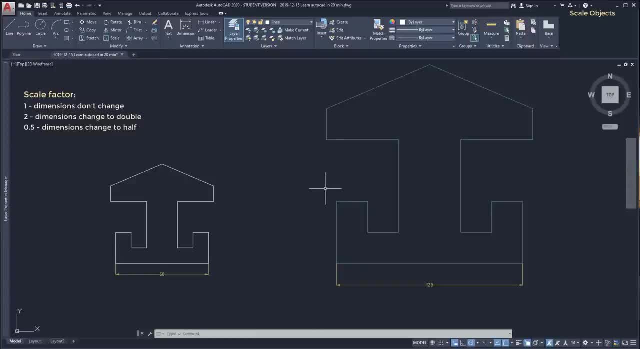 of all these lines change to double size. Ok, I am going to repeat the process, but this time I want to shrink the objects to half size. I type sc to activate the command again. Select the objects, but now I don't select the dimension line. 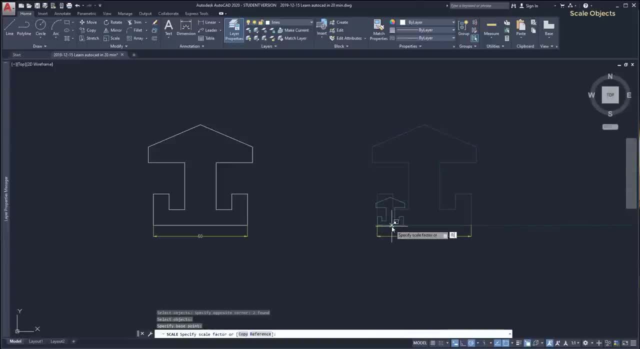 For the scale factor, I insert 0.5 and the lines were converted to half of the length that they used to have previously. Look that this dimension line was updated. even it was unselected Scale with a reference. Now I am going to show to you. 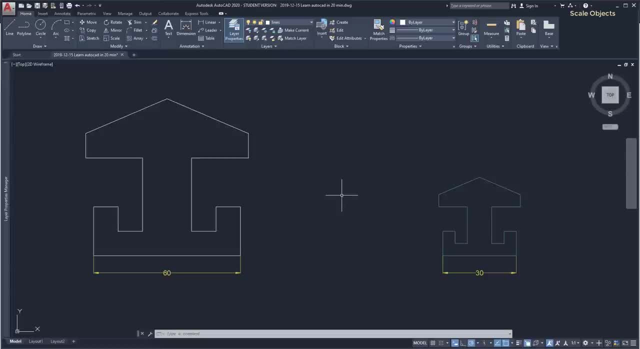 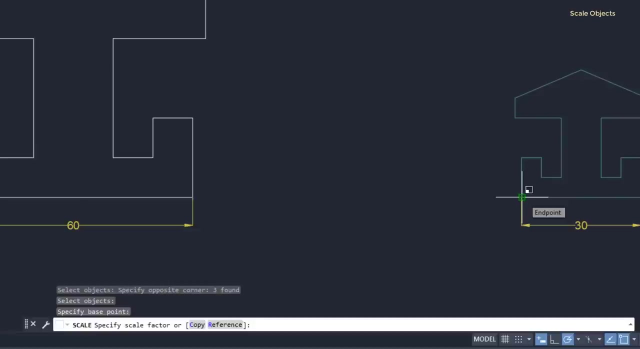 how to insert a scale with a reference. I turn on again the command scale and select the objects. Select the base point. Looking to the command bar, it says specify scale, factor or these options: copy and reference. I am going to use the shortcut R. 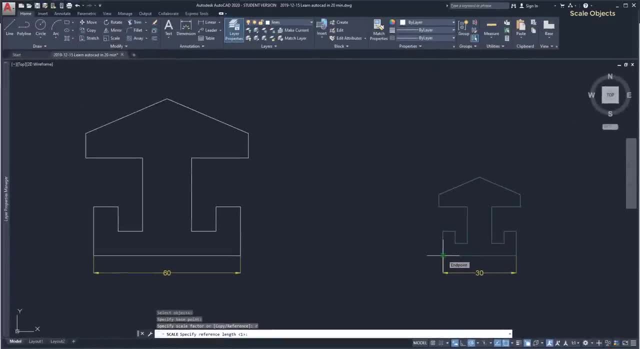 to use the reference, And what I need to do here is draw a reference line and type a new length for it. So it's very simple: I click for the first point and then I click for the second point. Finally, I type the new length. 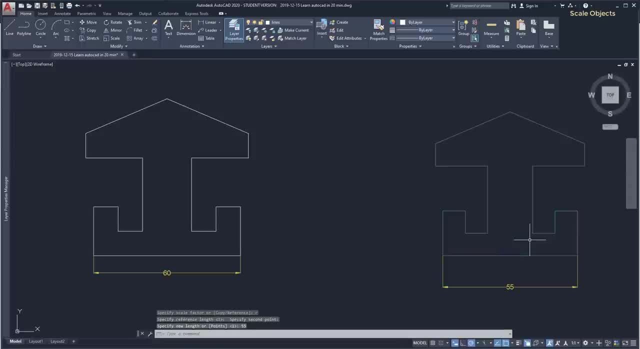 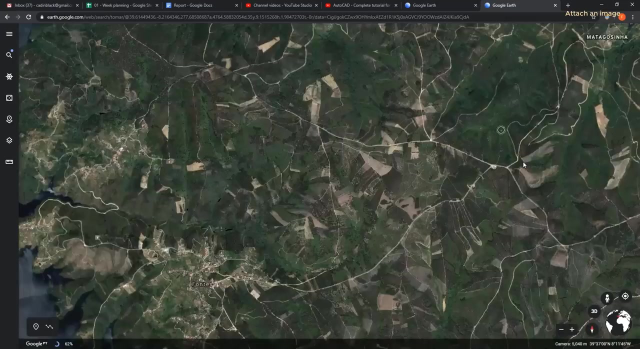 which is 55, and press enter to confirm it. Use scale to import a PDF or attach an image. In AutoCAD, it's possible to insert an image to use as a background of a project. For example, images from Google Earth can be used to draw. 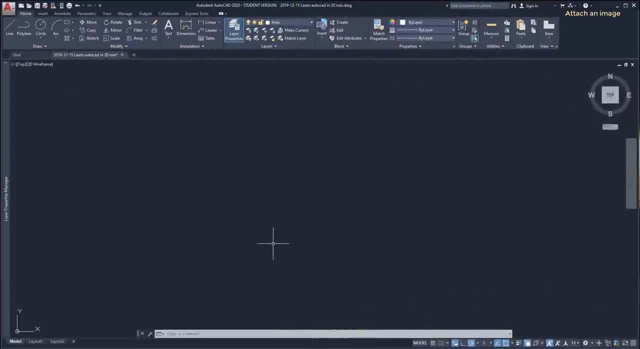 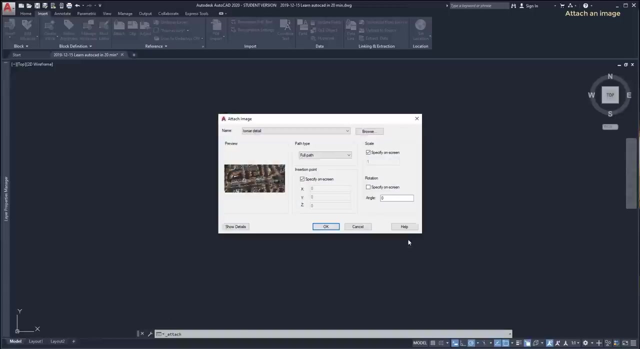 site plans To attach an image file. I go to the insert tab at the ribbon, click on attach and select an image from my computer. I choose this one In this window I can set few options Here. it's important that I tick on specify on screen. 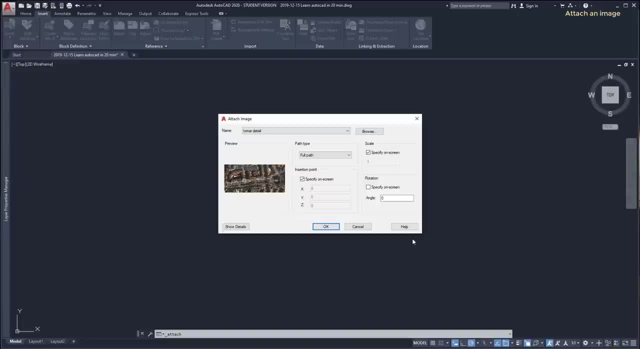 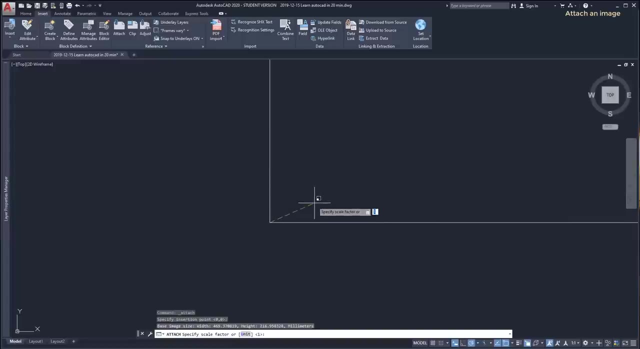 the insertion point. Otherwise the image is inserted on the coordinates which are specified here. Ok, except if it's exactly what you want, I click on ok. and now I click for placing the image And for the scale factor. I leave it for now. 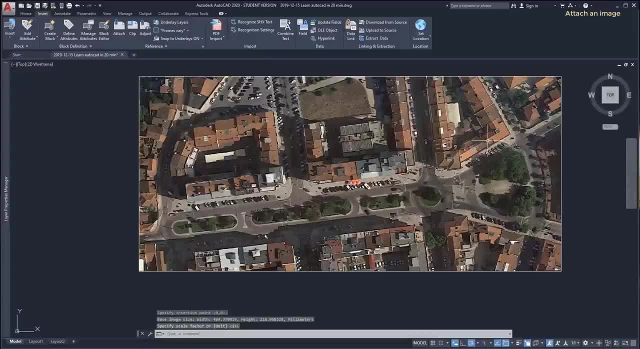 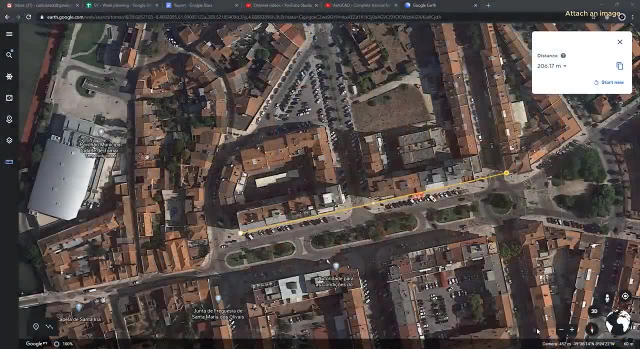 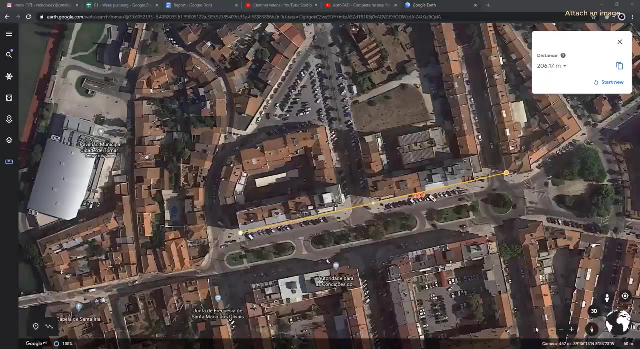 Press enter. So what happens here? Most of the time that we insert an image, it's not scaled properly. For example, I have a reference between these two points which is approximately 206.17 meters. If I use the distance command, I type DI. 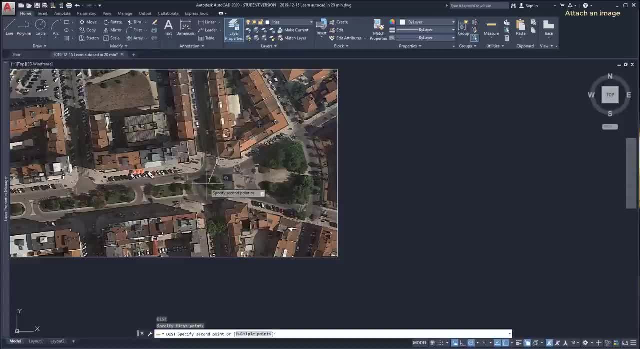 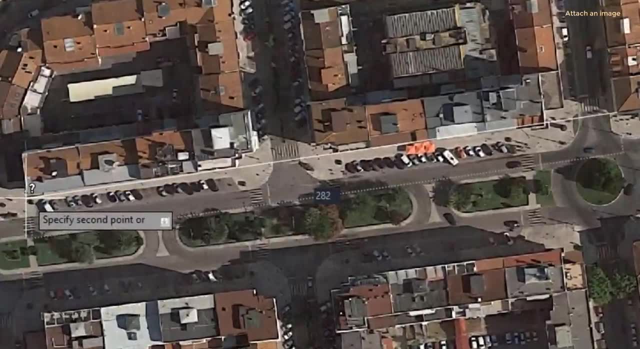 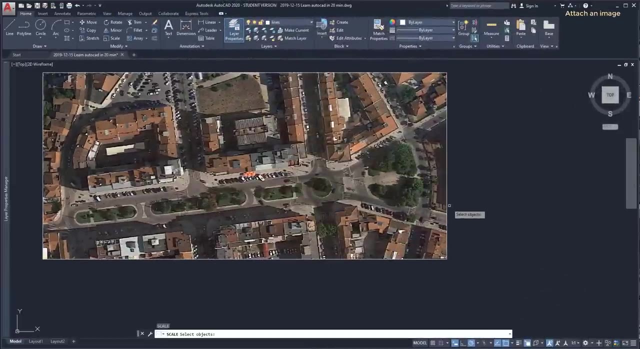 press enter. I can notice that the distance here is a bit longer than what it should. No problem, I can use scale with reference. I turn on the command and scale. Select the image by clicking on the border. If I click inside the image. 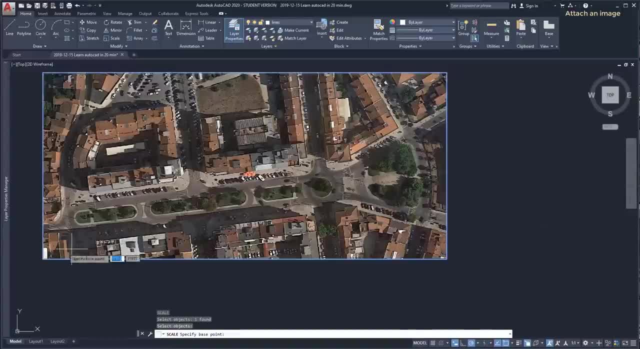 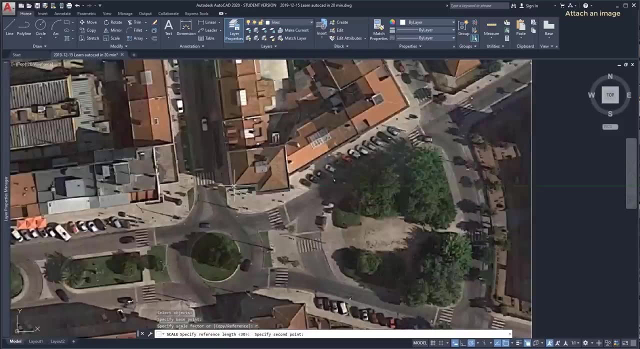 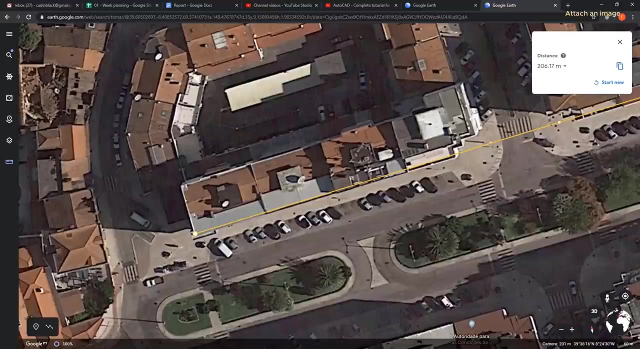 it doesn't work, Change the mode to reference, and then I draw the line between those two points. I will try to make it as accurate as possible. Now it should be correct. Ah, and I want to share a tip with you. Always try to use. 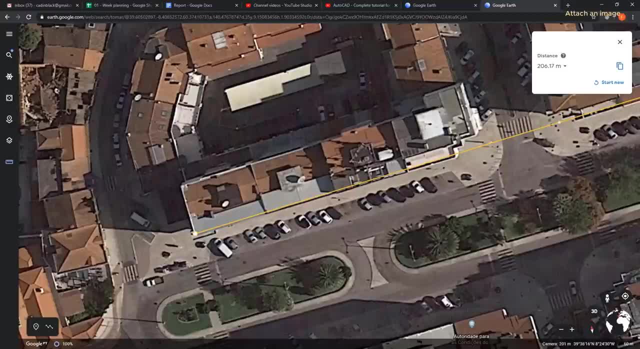 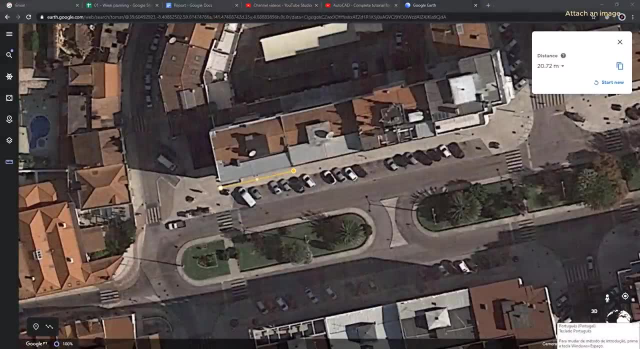 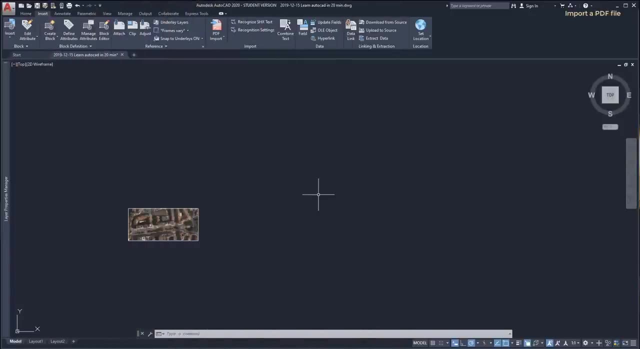 a long reference line because if, instead, my reference was a short distance, after scaling, the image tends to be less accurate. To import a PDF file, I can click on the icon also located on the insert tab. here I'm going to choose the file of the exercises. 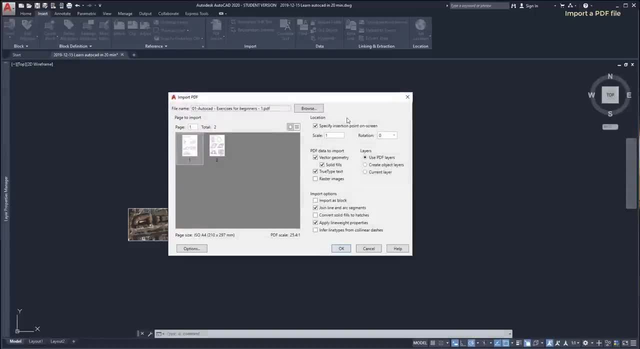 Then the window that opens has a bit more complex options than for attaching images. Actually, this is a very useful function because if I insert a PDF that was previously created in AutoCAD, I can recover all the layers and the objects, As this PDF has two pages. 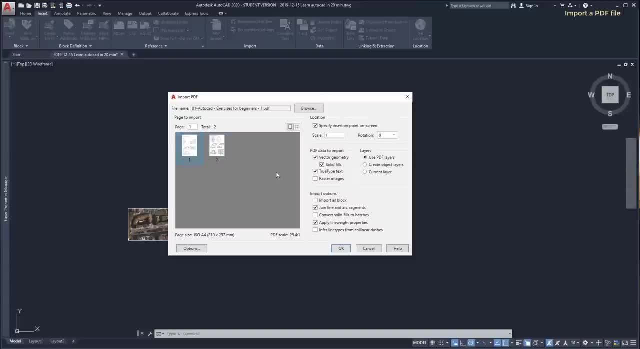 first I need to click on the one that I want to import. On PDF data to import, I tick on vector geometry to import the lines, polylines, circles, arcs and so on. If I tick on true type text text created with a font that has this symbol. 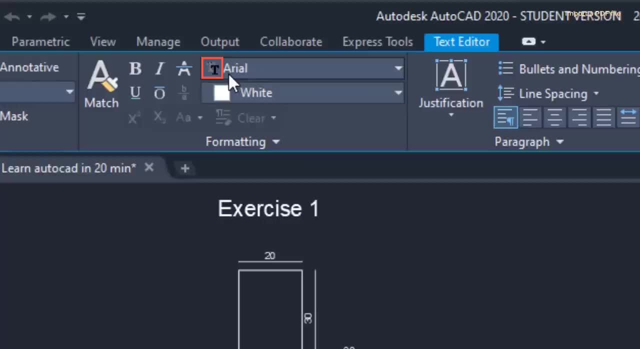 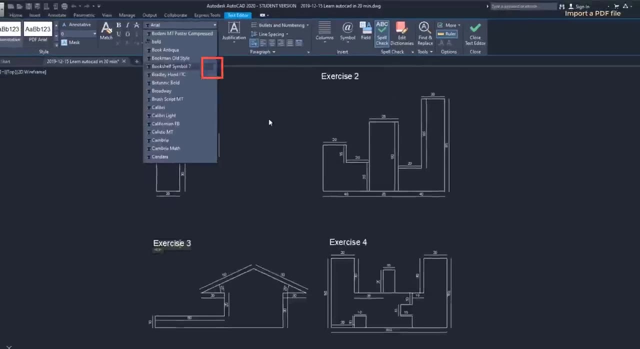 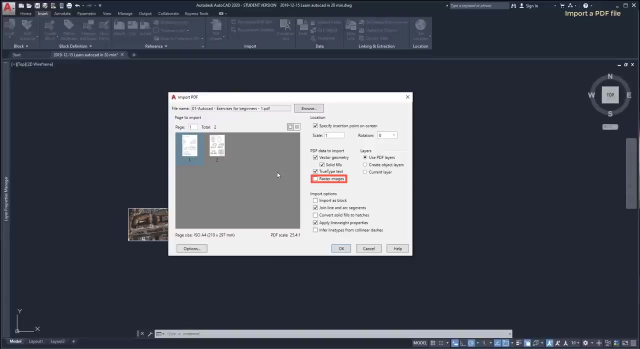 will be automatically recognized as text In AutoCAD. most fonts available are true type, so usually this is not a problem. The option below: I tick on it if I have raster images attached. in this case there aren't, so I keep it unselected. Then on the right panel. 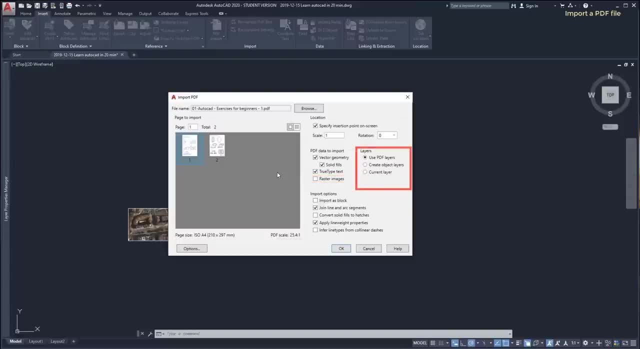 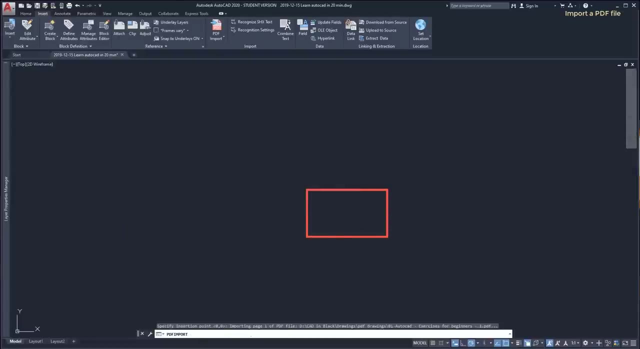 I tick on the first option: Use PDF layers. On the panel below you can find more options to add, but for now let's click on OK and I'm going to insert the file on the project Nice. Now, if I go to the layer properties, I can see that new layers. 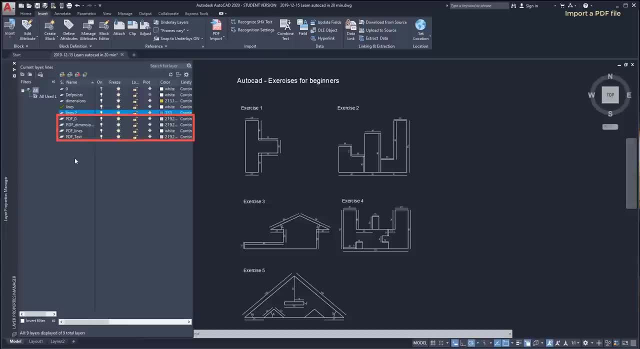 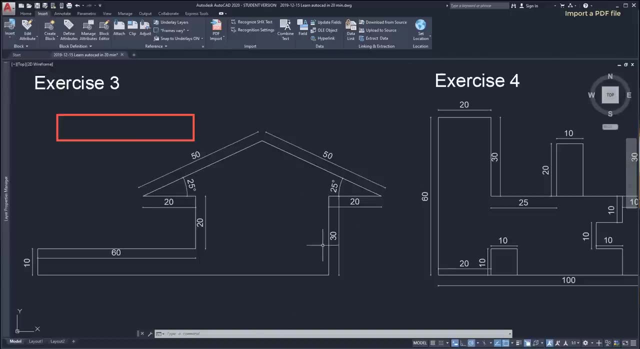 were created from the PDF and, due to the fact that I made this drawing in AutoCAD, the layers are the same from the original DWG file. I'm going to check out how the objects look like and you can see here polylines, among other objects. 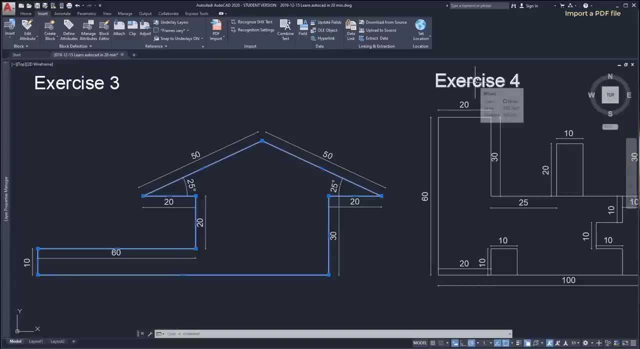 Also look how the text was recognized. if the text was not on a true type font, it would be splitted in very small lines and arcs, which wouldn't be so interesting. however, not everything is perfect. the dimension lines are not recognized, neither block references, which means I have to. 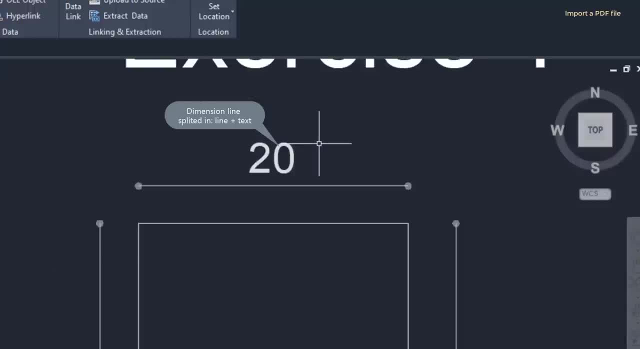 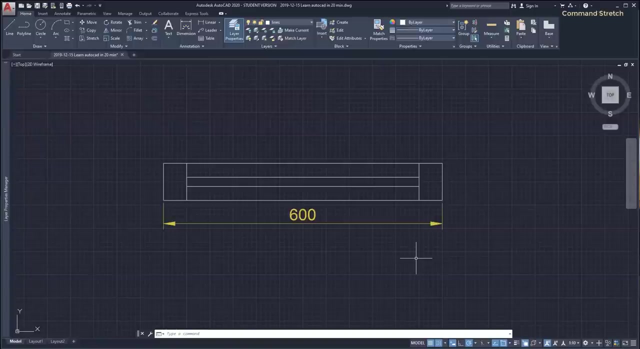 create them again. but in general, insert PDF can be very useful. just be aware that they are available in the versions after AutoCAD 2017 Stretch objects. sometimes in AutoCAD we need to stretch figures. let's learn how it works first. it's important to have in mind. 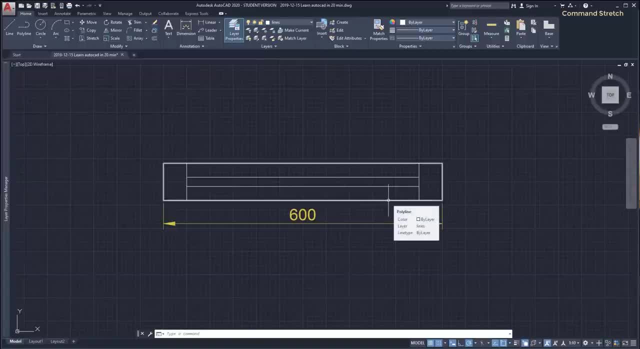 that this operation doesn't work for blocks. as you can see, here I have only lines and polylines. let's do it. I'm going to click on the command- it's this icon here. then I have to select the part to actually stretch. so I open the selection. 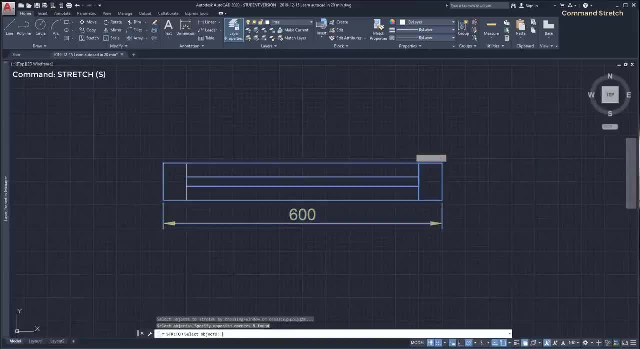 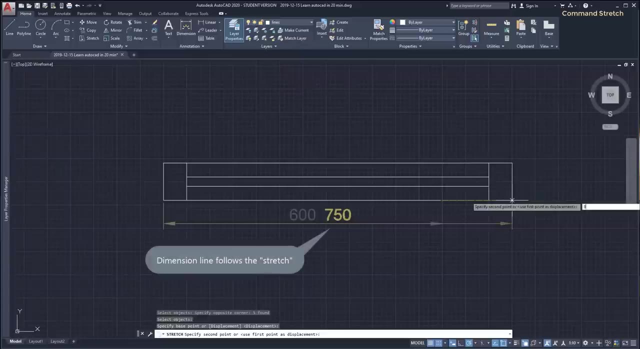 from the right just until here. then I specify this base point. as you can see, I'm extending and moving objects to this side and as the dimension line was in the selection, it is also readjusting. now I can click to place the objects exactly how it's on the screen. 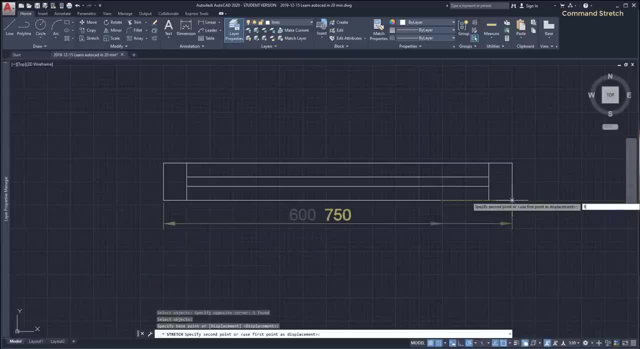 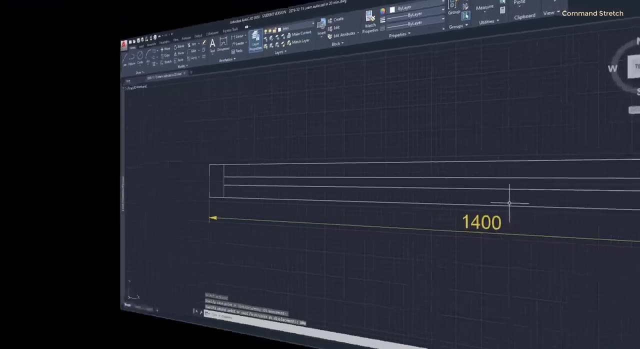 however, it's without any kind of precision or type a distance to extend. if I type 800, actually I add that value to the original length of 600. the total is 1400. the way that the objects stretch depends only on the selection. even I select a different base point. 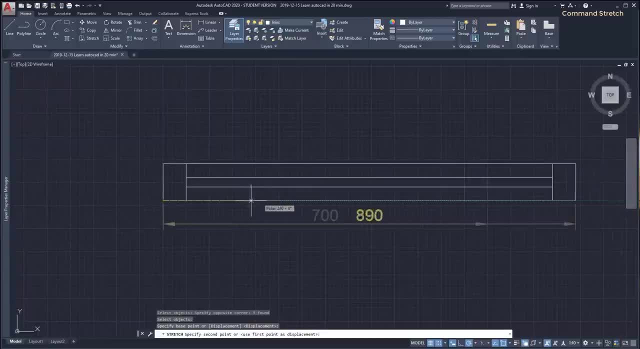 the result is the same. let's repeat this again, and this time I want to change the selection to cover also this line. I press enter and you can see the objects stretching differently. now I want to try to stretch vertically. I select the objects, press enter and oh. 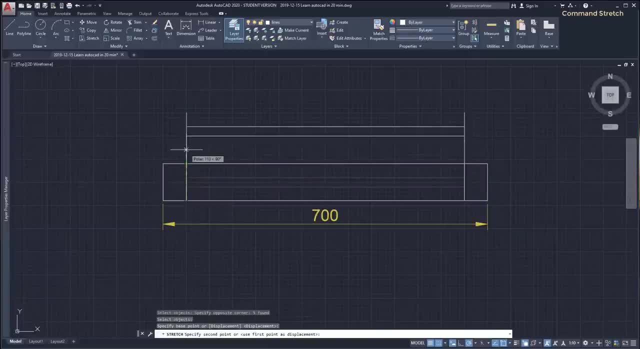 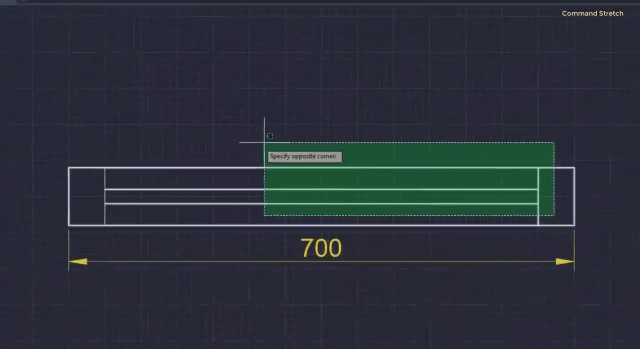 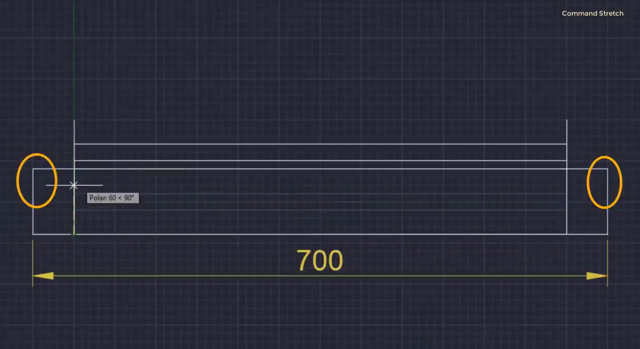 it's not as I was expecting, but I select all the objects. why does this happen? when I was doing the selection, I kept these sides outside of the selection area and even everything was selected, because the external rectangle is a polyline, a single object. the really important thing. 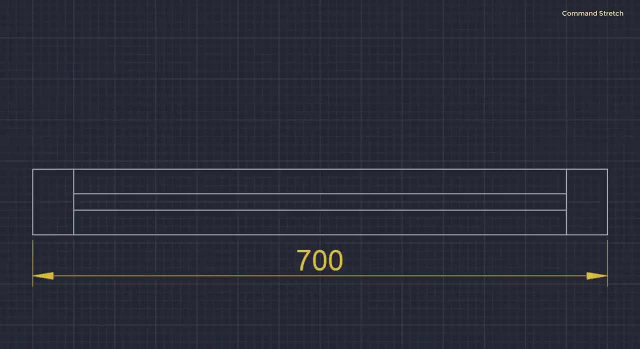 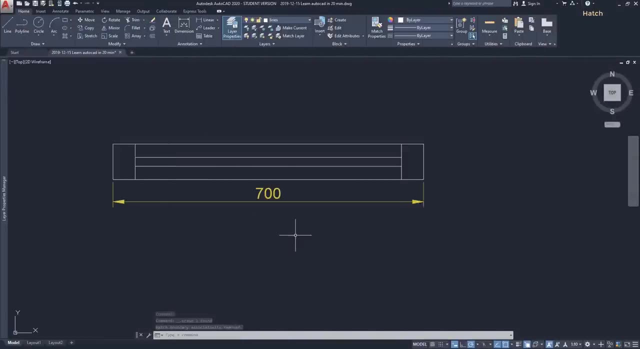 here is what actually I am covering with the area hutch in this section. I will be talking about a drawing tool which is used to fill enclosed areas. it's the command hutch. but first I am going to create a new layer in this file. let's check out if you remember. 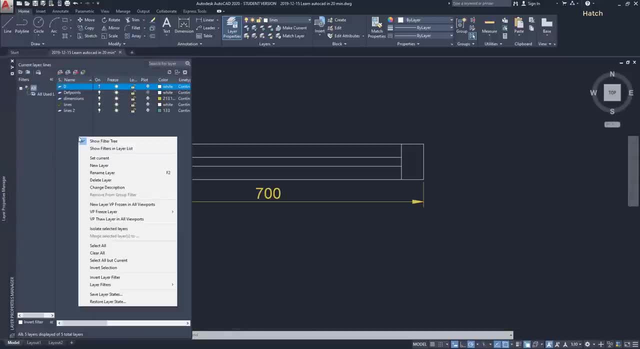 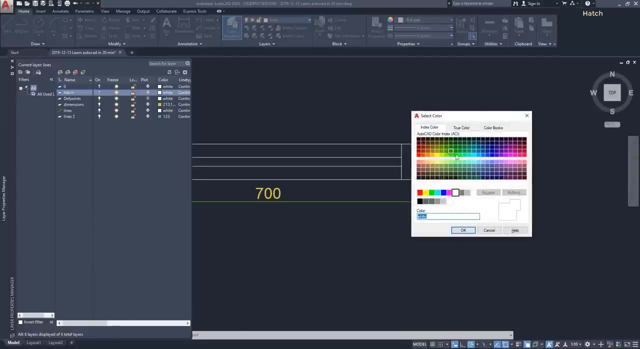 how to do it. I go to the properties manager, click with the right button and new layer. I name it as simply hutch. then I am going to choose a color for it, for example, this kind of pink. ok, now I am going to turn on the command hutch. 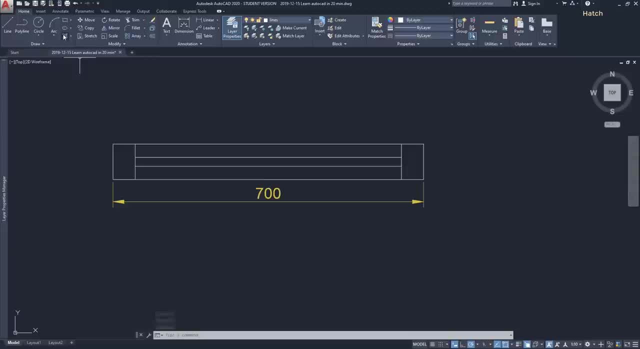 it's located here at the drawing panel. wait a few seconds if you want to read the description of this tool. sometimes it can be interesting then to apply a hutch click on it and I have to click inside an enclosed area. it can be any of these rectangles: 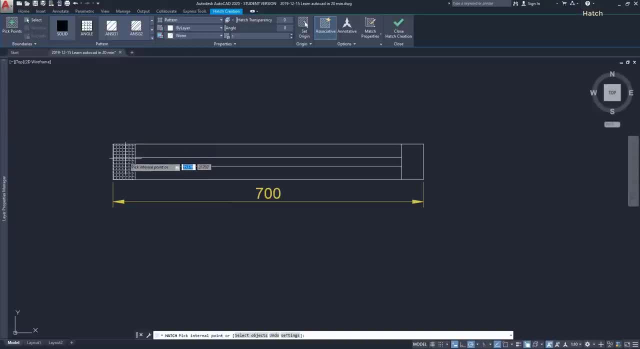 I click to fill this one. ah, it's in a white color. I forgot to change the layer. yes, when you create a new layer, you still need to set it as the current layer before you draw the objects in, otherwise it will not work. go to the layer tab. 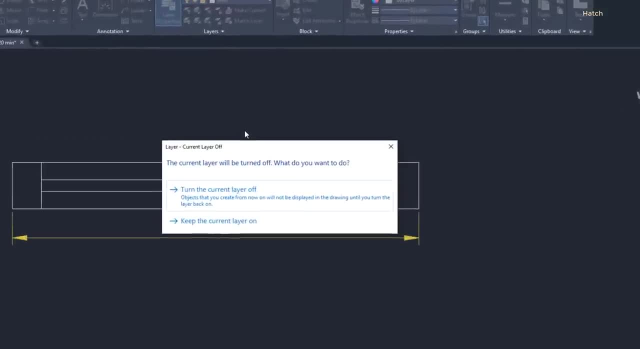 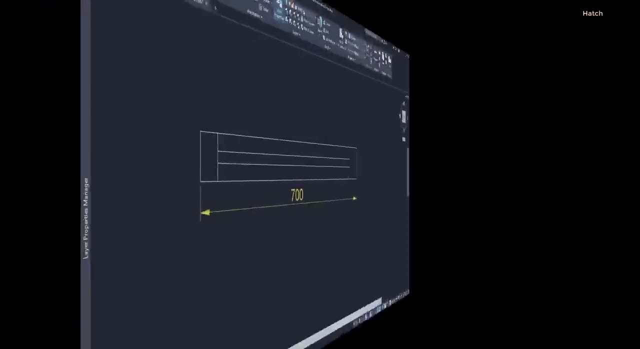 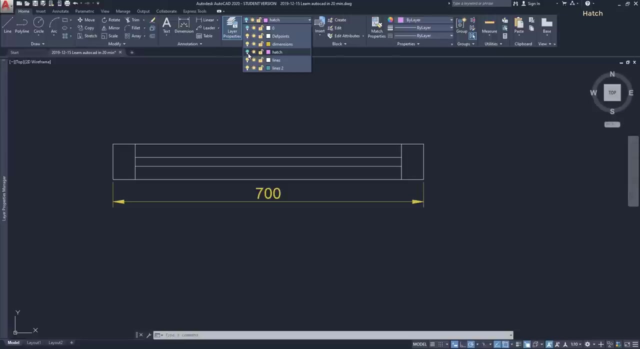 and click on hutch. hmm, now I see this message appeared. the current layer will be turned off. what do you want to do? for any reason, this bulb is switched off and if I draw objects on that layer, they will not be visible. click to turn it on. 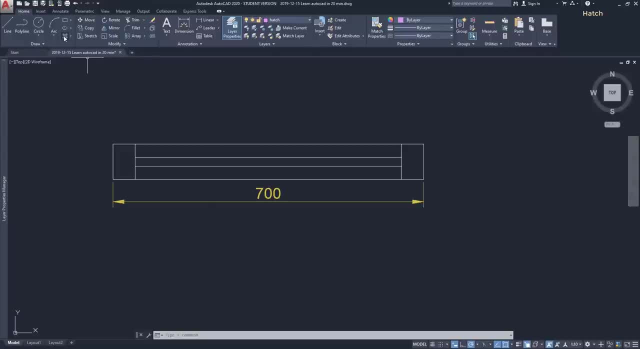 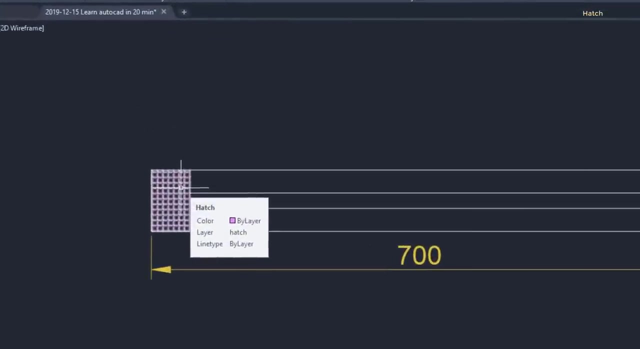 I am going to repeat the process. click on the command hutch and fill that area. now it's on the correct layer, press enter to confirm. then, by dragging the mouse over, you can see that it's a hutch object. now I will show you another way. 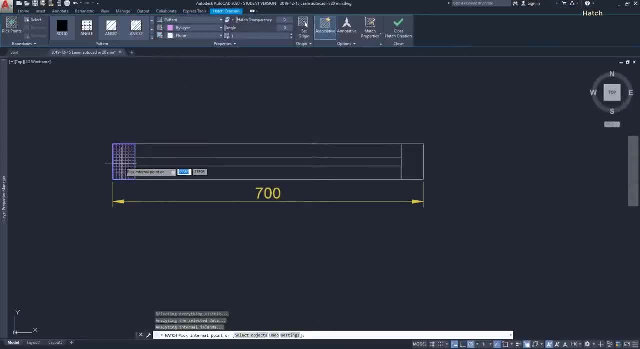 to use hutch. I click again here and then, instead of pressing enter, I fill a different area right away. what happened is that both areas are now a single object: hutch editor. above, a new tab appeared. I am going to show you briefly the functions here. I am going to click on this button. 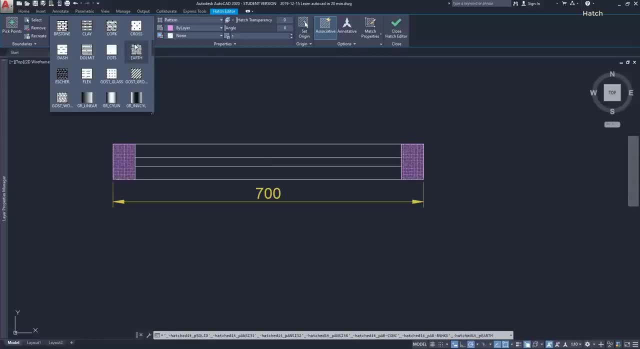 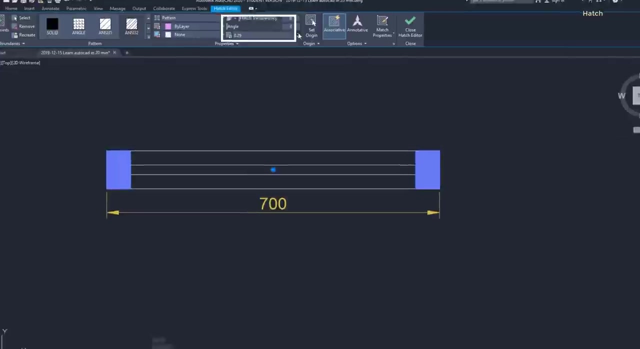 at this panel and you can see a lot of patterns to use here. the first one, solid, is the simplest one. it fills the area with just one color. I choose, for example, this: now let's have a look at the options at this side. on these controls, I change the scale. 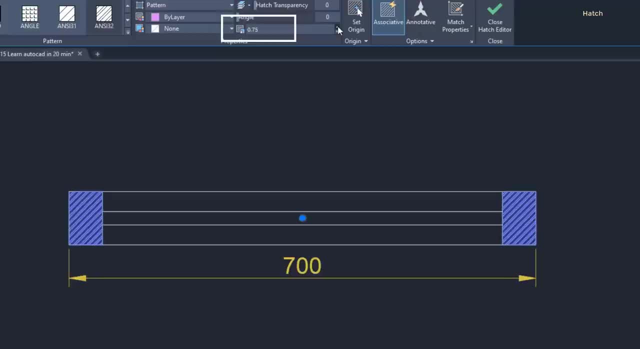 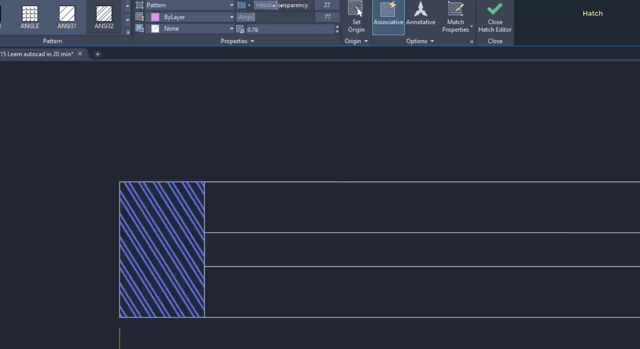 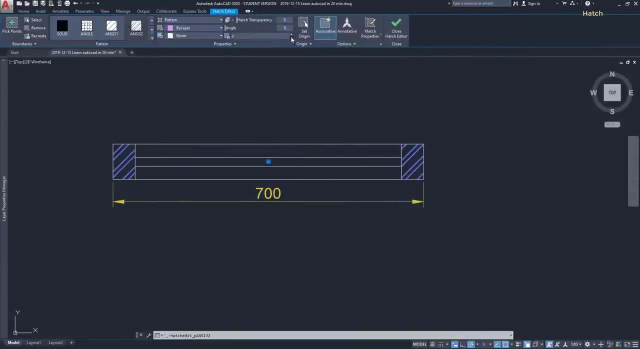 look how is the effect. on the angle tab above, I can rotate the pattern. finally, on hutch transparency, I add a transparent effect to the objects. I want to mention one thing. when I first press try to change the scale by clicking on the controls, I realized that these values 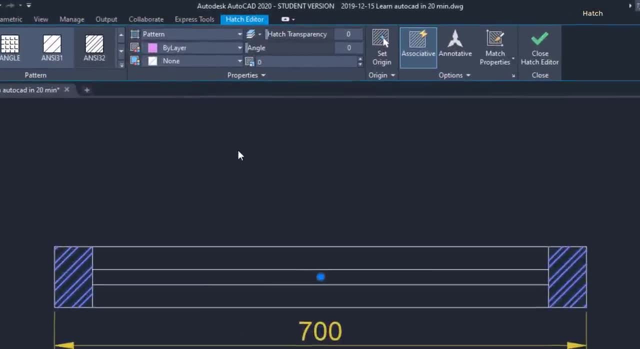 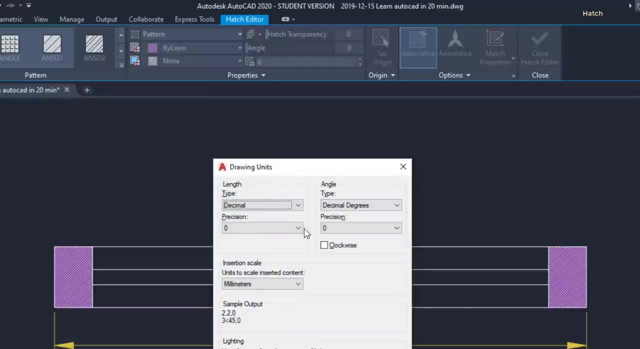 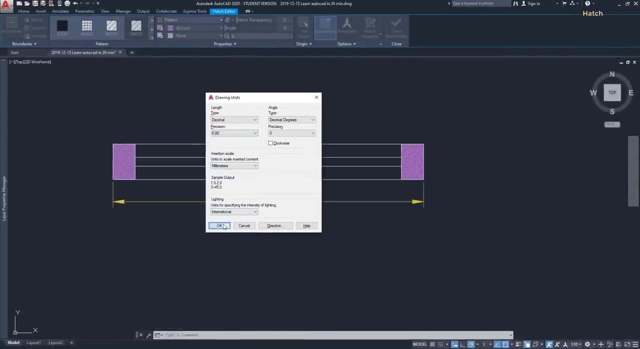 didn't change a lot. even if I type a number with decimals, it shows just zero. when this happens, it means that I should go to the unit properties, type un and press enter, and in this tab I need to set decimals, for example two decimal cases. then it should work fine. 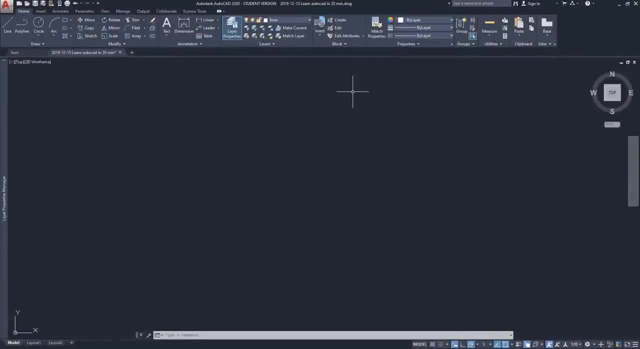 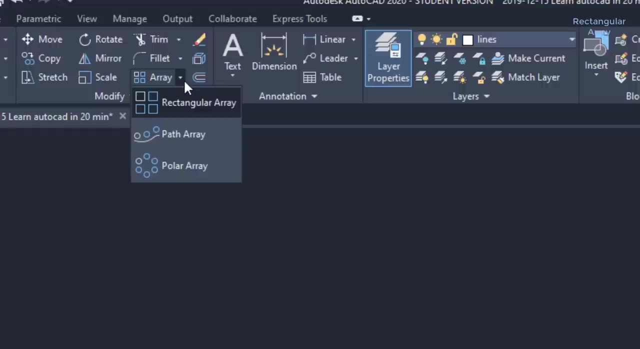 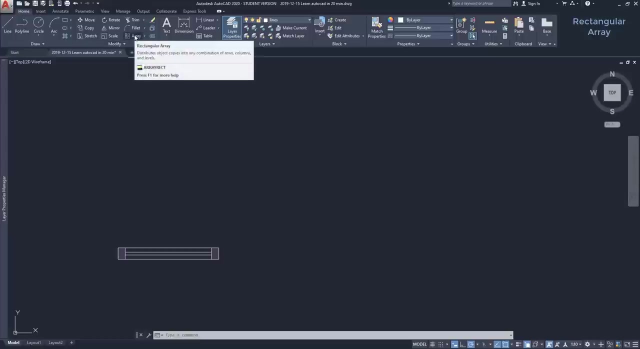 part 5: how to use array. with the command array we can copy objects arranged in a pattern. there are three different modes: rectangular array, polar array and path array. I start with rectangular array, and for that I just need to click on the button set by default. then I'm going to select. 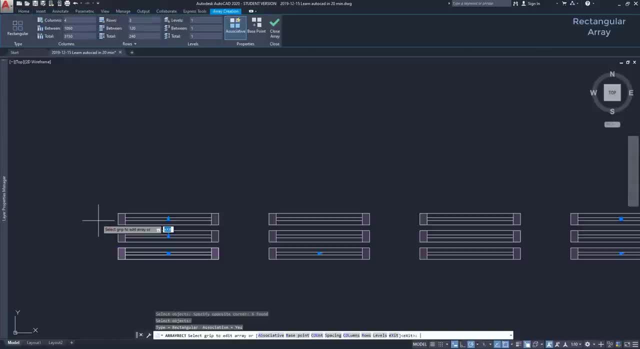 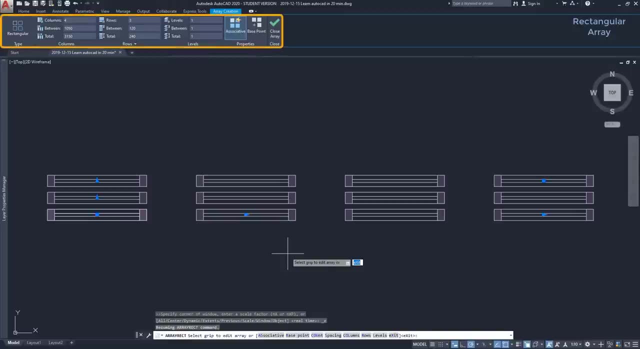 these objects and press enter. so an array was generated and the special tab on the ribbon has appeared. now I can edit this pattern as I wish. here I can set the number of columns and rows. if I decrease the number of columns, for example from 4 to 3, 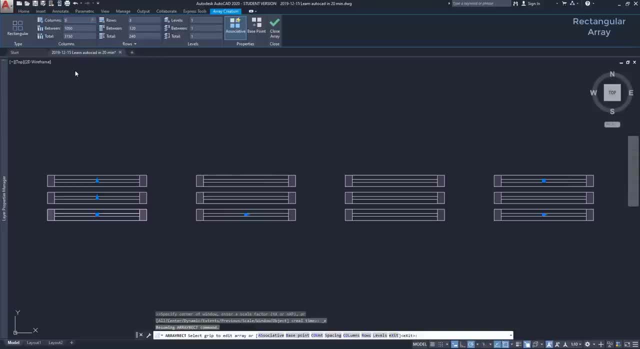 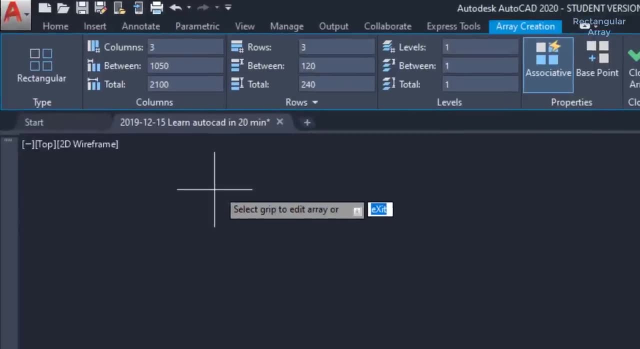 as you can see on the screen, the last column is suppressed, the array creation. I find it very intuitive and I think it's easy to understand the options here while looking to these little drawings there. the distance between is the distance from the origin to the beginning of the next element. 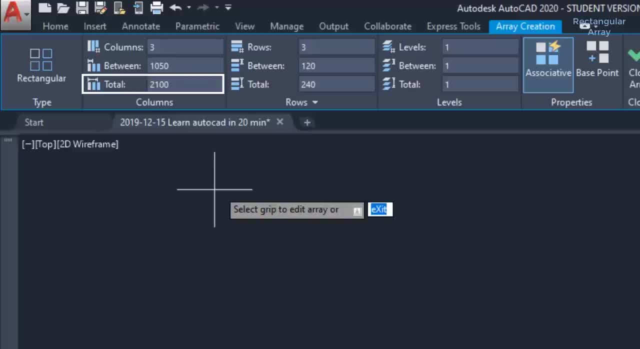 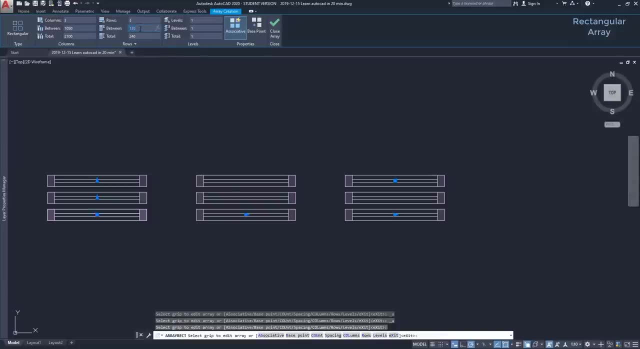 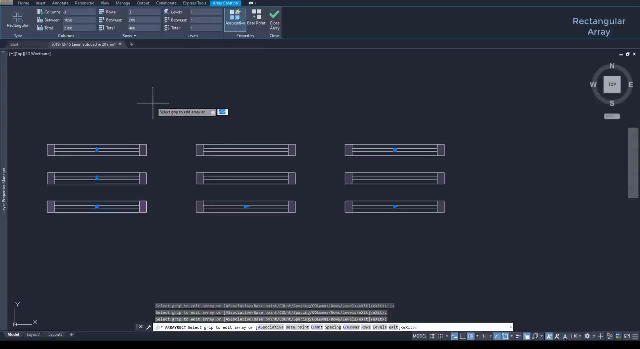 the distance total is from the origin to where the last element starts. simple, I'm going to change the distance between rows to 200 and look how the pattern moves. of course, the total distance was updated in order to match to the new distance between lines. to exit the array mode. 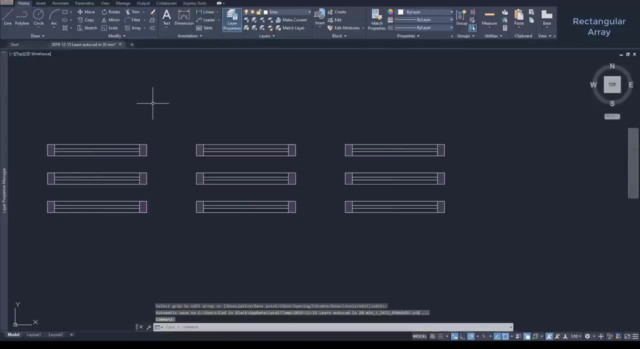 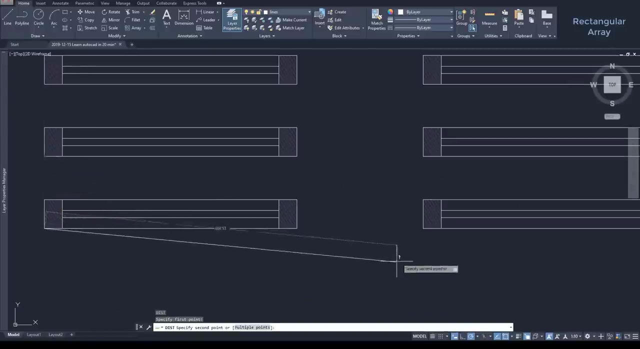 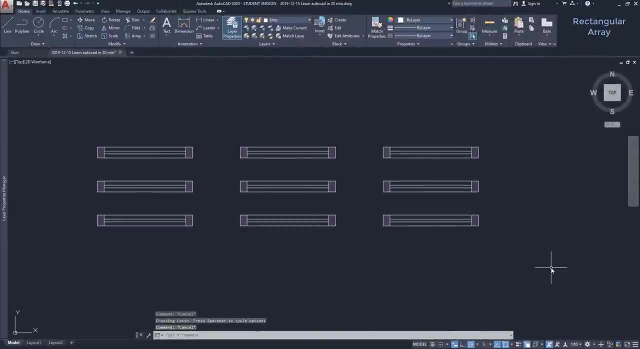 I press escape. now, if I want to confirm the distances, I can use the measure tool, type DI and press enter. notice that the vertical length between two elements matches, as well as the horizontal length grips in an array object. whenever I select an array, you can see these dynamic grips. 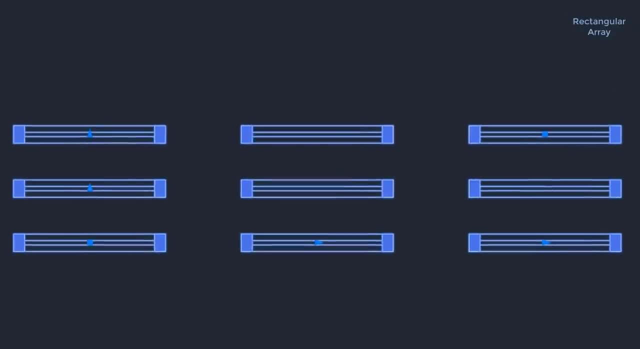 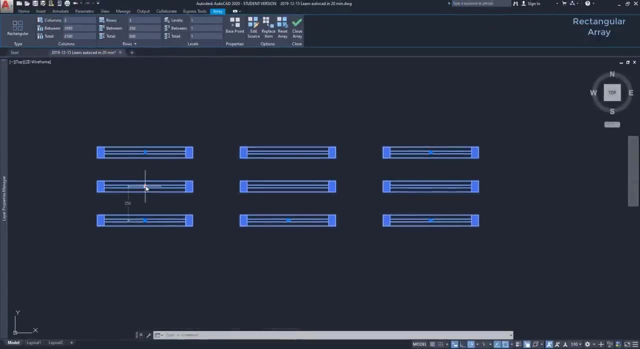 the blue buttons here which I can use them. for example, if I click on this one on the second row, I can change the vertical distance between two objects. for that, I simply type the new length. to change the horizontal length, on the other hand, click on this one. 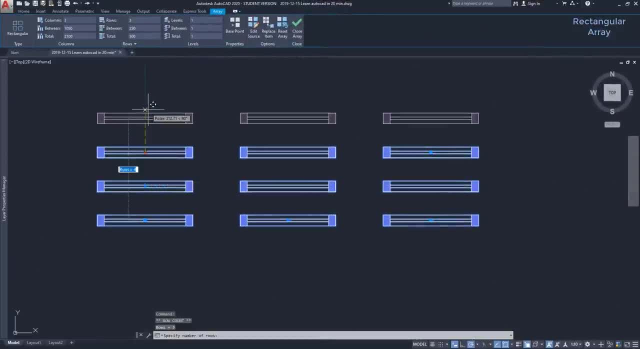 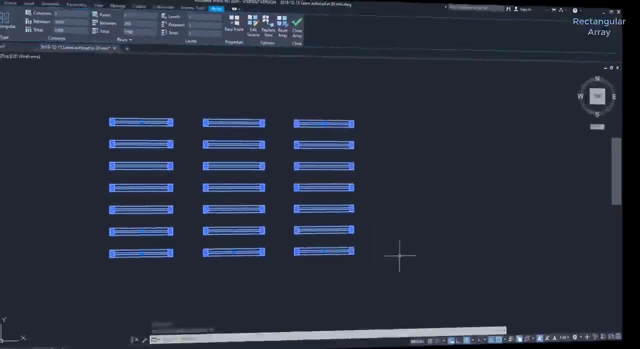 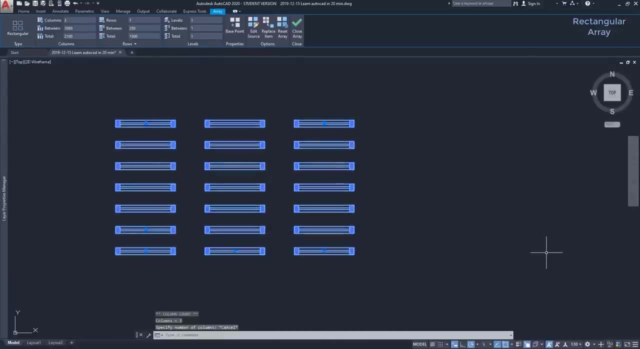 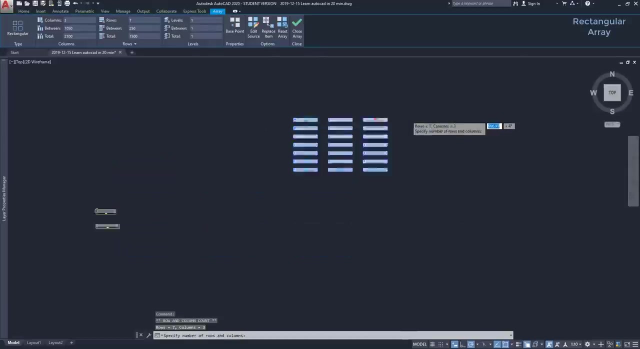 if I click on the grip at the last row, I can add more, for example 7. if I click on this side, it's the numbering of columns that I can change. the grip on the opposite corner changes both rows or columns by dragging the mouse. basically these operations. 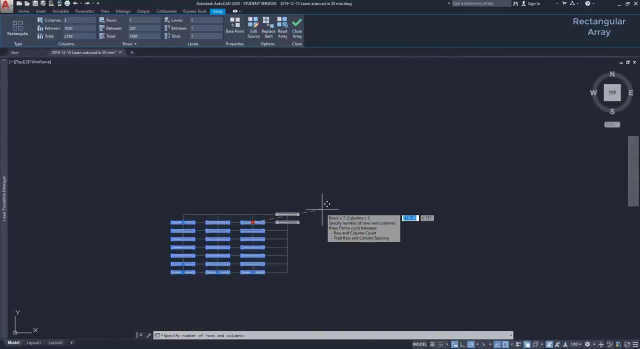 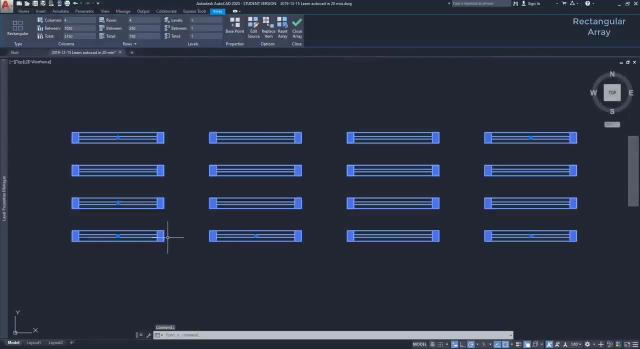 can also be performed on the array tab, but sometimes it's just more practical with these buttons. another useful thing in array is changing the base point. I click on this icon, set the new point, for example on the corner, and the grips moved with the base point, but they perform exactly. 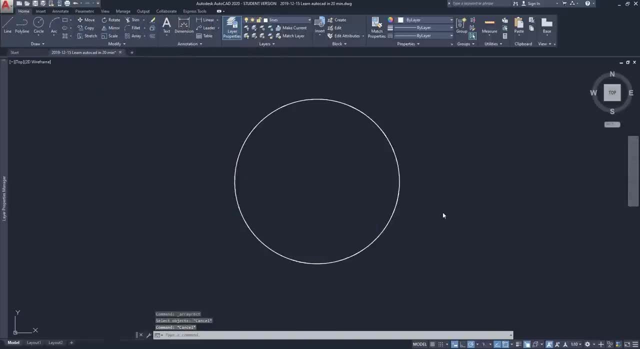 the same actions. let's make a polar array. I'm going to draw a small circle with its center located at the boundary of this big one on this side. now I can click on the command polar array. it's this one there. basically, what I want is to have this object. 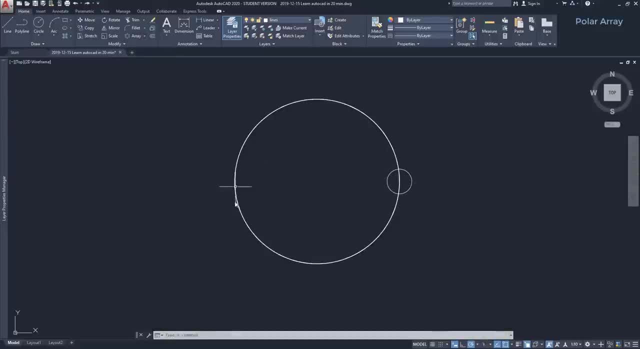 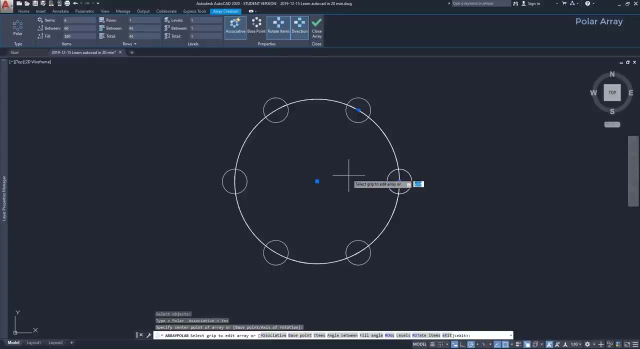 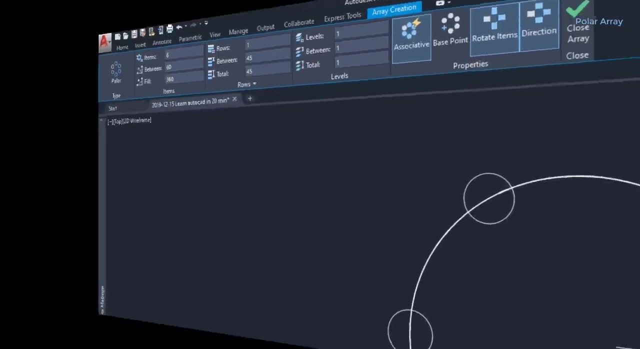 displayed around. I click on it, then the center point of array is going to be the center of the big circle, and that's the result. the program sets 6 circles around the center point by default but, like for the rectangular array, I can edit this on the tab at the ribbon. 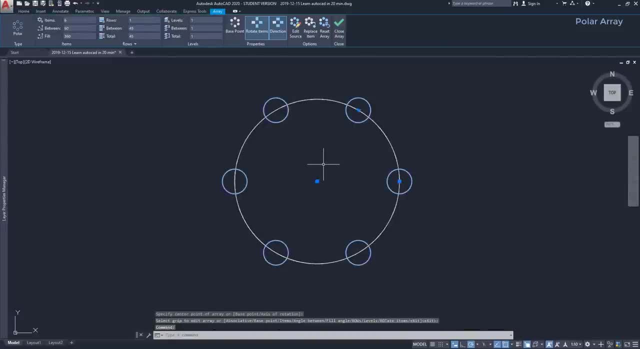 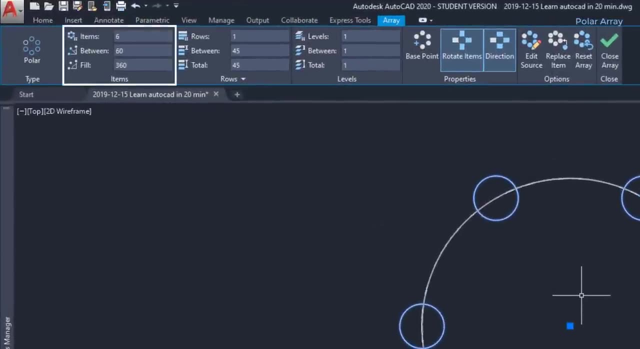 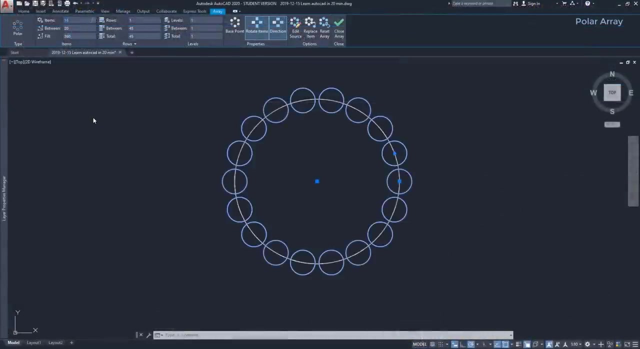 so the array tab for polar array is a bit different, especially the panel items. on the first parameter I set the number of items. in this case I specify 18, and they cover all the circumference, because I have 360 degrees in between, I specify the angle between two items. 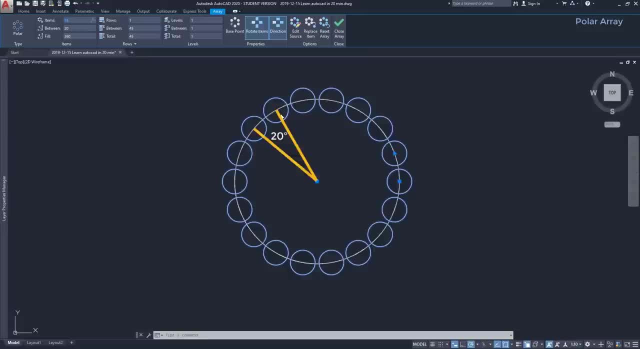 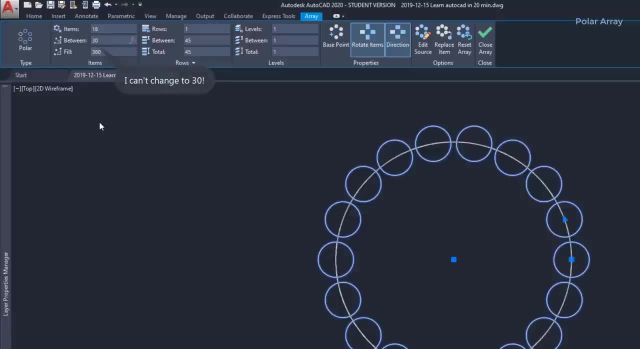 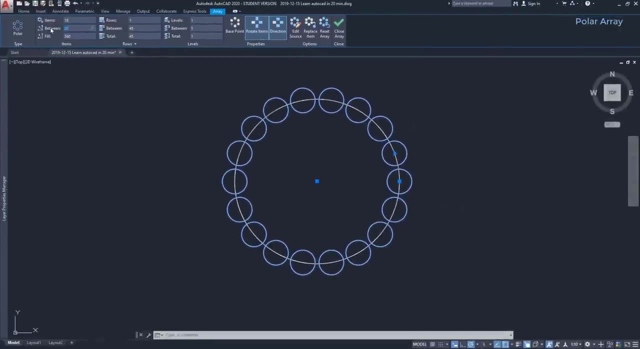 and in this case it's 20 degrees. if I try to change the angle to 30, you can notice that it doesn't work, because it's not possible to fit 18 items with that space. let's try 15 degrees. so what happened here? in order to 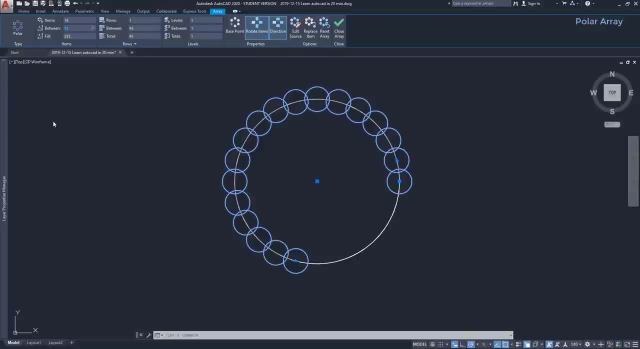 keep 18 items. the angle on fill was updated. now it's only 255 grips on polar array and tips. the small square on the original item allows me to change the radius of the array. I'm going to set, for example, 50, and this is how it looks like. 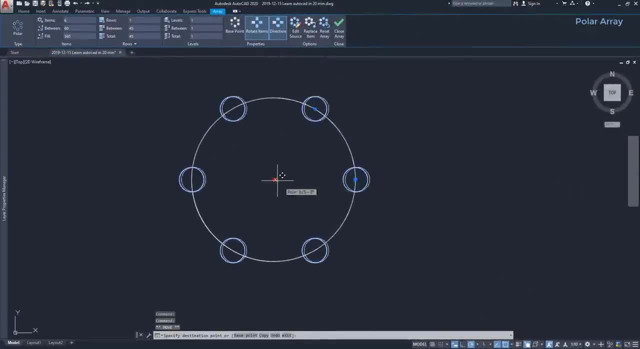 the grip on the center can be used to change the position of the array. on the other hand, if I click on this little arrow, I change the angle between two items. let's suppose I want 6 items. the angle to have them distributed equally is 60 degrees. 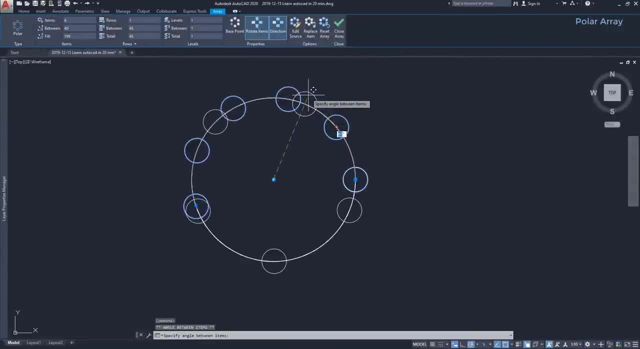 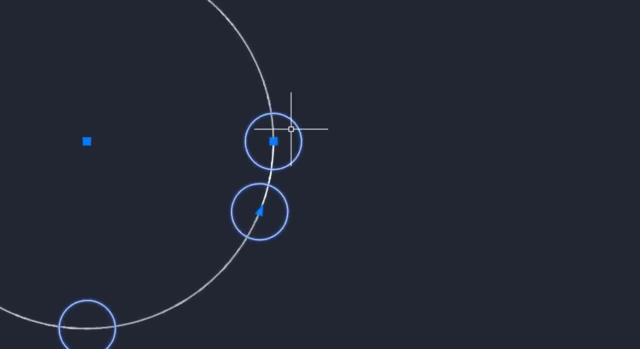 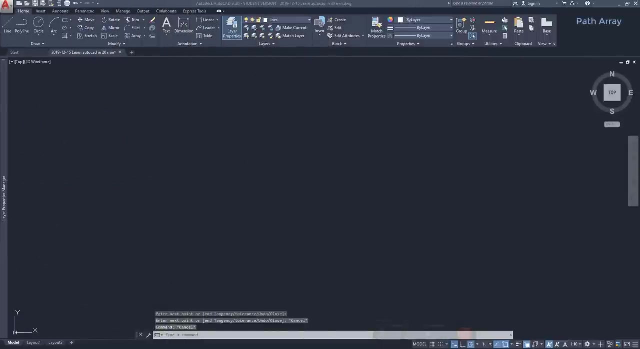 however, it's possible to increase a bit that angle, but the last and first item will stay closer than the others. path array. the third array mode available in AutoCAD is path array. we can copy objects along a line or a curve. let's see how it is. 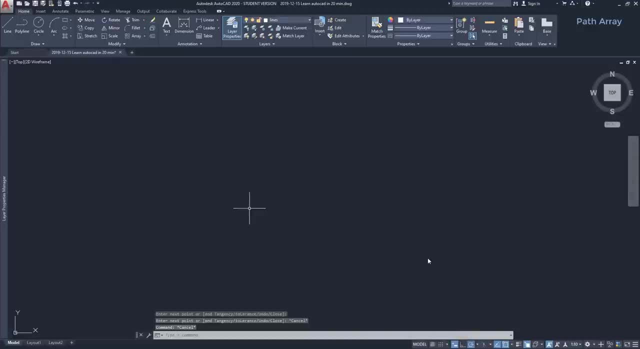 first I'm going to draw a spline, which is a smooth curve. I click on the command located here, spline fit, and I can draw a curve by specifying some points on spline fit. the curve crosses exactly the points that I insert. when I finish. I press enter here by pressing escape instead. 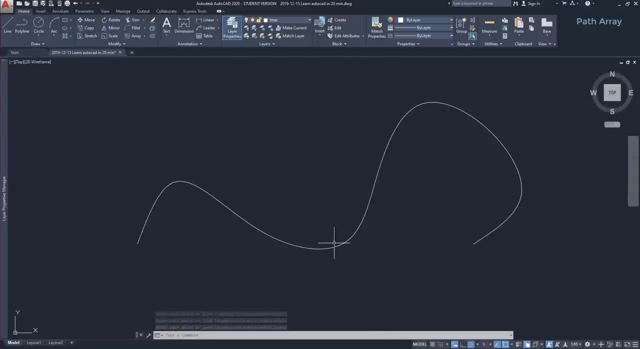 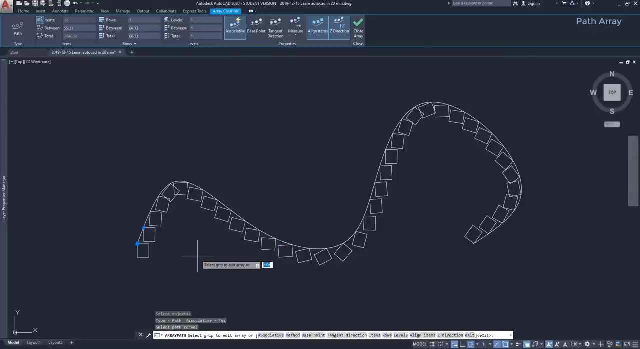 it cancels the command, it will not work. next, I draw a rectangle on the first end point of the spline. now let's use the path array. I click on the icon, select the object to copy, press enter and then I select my path. so I have made it. 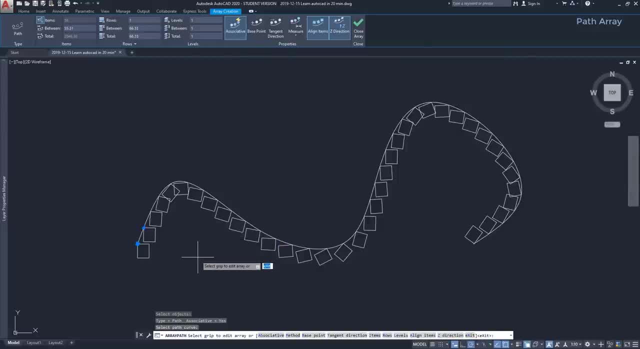 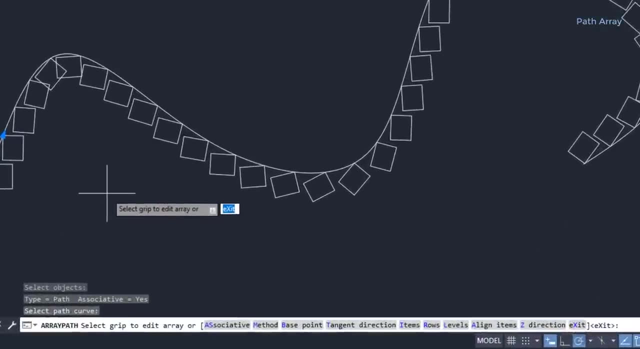 however, probably I want to edit the spaceman position and rotation at the command bar. you can easily check out that. there are several options to edit. let's analyze some of them. base point. the base point will be exactly at the start of the path. I click on the option. 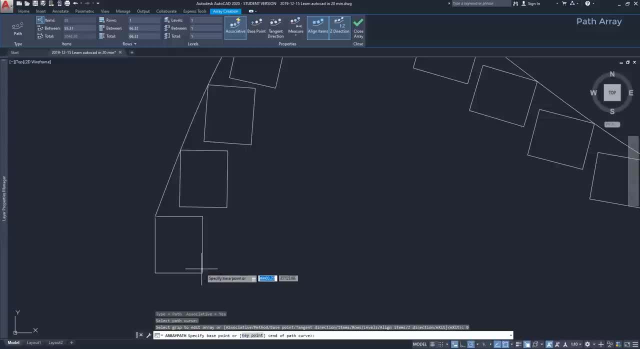 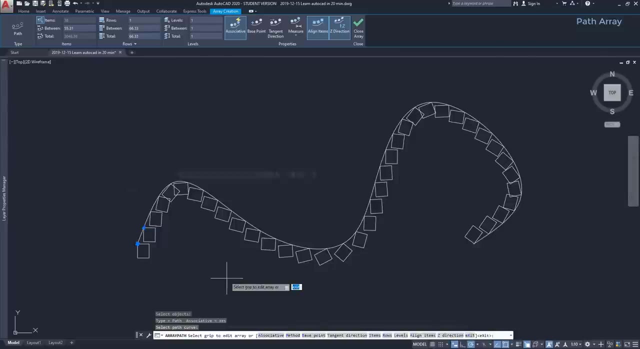 then I change, for example, the base point to the opposite corner, and that is the result: the object is moved, but without rotating tangent direction. this one is useful if I want, for example, to have tangent with the curve. I'm going to click on the button tangent direction. 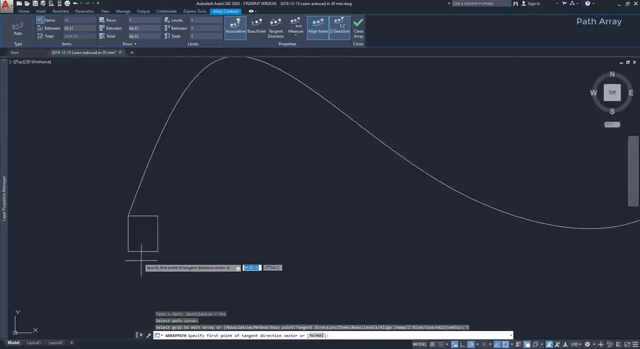 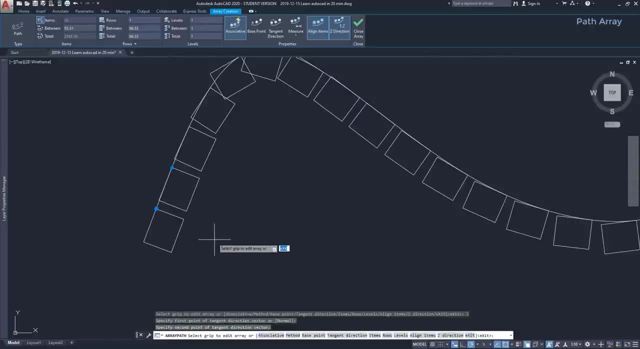 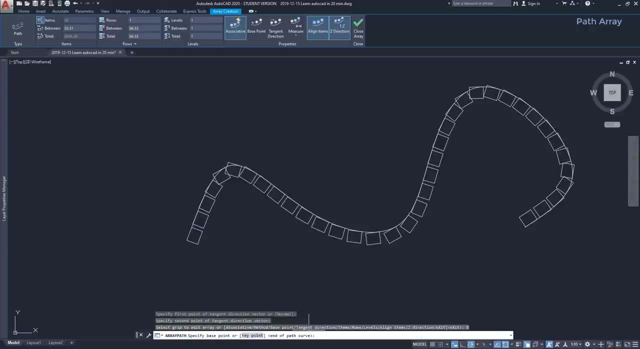 then just specify two points and the objects will rotate. but now suppose that I want the path to cross the center of the objects. I'm going to use the option base point and click on the center of the rectangles, mmm, but it's not snapping to the center point. 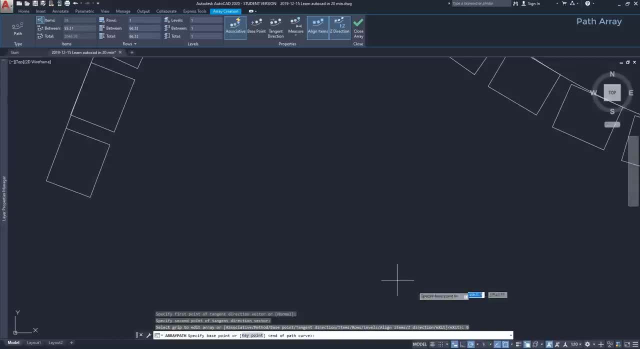 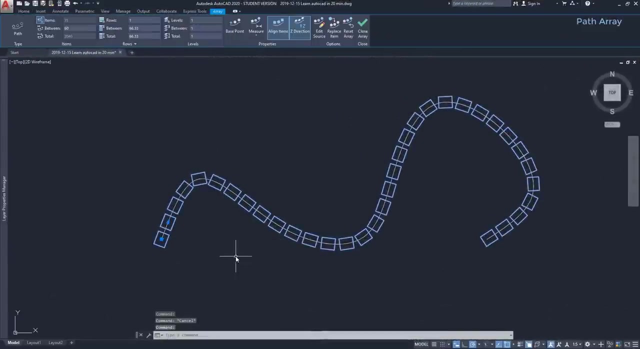 if this happens to you, it means that you should turn on the mode geometrical center in object. snap, it's this one. now it's going to appear. I just need to hold the boundary first and click on the center array tab on the ribbon. the tab on the ribbon. 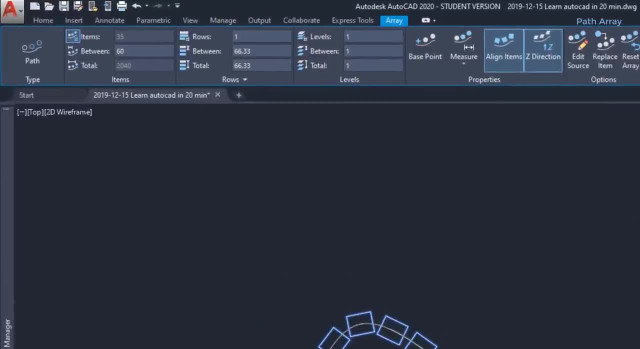 is now specific for path arrays, especially the first panel. I can change here easily the spacing between total spacing and number of items. I think the best way to absorb these things is to simply practice. you can play around with all these options and after a while it will be easier for you. 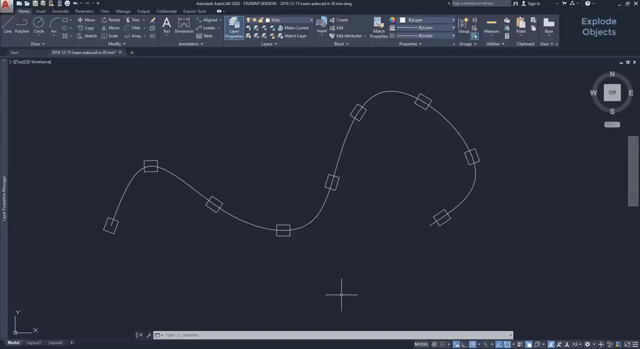 explode objects. once I create an array, all the group is considered a single object. now imagine that I want to get rid of the array it doesn't work with. just select it and press delete. it erases the the whole thing. as you see, what I need is the command explode. 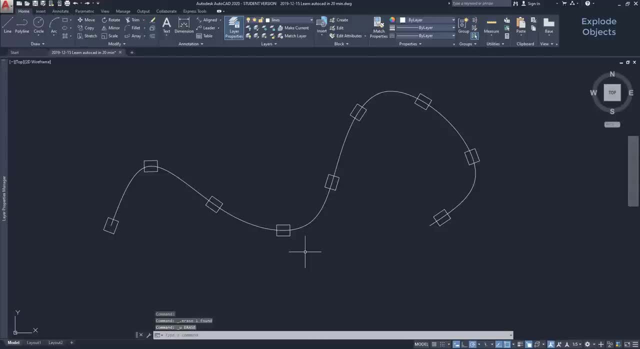 it basically returns a compound object to its original components. it's very easy to use this. I click on the command explode, see select the array, and press enter. as you see, all these are now separate polylines. then I can manipulate the objects as my preference. consequently, 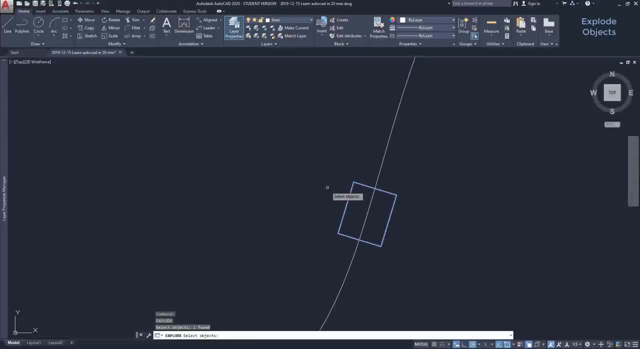 I can explode a polyline in separate lines. another way to use explode is on blocks and I can also use objects like hatches and other kind of objects, but some of them it doesn't work like text. utilities panel. let's talk about the utilities panel and I'm going to start. 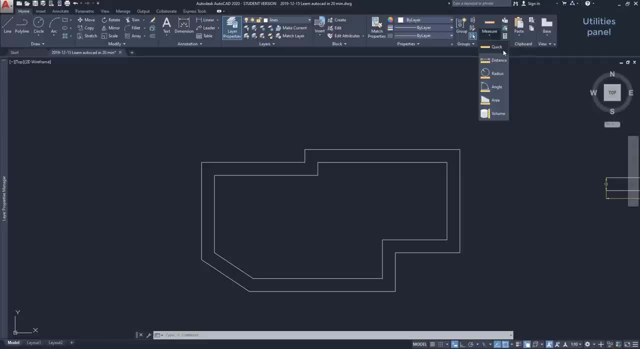 with the measure tool. there are several ways of measuring, as you can see here, which is the one set by default when you click on this button for the first time. when I move the mouse over the objects, some dimensions appear on the screen and these yellow lines measure. 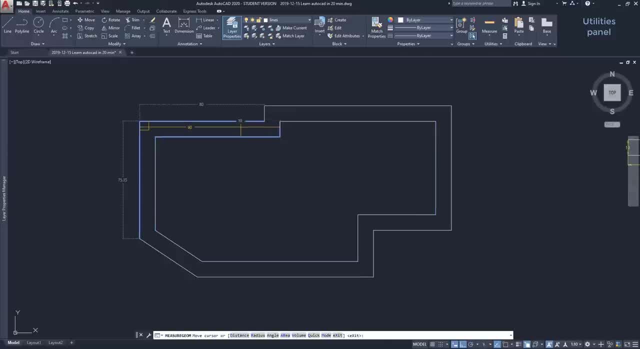 vertical and horizontal distances between the closer objects. on the other hand, if I try to check the dimensions in a circle at the first time, it looks a bit confusing all these values here. but they just show the radius. for example, 100 is the radius of the biggest circle. 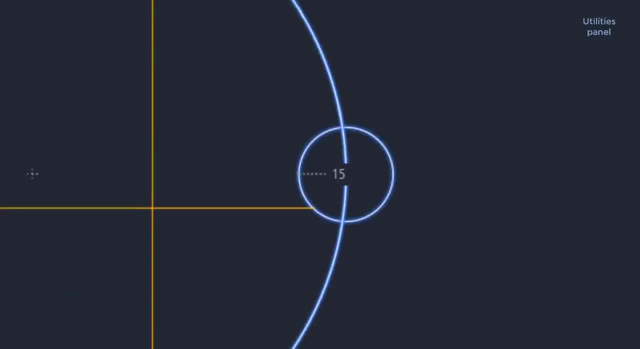 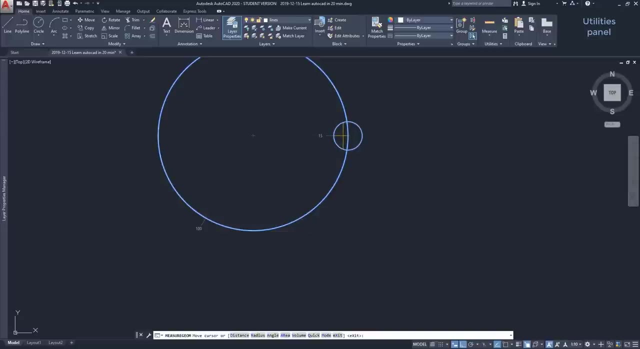 as well as 15 is the radius of the smallest circle. the yellow lines don't measure anything here, just don't care about them. honestly, this quick measure, it's not my favorite, because even it's true that we can have a lot of information at the same time. 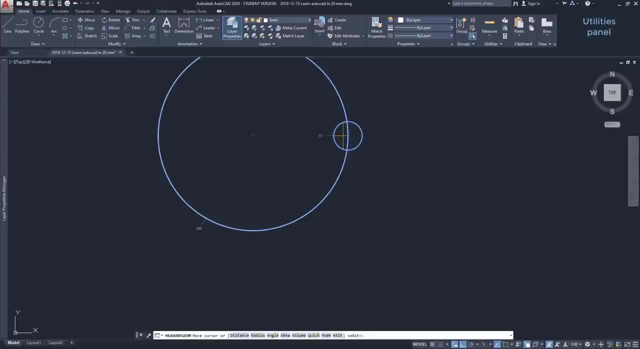 it can be a bit confusing, but of course that is just a personal taste. the icon distance: I use it a lot as I find it very intuitive. it simply measures the linear distance between two points. another one which is very easy to use is the radius. I only need to click on a circle. 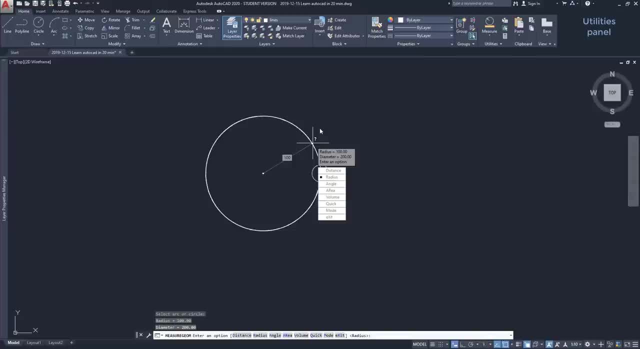 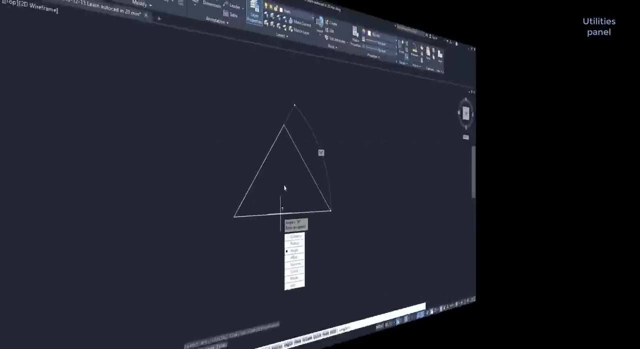 to check it out: measure an angle. this one is simple. I can select two lines to measure the angle between them, or I can check out the angle of an arc by clicking on it. now let's go to where I was before. I want to focus on something. 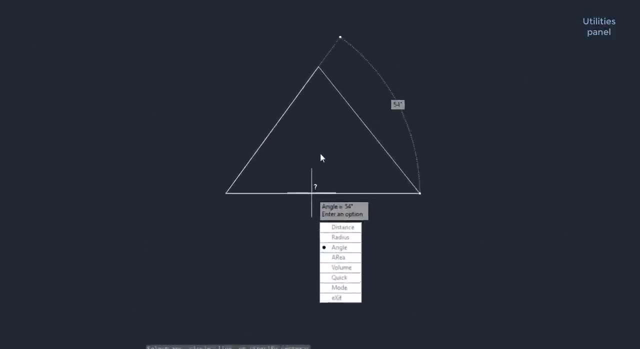 when I select the objects to measure the angle, this menu appears where I can choose from different types of measures. I can click on, for example, area, and with this I can measure the area of the triangle. it's very simple: I just need to click on all the vertices. 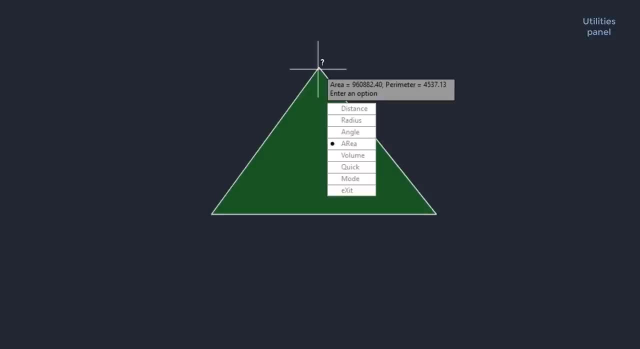 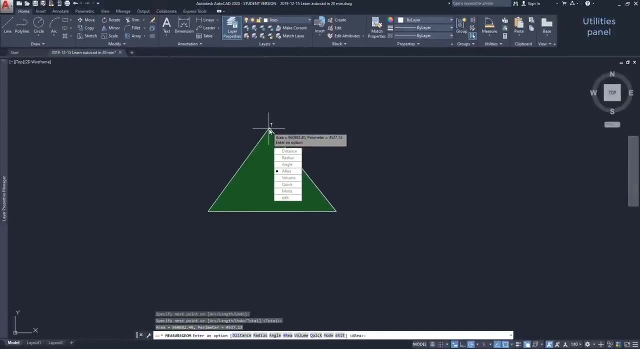 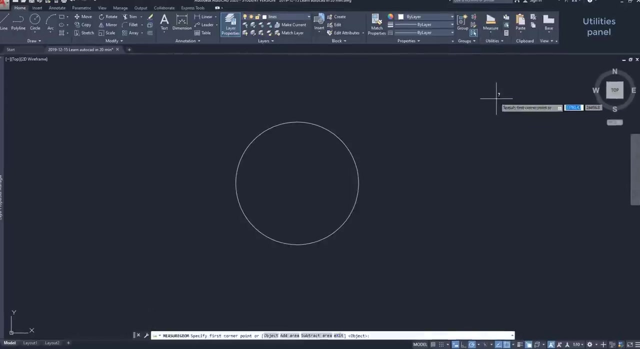 and press enter at the end. then you can see in this box the area and the perimeter. but how could I measure the area of a circle, since it doesn't have corners? I click on the icon. then at the command bar I can switch to object. I type O and press enter. 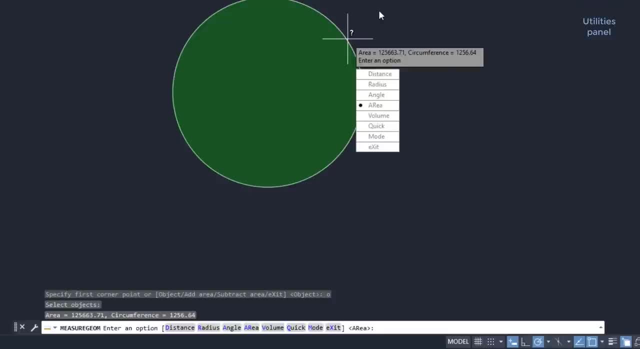 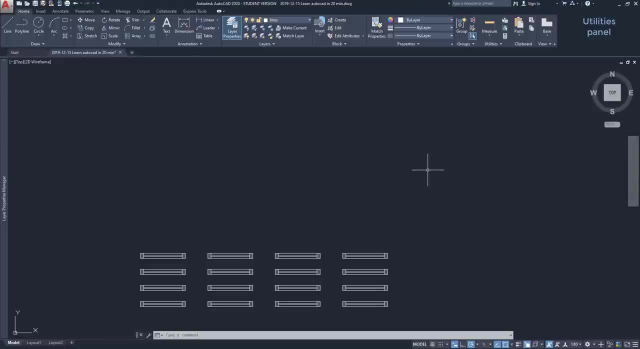 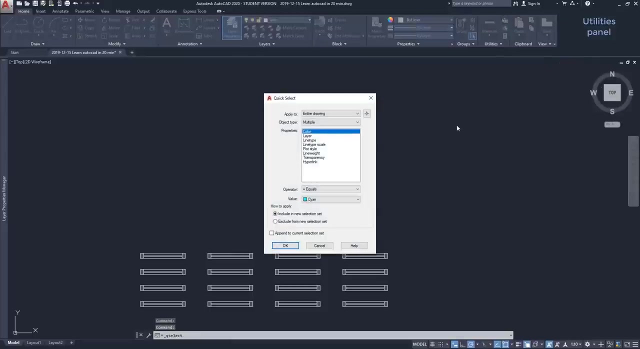 finally, I just select the circle quick select on the utilities panel. you can find other tools at the small icons at the right. the first one above is quick select. if I click there, I open this window. I can select all the objects by using filters. for example, I can specify a type of object. 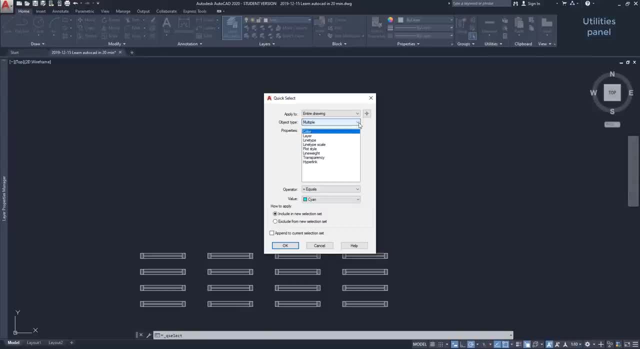 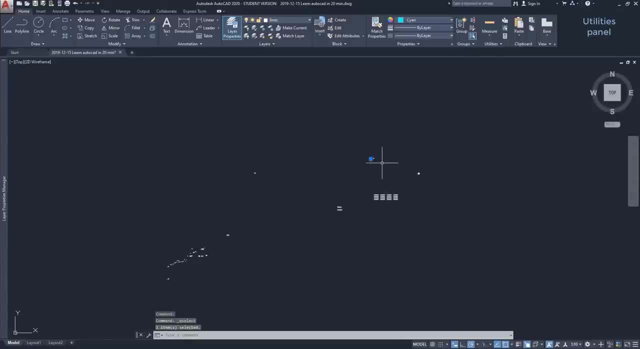 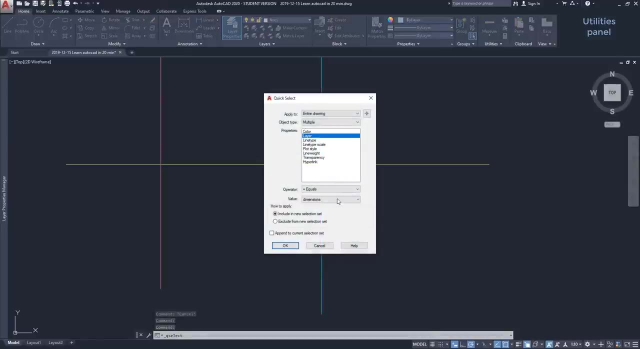 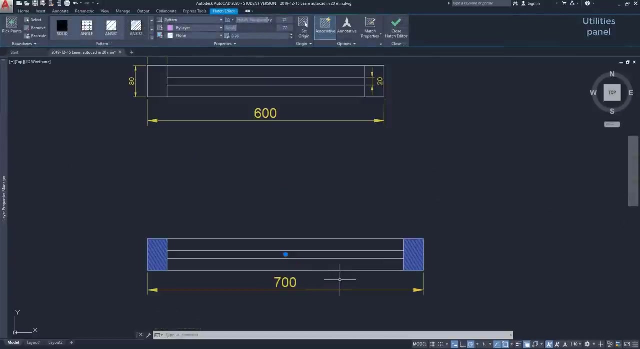 or select by color. now I will select all the objects with color cyan, click on ok and here it is. this is the only one in this color. other options can be: select all the objects of a specific layer or you can select by line type, among other options. 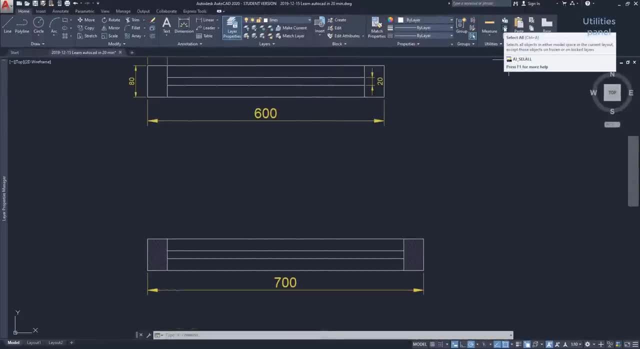 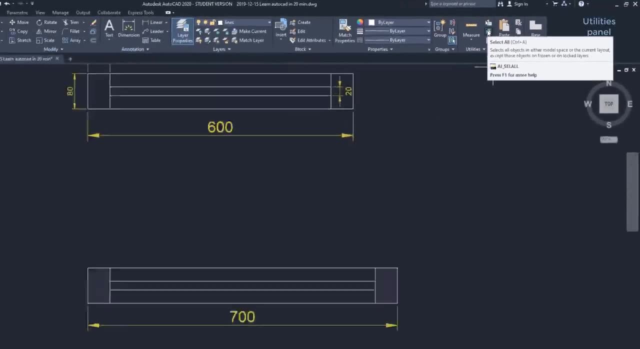 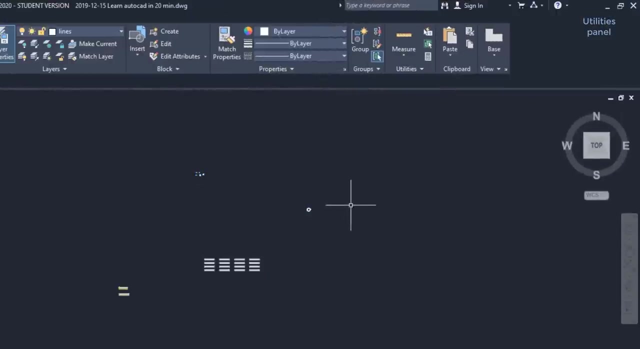 if I click on this icon, I select all the objects in the workspace except the ones that are frozen or unlocked layers. the button below is the quick calculator. actually it's a kind of scientific calculator, and there we can do from basic calculations to a bit more complex ones. 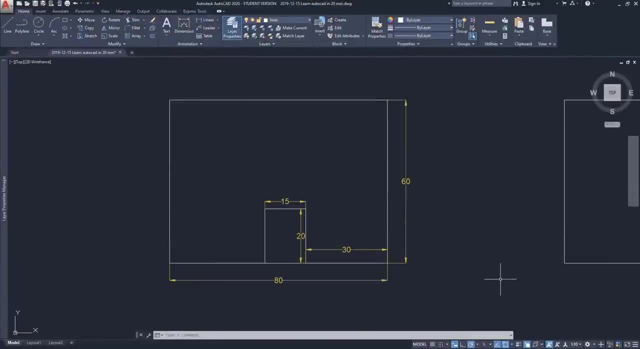 dimension lines. now I am going to teach you how to draw dimension lines. this is a classic feature for annotation in your drawings. in this figure, you can see the dimension lines indicating its distances. now to draw dimension lines: there is a panel on the home tab, here, or if we go to the 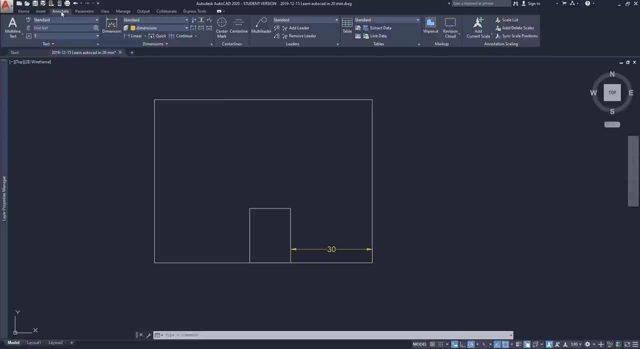 annotation tab, we can have all the tools. so there are several types of dimension lines whose you can find them by clicking on this arrow. for now, let's start with the most common one: linear dimension. to insert a dimension line, I just click on two points, then I click again to put the dimension line. 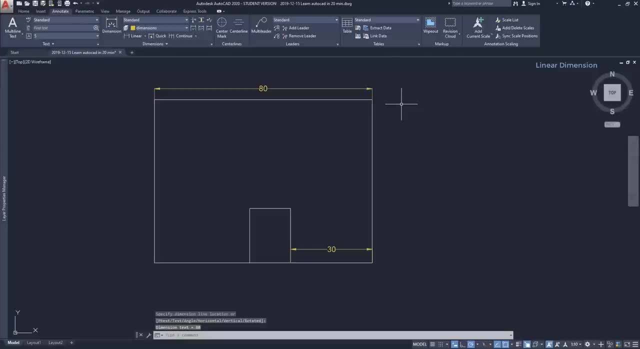 on the place that I want. so it's very simple. however, this feature is quite complex and we usually have to set up some settings. sometimes the dimension lines are not proportional with the sizes of the objects that they measure, so I am going to open the dimension style manager. 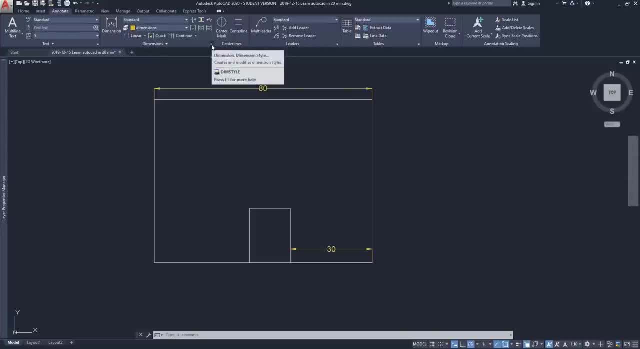 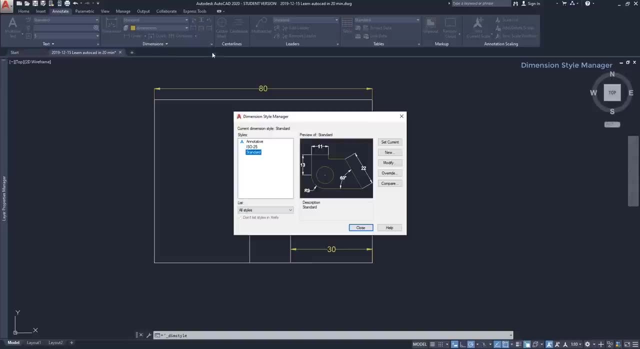 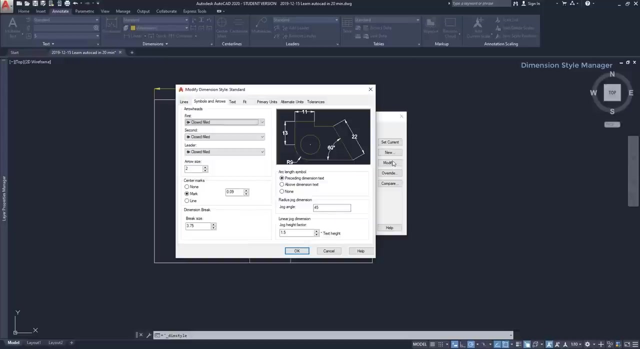 by clicking on this little arrow here. I need to choose the dimension style that I want to edit. I select standard, which is the current one, and I click on modify. now there are lots of options here, but for a beginner the most important is the size of the text and arrows. 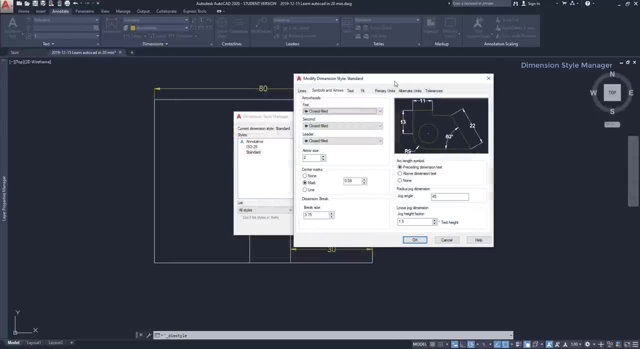 as well as the units. go to symbols and arrows tab, look for arrow size and put a value that seems convenient. then the size of the text can be changed in the text tab. as you see, both sizes have a height of 2. to confirm this, I can always measure. 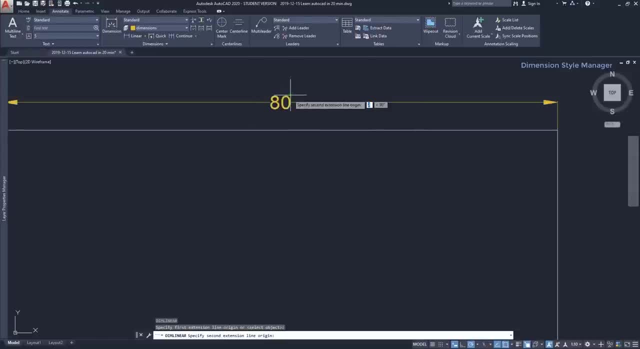 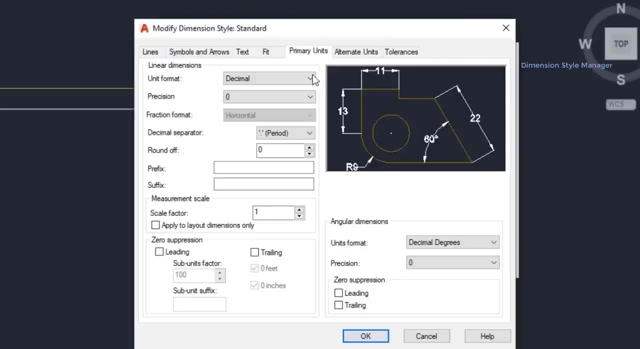 the distance. here you can see it's 2. on primary units tab I can edit the unit format, the number of decimals- let's change it to 2- and I can add a prefix or a suffix. for example, suppose that the units here are emitters. I can type the symbol m. 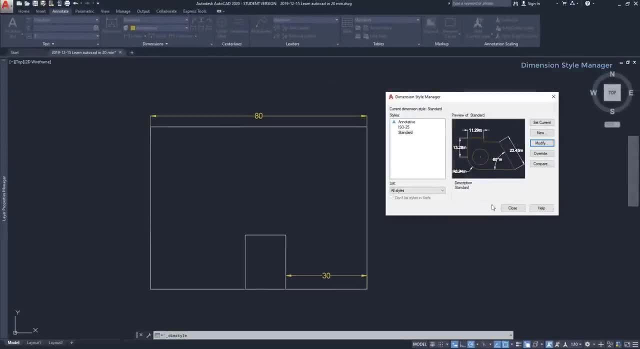 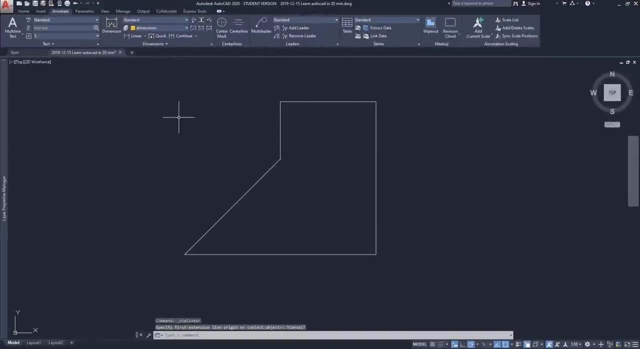 on suffix to appear after the values, like this: other types of dimension lines. as I showed in the beginning, there are more types of dimension lines to use in AutoCAD, depending on what we want to measure. for example, let's measure using the linear dimension, the distance between this point. 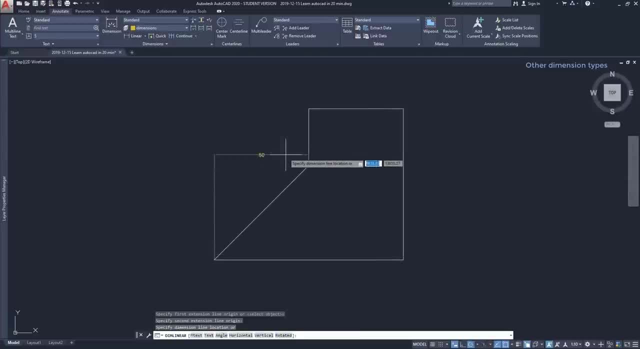 and this one. as you see, it's measuring either the horizontal distance or the vertical one if I move the pointer this way. but this is all fine because I can insert. with this option I can measure objects that are not located in the cortisian axis. so 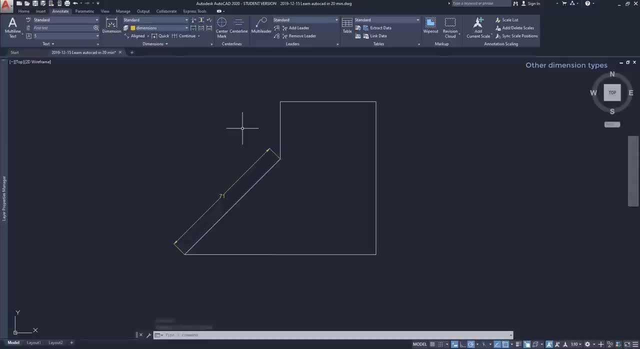 it's much better, as you see. angular dimension. now I am going to click on the angular dimension. this one is still simple to use. I can measure an angle by clicking in two lines that intersect each other. the angle itself I can place in any of the four sides. 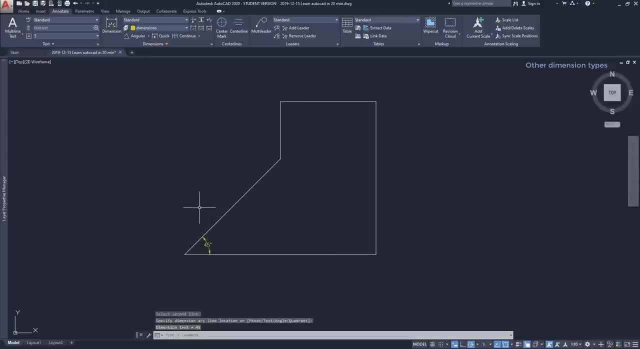 of the intersection plane radius. to measure the radius of a circle, first I am going to draw one here. then I choose the option to measure the radius and just click on the circle. I click again to place the dimension line. in this tutorial I want to show you also. 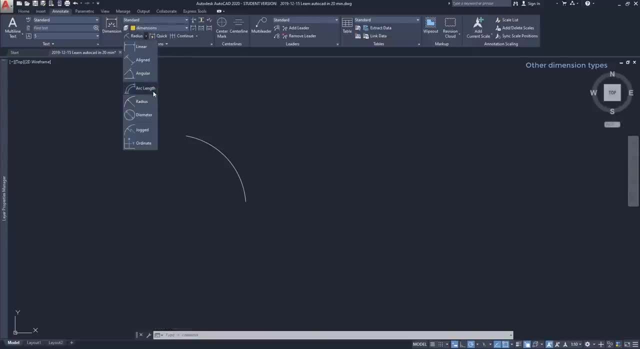 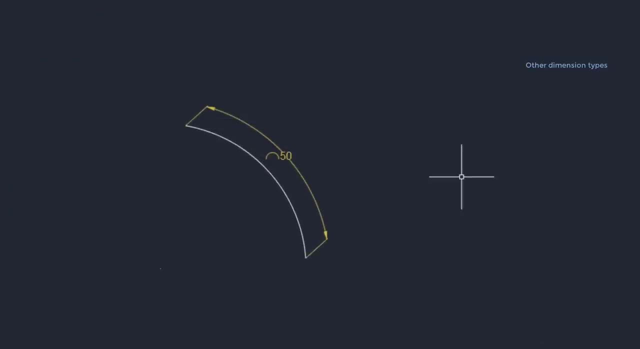 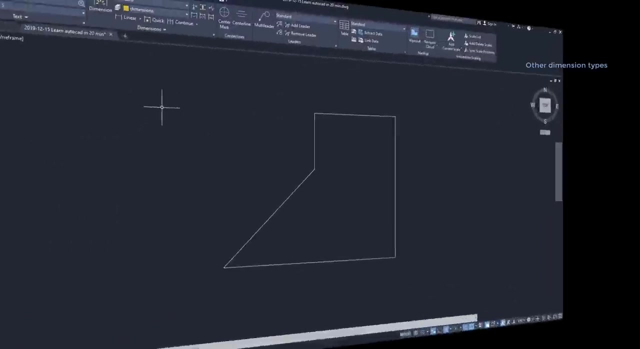 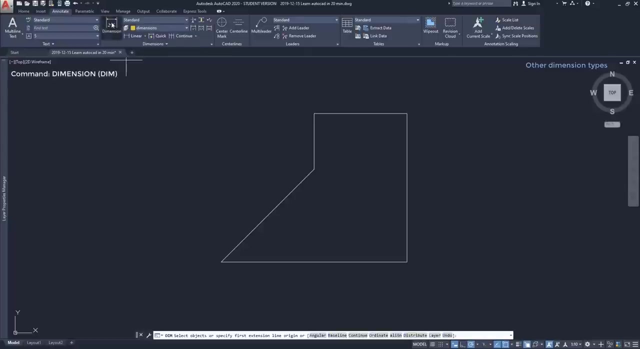 the arc length, I can measure the distance of an arc and, yes, this only works on arcs. if I try to measure the perimeter of a circle, nothing happens. as you see, apart from those tiles, there is the automated dimension, which is the icon. here you can see what is the most suitable type of dimension. 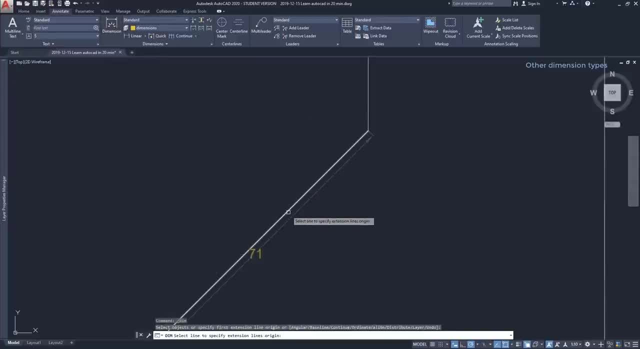 in each situation. for example, if I hope this line, this square, appears and I can click on it and I will place the dimension of the length of this line. I can do the same for the other lines. as you see, for measuring an angle, I have to choose the option angular. 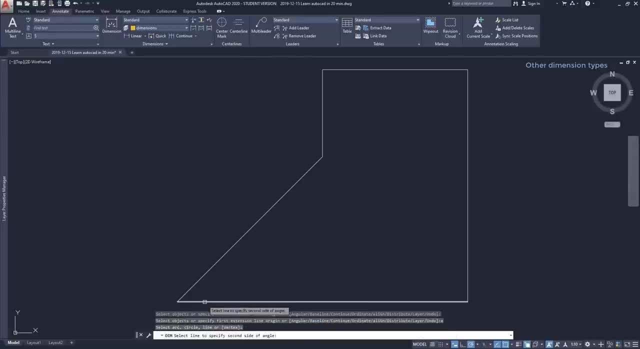 and then I can place it, as I did previously, in a circle. the automated dimension places the diameter by default. however, I can change to place the radius instead. now let's see some tips and peculiarities: dim layer on this tab, at the panel dimensions, I set the layer. 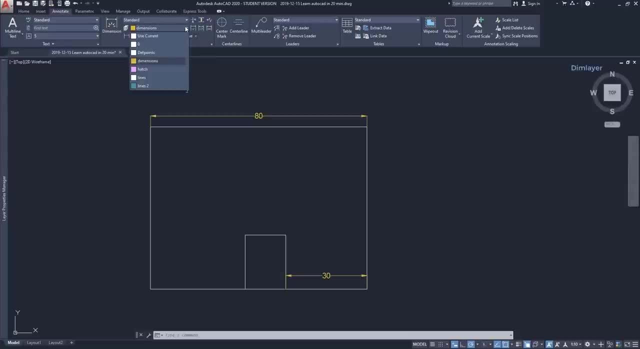 dimension lines in. I choose the layer dimensions as I created it especially for placing the dimension lines. however, if I switch to the home tab, the current layer is lines and if I draw a dimension line, you can see that it goes automatically to the dimension layer. snaps on arrows. 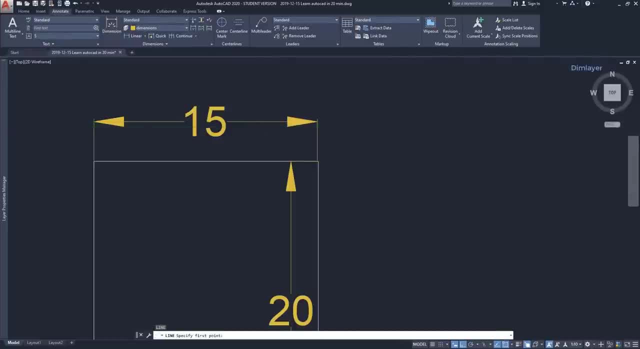 in some versions of AutoCAD I am using the system snaps to the end points, mid points, geometrical centers on the arrow shape, and this is a bit annoying because usually I only want to snap to the end of the dimension line, this point and honestly, I haven't figured out yet. 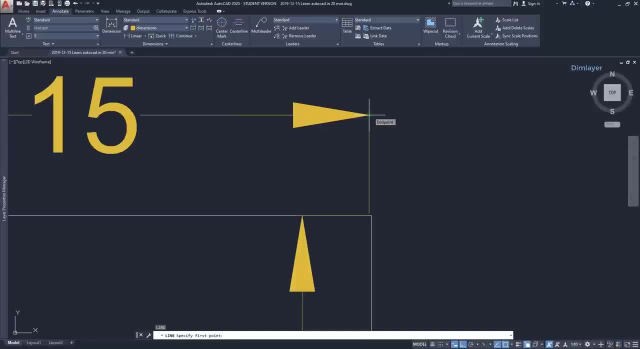 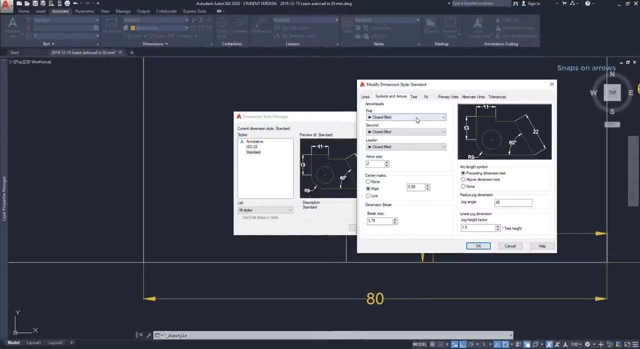 if there is a way to get rid of those snaps. if anyone knows is welcome to post a comment on this video. it would help a lot of people. however, I think this is a good way to deal with this. on symbols and arrows: tab at the dimension style manager. 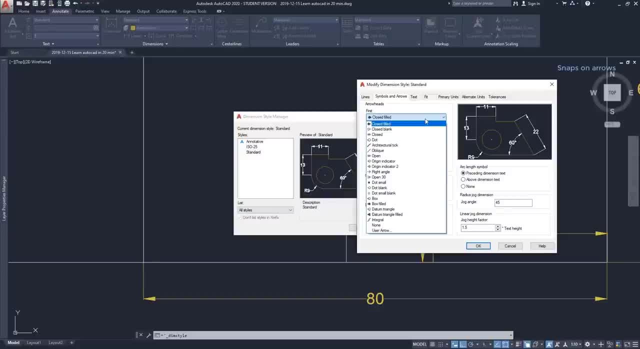 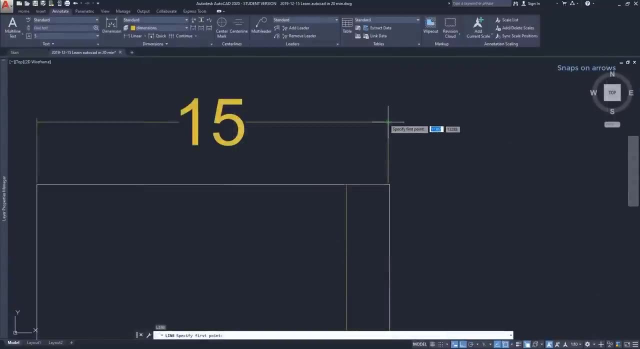 click on the first arrow head and, as you can see on this list, there are plenty of them to use, but for now I choose none. automatically, the second arrow head is updated to match the first one. the result is this: it's easier to snap to the end point.